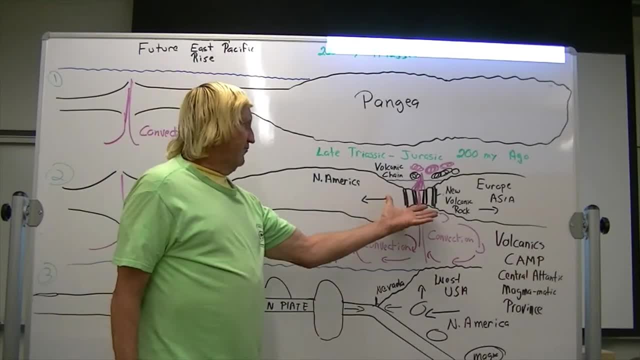 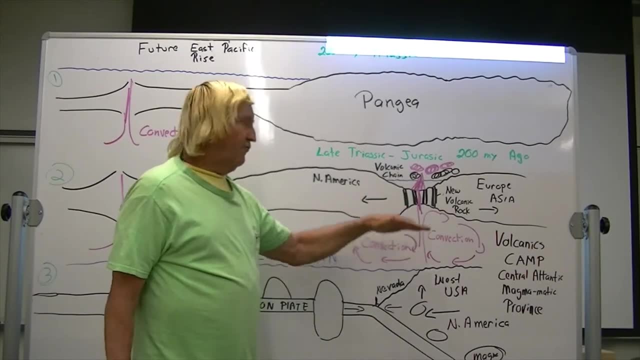 So, as this volcanic activity occurs, it's going to lay down some very mafic basaltic rock. That basaltic rock over time is going to cool, condense, form low depressions and eventually it's going to fill with water. hence the opening up of the Atlantic Ocean. 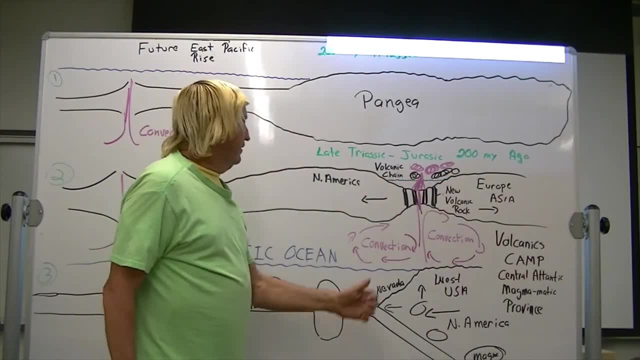 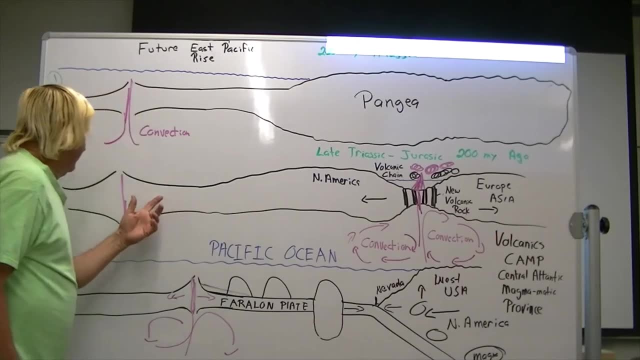 As Europe tends to drift towards the east and North America drifts off to the west, the Atlantic Ocean opens. So what's occurring over here, along the western margin of the North American continent, is that there was a plate called the Fairlawn Plate. 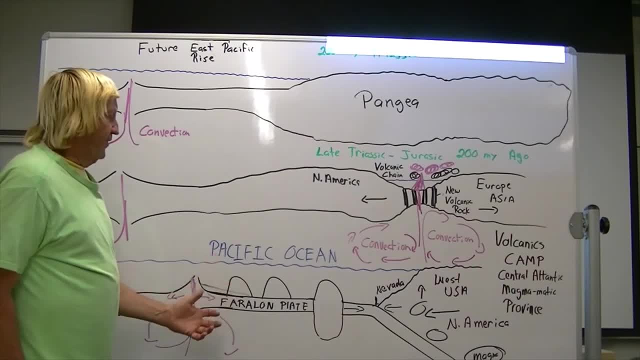 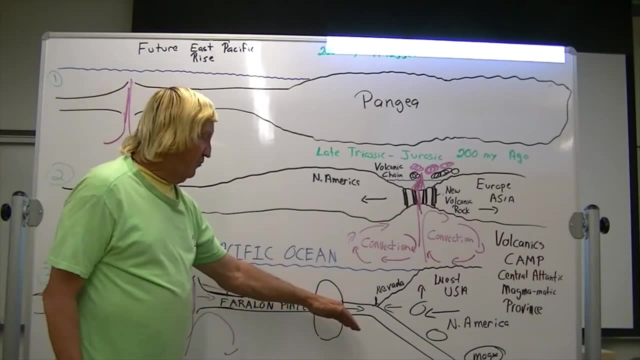 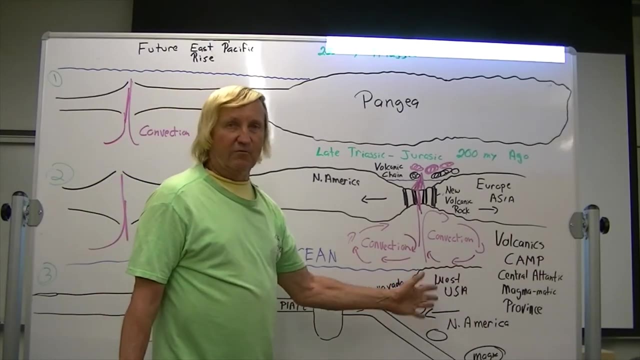 And that Fairlawn Plate now is being acted against by the North American continent, the North American continent moving against it. So the Fairlawn Plate's now beginning to start to move, we think. Certainly the North American continent starts to move west. So at that time there was no California. okay, There was no California. 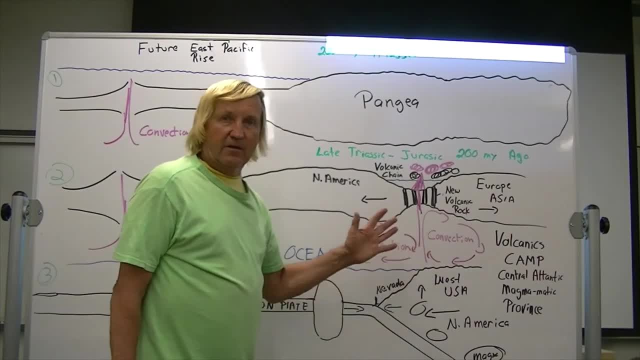 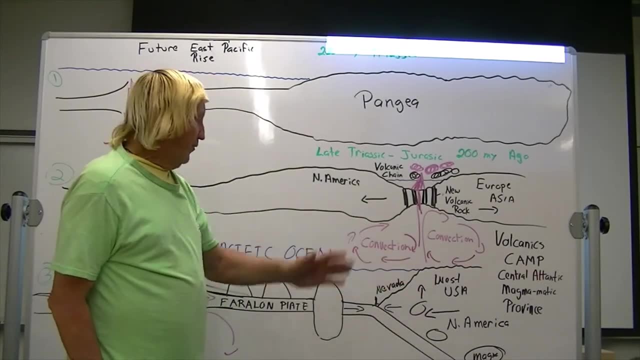 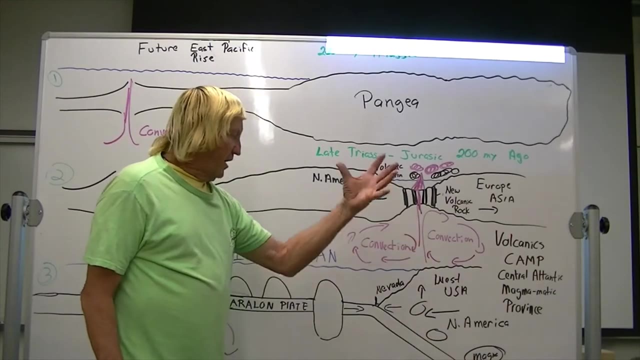 Basically, the edge of the continent during the Jurassic was Nevada, Las Vegas basically. So even eastern Nevada, that was the boundary. So as this Fairlawn Plate subducts, it's going to melt. It's going to then create baffles of magma. Those magma plumes are going to rise. 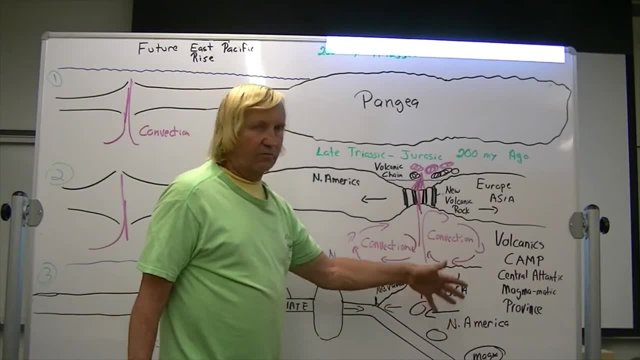 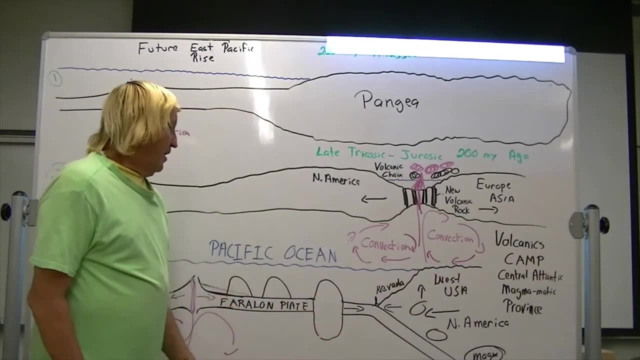 Some of them are eventually going to crystallize and cool underground And then later be uplifted into what we call today the Sierra Nevada Mountains. This little Fairlawn Plate that's coming- actually it wasn't a little plate, it was a pretty good sized plate. 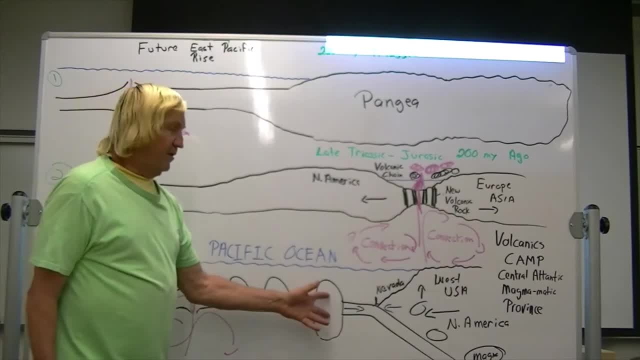 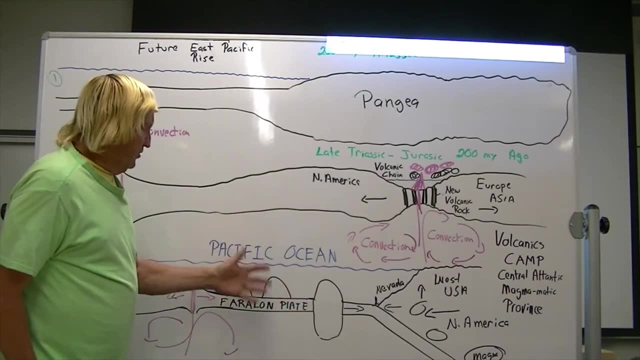 It was kind of a mixed bag. It had some continental material, It had some oceanic plate, basaltic, rich oceanic plates. So there's a combination of things occurring. So what happens over in the western portions of the North American continent? 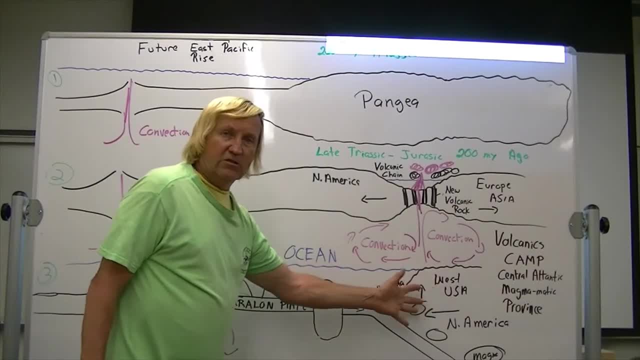 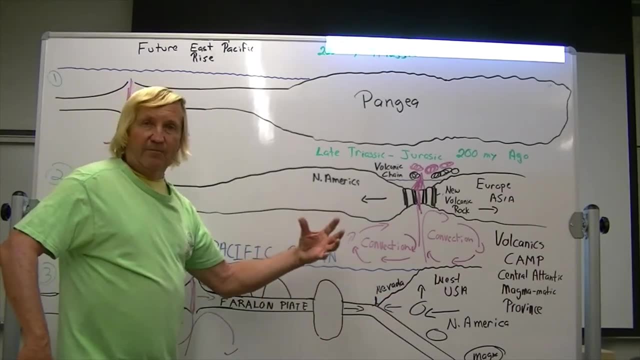 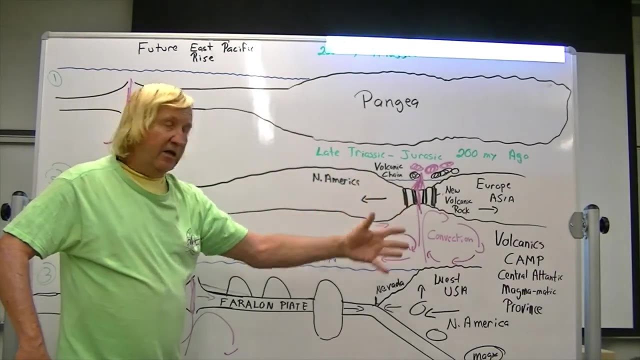 is the continent's going to grow from the east towards the west, because these new terrains are exotic terrains. As Pangaea breaks apart, it breaks up apart into two continents: Laurasia, which is North America and Europe, and basically Asia, And then Gondwanaland, which is South America, Africa, Australia. Antarctica. Then Antarctica and Australia are going to separate, And then that breaks up into a smaller continent called Rodnia. Rodnia part of it was India, which then drifted all the way across the equator to collide with Asia, as it's doing today. 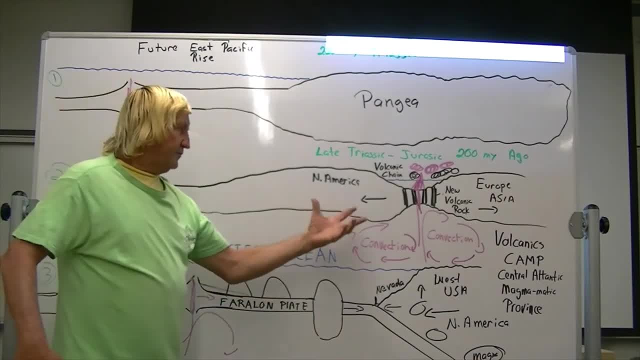 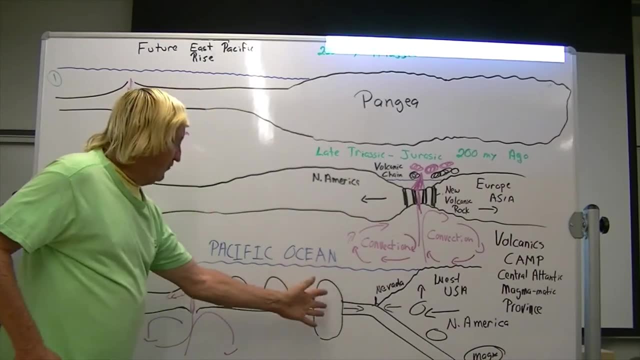 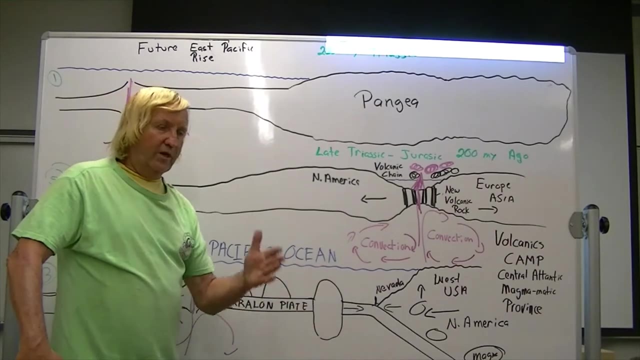 creating the Himalayan mountain ranges, And then Michael Cotton is a Rodnia, so it's not like one continent. It was basically a very fragmented continent and it came over in multiple continents. Up in the Klamath Mountains of Northern California we can identify four different little sutures. 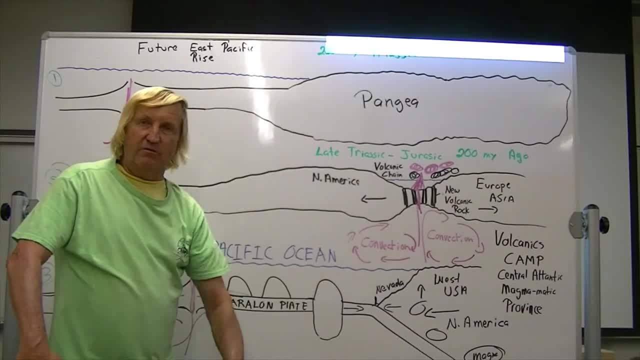 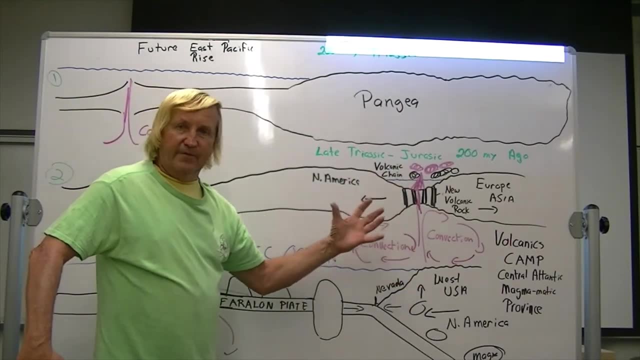 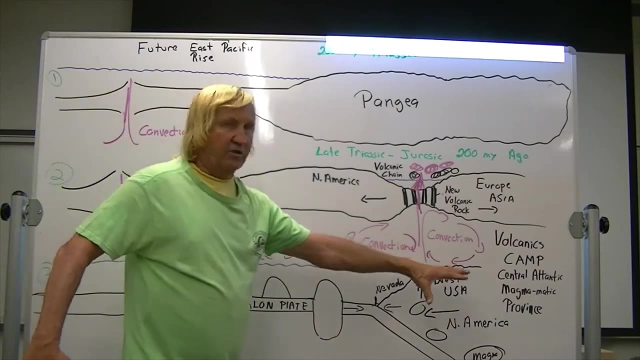 where microcontinents stuck themselves on to the North American continent. So the North American continent, the western portion of Nevada all the way up into Oregon, Washington, California- is basically a collage of all these microcontinents. So what happens with North America is we have a mountain range on the eastern seaboard, the Appalachians. 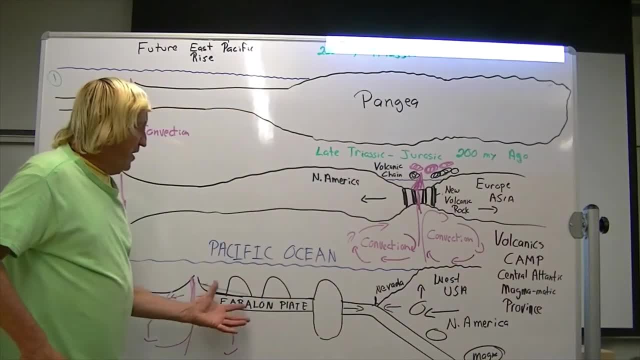 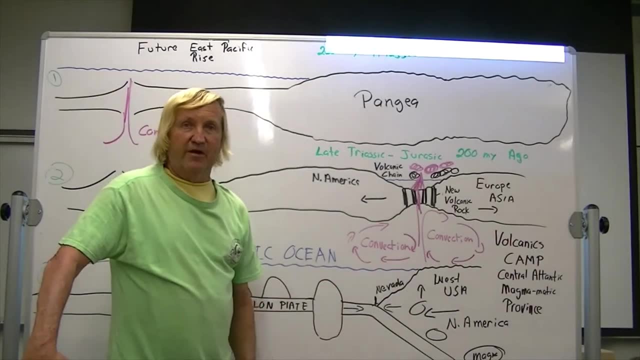 which is an old mountain range at this time, by that time, And we now start to see uplifting western mountains, the ancestral to the Sierra Nevada mountains, And they're really going to start uplifting about 65 million years ago through the Cenozoic. 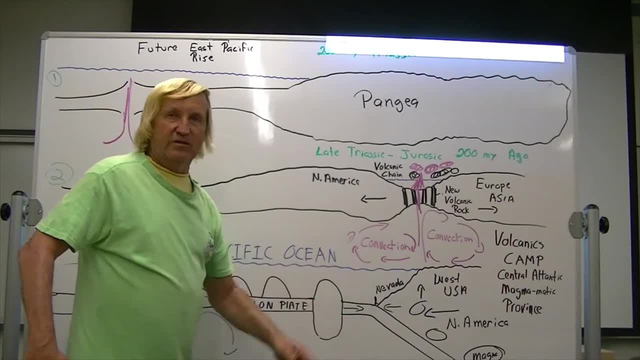 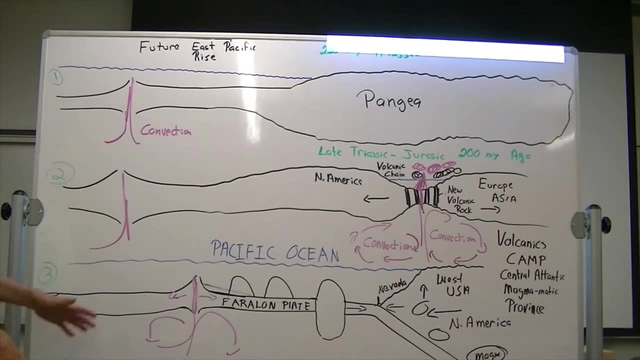 So our goal today is to kind of wrap up the Mesozoic and then get through the Cenozoic, And so I just thought I would show you this nice little illustration I drew to kind of show the sequence of events. Where are we today? 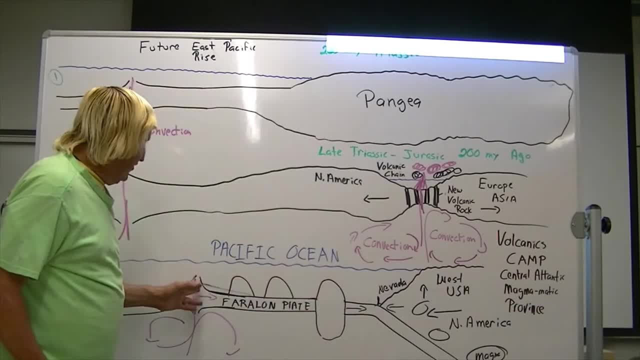 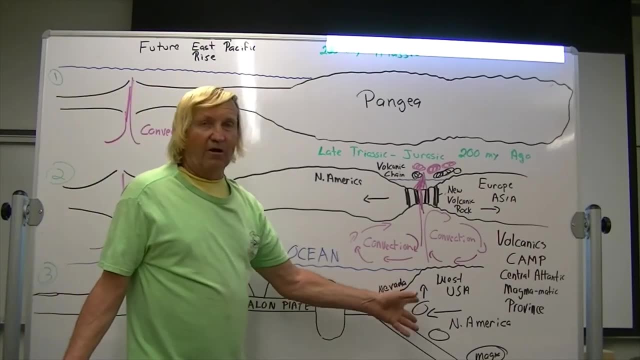 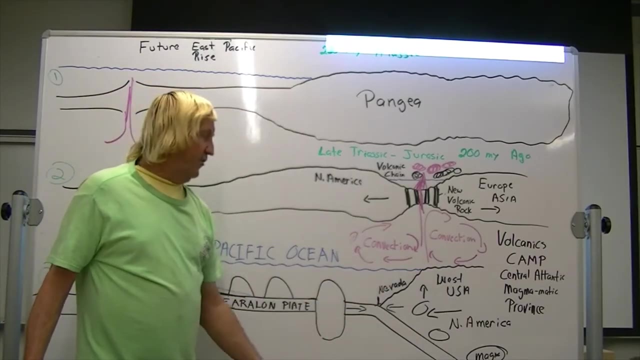 Well, the North American continent moved so far to the west that it overrode this spreading center. This spreading center is now in a good part of the North American continent and that spreading center is the San Andreas Fault. So the San Andreas Fault is the plate boundary between the Pacific plate and the North American plate. 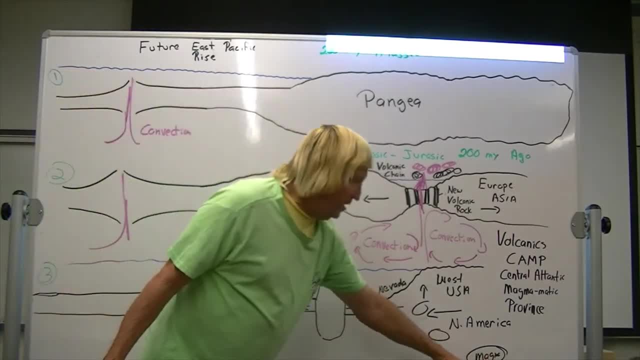 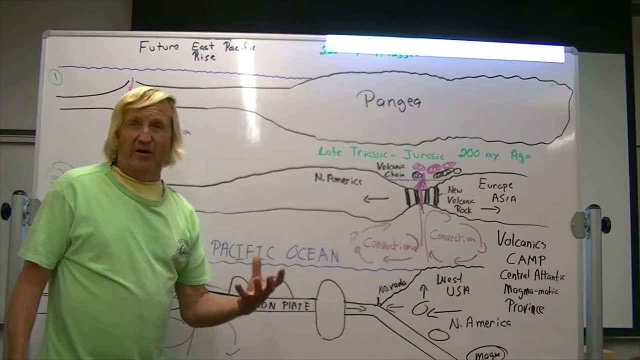 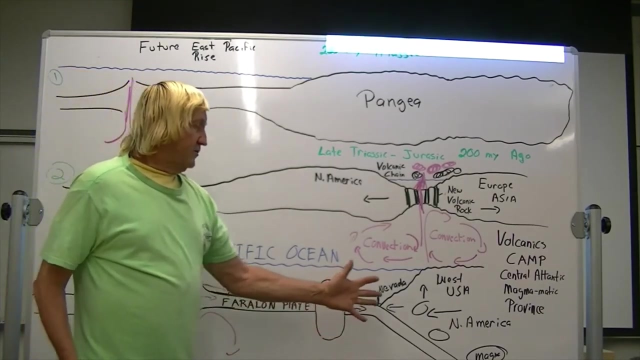 So the Farallon Plate? it's gone, It's subducted. What's underneath? it's melted. Some geologists believe that what's left of the Farallon Plate is kind of under Nevada in Arizona right now. And so the North American continent has continued to move to the west. 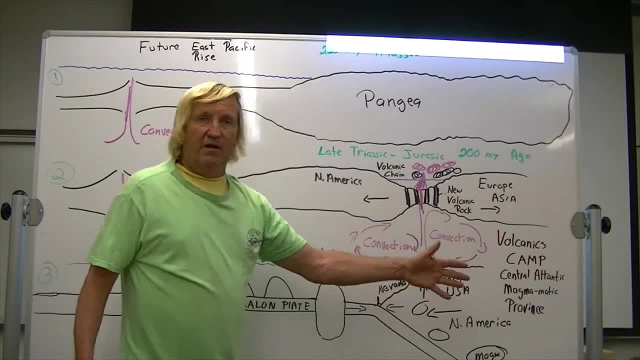 And as it does, that's creating the San Andreas Fault to migrate towards the east. So right now the San Andreas Fault really wants to jump. It can't because it's locked between the Pacific and the North American plate. It can't because it's locked between the Pacific and the North American plate. 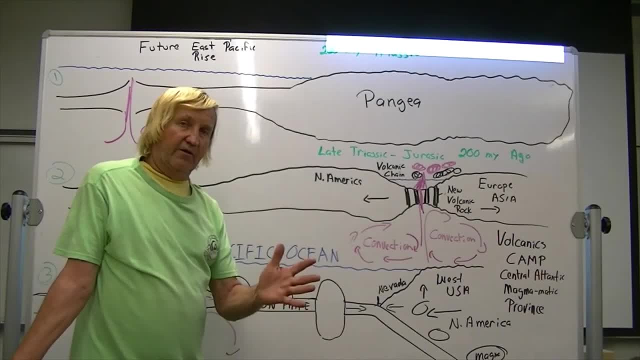 It can't because it's locked between the Pacific and the North American plate, The San Bernardino and the San Jacinto Mountains. it's kind of locked there. It wants to go to the east. It wants to actually connect with the Calico Fault near Barstow. 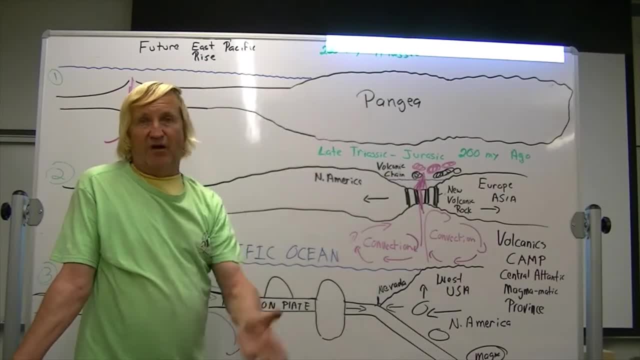 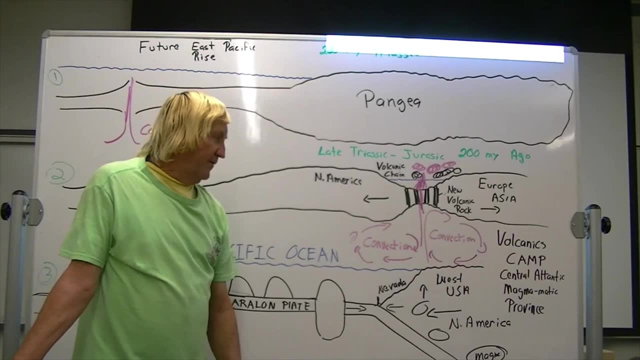 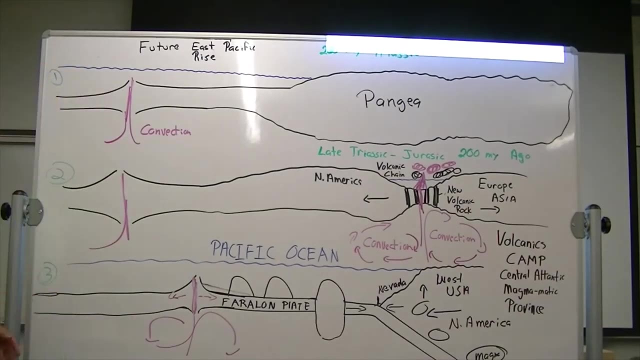 Eventually that is then going to move a little more to the east and connect with the Death Valley Sequence of Faults And then eventually with the Walker Lane, which is in Nevada and California, And so this is kind of a general history of what tectonically has been going on. 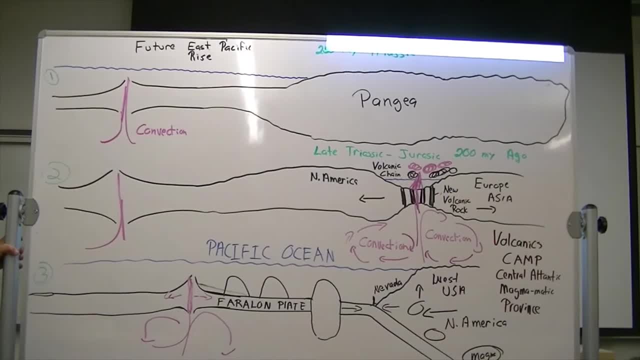 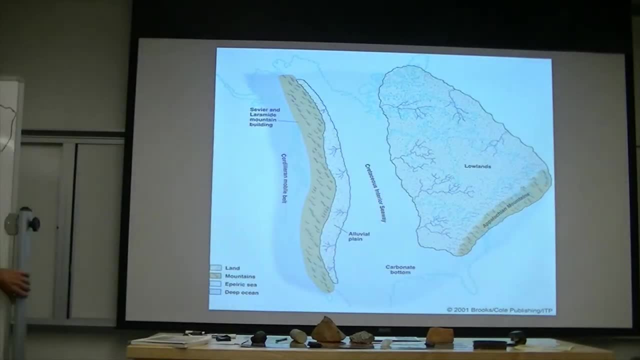 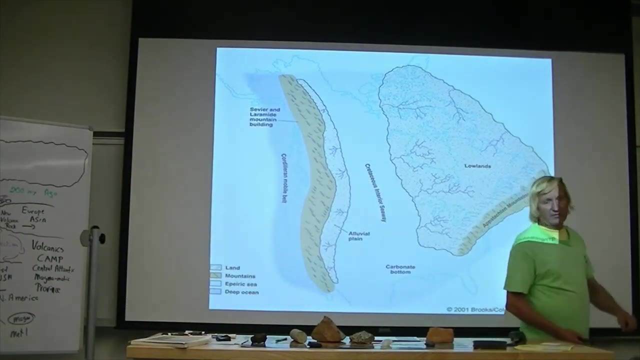 So now we will continue. so the Cenozoic starts a new era. before we get to the Cenozoic, we have to kind of wrap up the Mesozoic, The most important thing about the Mesozoic occurring in the mid part of the continent. 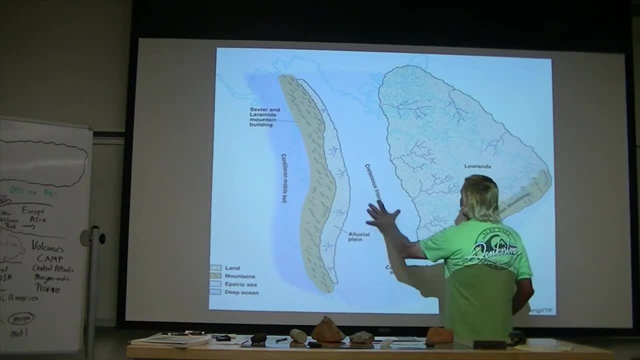 was basically this wonderful little Sundance Sea, And the Sundance Sea is going to disappear because it's going to get filled in. It starts to get filled in because, as Pangea breaks apart, over in the western United States, we're meeting this Farallon Plate and all these little microcontinents. 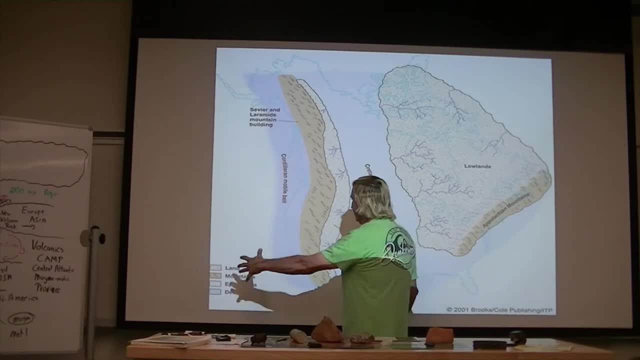 We've got subduction going on, we have accretion of exotic pieces of Rhodnea being stuck onto the North American continent And that causes the North American continent on the western edge to uplift. so we have a mountain range in the west, a mountain range in the east. 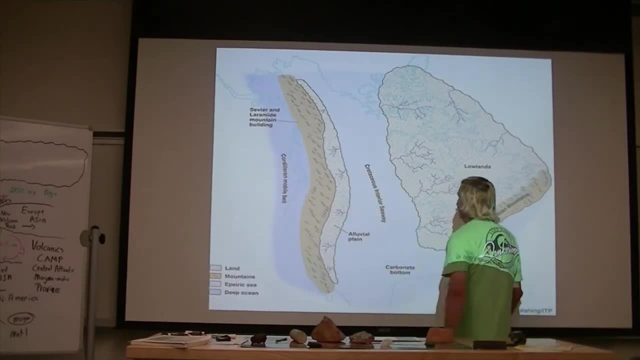 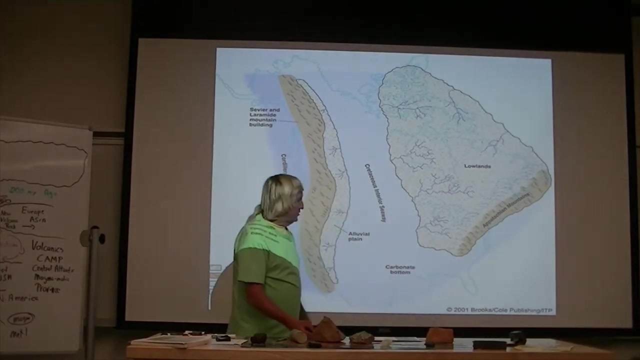 That's generating sediments. that's eventually going to fill this interior seaway into the Sundance Sea. And one of the most important things about the Mesozoic, throughout the Jurassic and the Cretaceous, is it really evaporates So a lot of salt gypsum. those minerals are formed during the Mesozoic. Why? Because the North American continent is at the equator. still It's pretty close, pretty equatorial, And that is the perfect environment to get these small little pockets of seas where salt water can intrude and then not have any influence from the rest of the oceans. 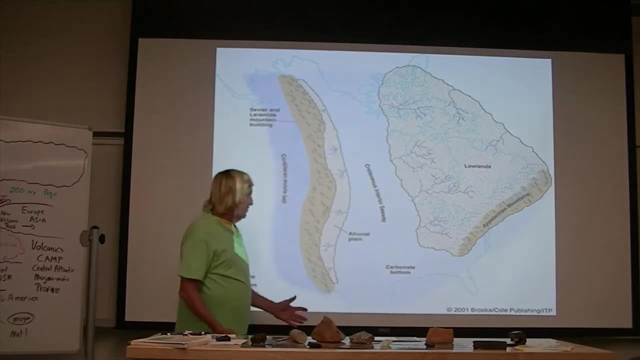 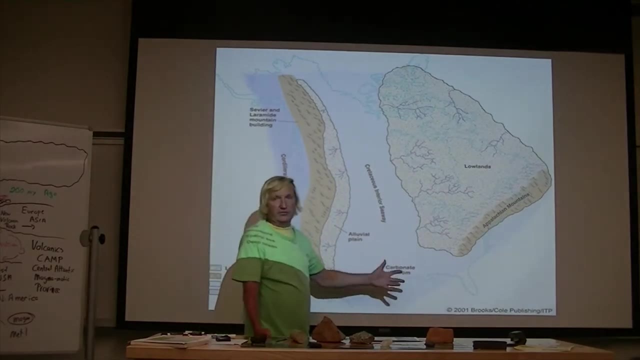 and then those water deposits will evaporate and they seem to get flooded again periodically, get flooded and the water was evaporating and over time it resulted in huge accumulations of salt and gypsum And they're very important resources today, especially gypsum. It's used for a lot of things: for wall boards and construction. 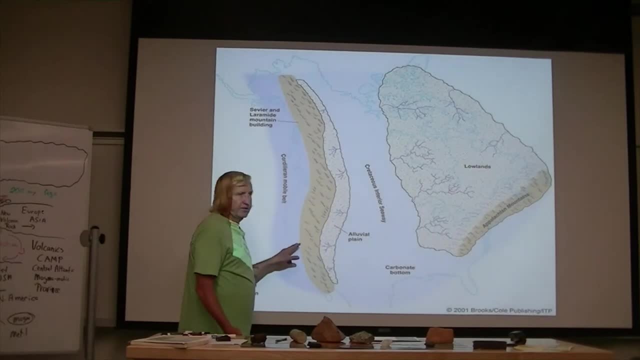 Interestingly, there is a gypsum deposit off the 91 freeway called Gypsum Canyon Road, And that was probably one of these small little seaways where water got trapped in. There's some great ones in Utah where, as the Sundance Sea, retreated, 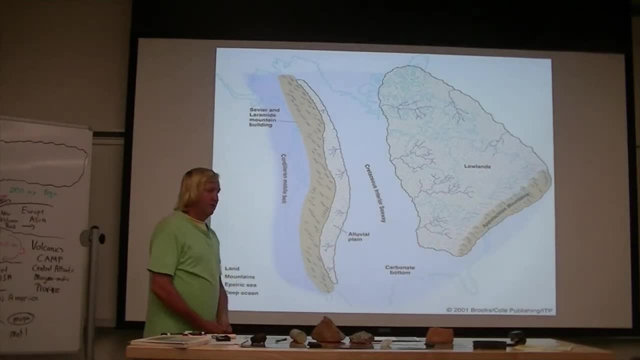 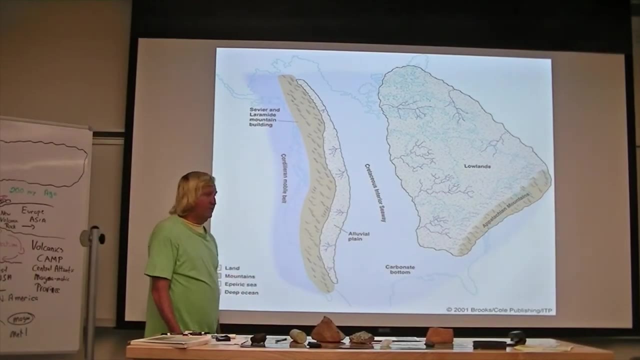 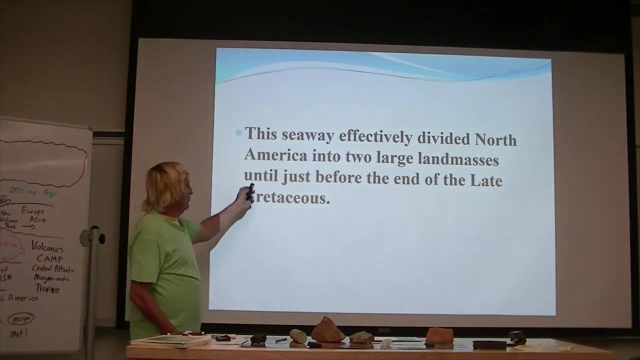 little pockets were left behind and gypsum was deposited. So the most important thing about you know, from a mineral perspective of the late Mesozoic, mid to late Mesozoic, was basically evaporates, salt and gypsum. So eventually this seaway is going to divide North America into two land masses. 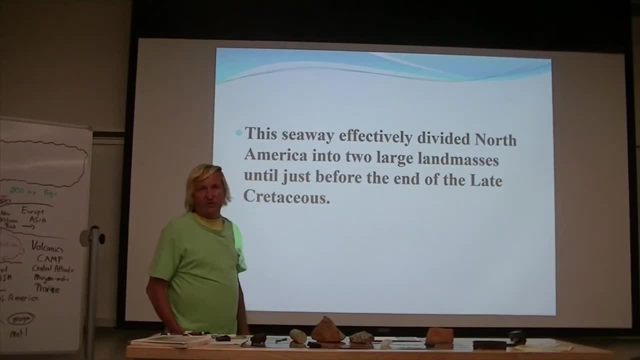 Those land masses are going to shed off sediment, throw off the Cretaceous, fill it in and then, as the Panjshir breaks apart, now we now have subduction going on along the western margin of the North American continent and that is going to result in the growth. 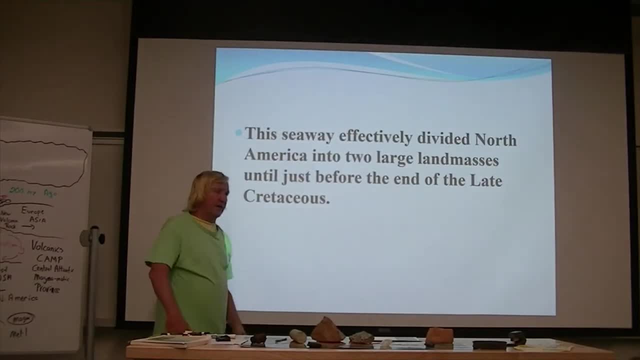 of the western United States. So everything basically, that is British Columbia, Oregon, Washington, all of California, parts of Nevada. that is all what we call a created terrain. This is geology that came from someplace else. Australia- And Catalina Island, is a really good example of that. 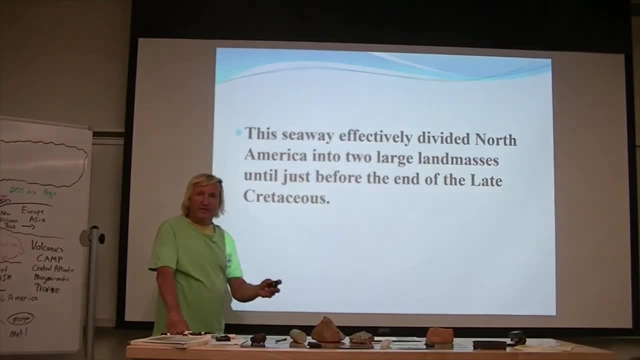 Catalina Island is definitive proof that California is part of the Australian continent. So in Catalina Island, the rocks there don't match any of the other channel islands. There's blue schist and green schist. Those rocks were once sedimentary sequences of rocks. 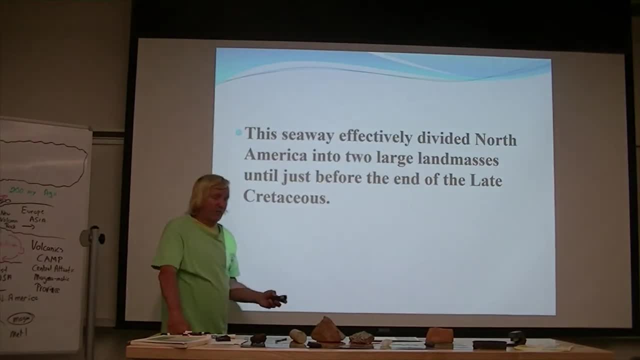 We even have amphibolites, And what this suggests is that this microcontinent that broke off from the land mass of Rodnia tried to subduct, but it could not subduct. It did have some partial melting, to the point where it formed metamorphic rocks. 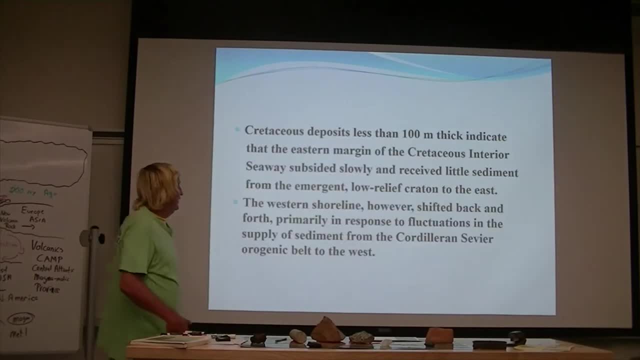 and then I think it popped back up again. So, Cretaceous deposits: we have this huge accumulation And this indicates that this low relief eastern part of the United States shed very little material into the sea. But as the western United States starts to uplift, 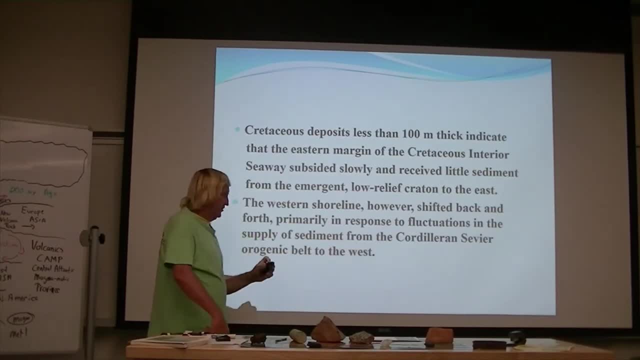 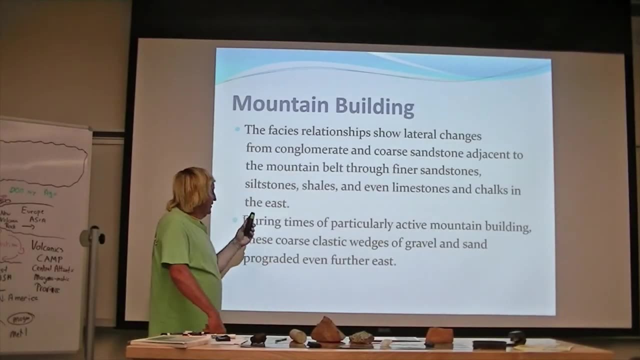 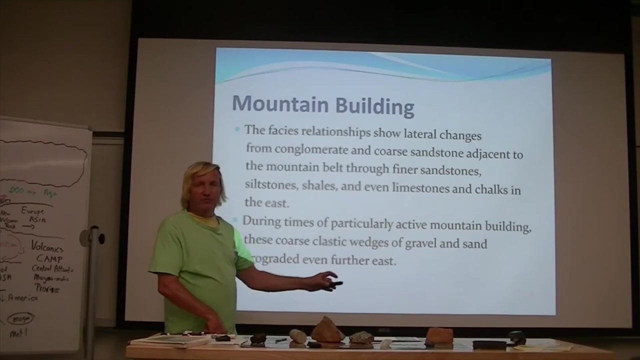 that's going to fill in the Sundance Sea And the Sundance Sea is going to go bye bye, And so we have mountain buildings. At this point the western United States goes from a passive margin. very broad continental shelf, great for aquatic fauna. 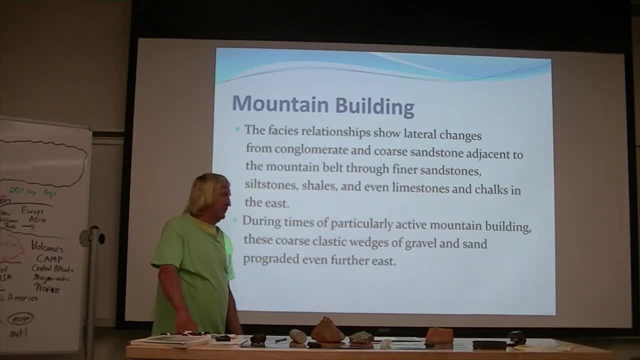 very exotic organisms live off of this shelf, And creatures that live in oceans that are filter feeders do not like water that has a lot of sediment in it. So, as a result, the biology of the western United States changed because of geology. 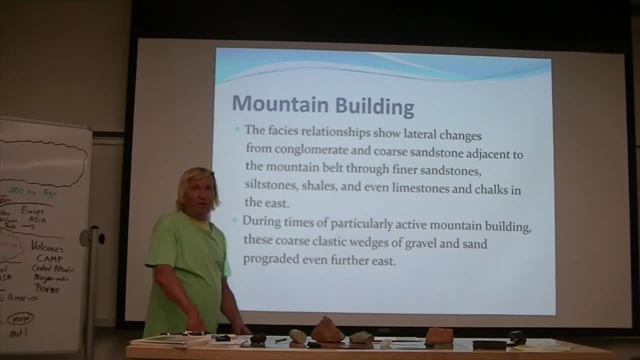 So geology has a very strong influence on the biological setting, on what plants and animals are going to live there, And so coral reefs and things like that they're going to go bye bye, because what's going to happen at this point in venture of the North American continent? 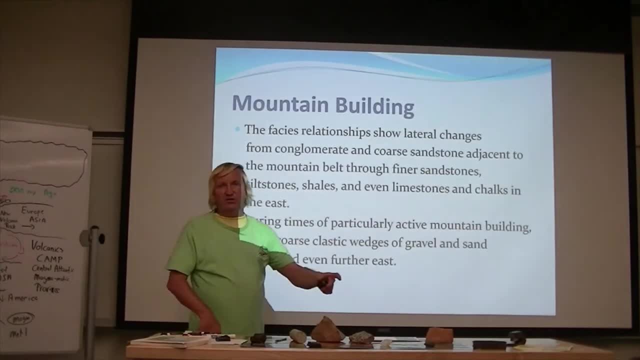 as mountains start to uplift, a lot of sediment is going to be shed off. So on the Santa Ana field trip up into the Tucker Wildlife Reserve, we have these very rounded conglomerates, red ones, which are indicative of shallow marine water with sufficient oxygen. 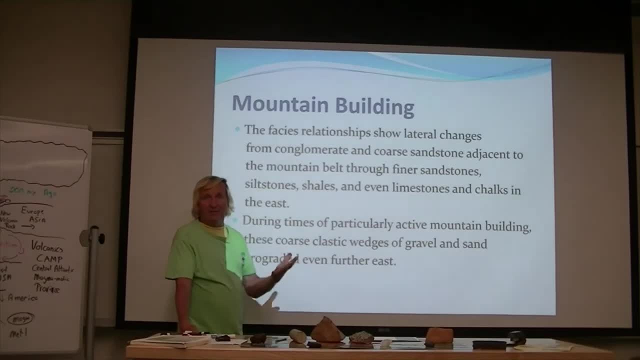 So, with sufficient oxygen, the iron oxidized into hematite iron oxide, which is red in color. Those green sediments indicates that that was a deeper water environment. So there's a lot of tectonic activity going on in the western United States. 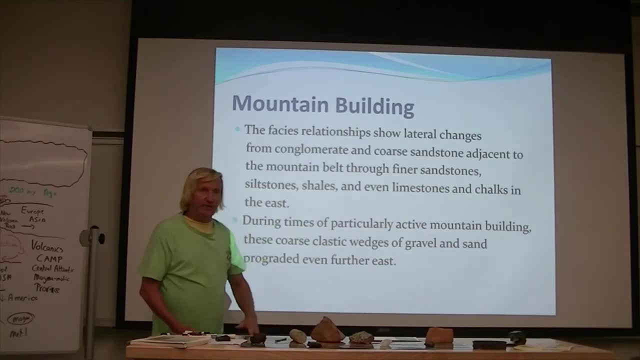 Rocks are being pushed up. In other areas rocks are being shoved down And that green color sediment is suggestive that that was deeper water, That was water that was void of oxygen, And I think that you could build a case for that because of the presence. 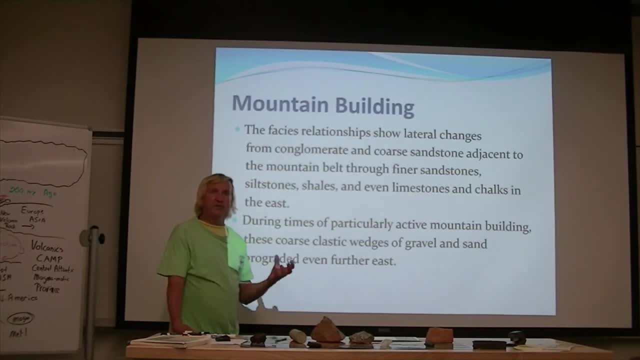 of the jasper and the flint, the sedimentary quartz. Those quartz minerals grow and very what we call pelagic waters, waters that are void of oxygen, And that's the right environment for that. So the green color plus the presence of those minerals. 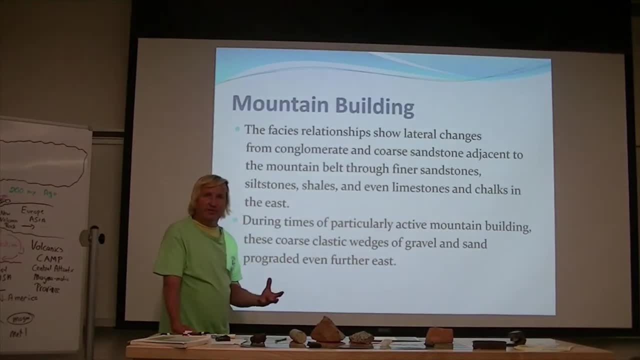 the sedimentary versus the quartz, the jasper, the chert and the flint suggest that those sediments on that Santa Ana field trip were deep, deep water Off the coast. so this is sediments being shed into deep canyons. 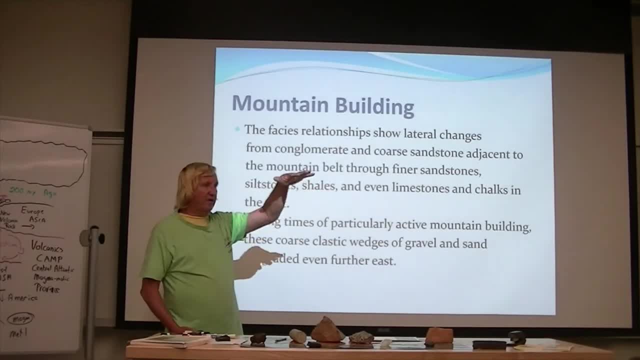 so mountains are uplifting so rapidly that they're creating a coastline that is very steep. So instead of a continental shelf, like you see in the Asian Sea or the United States, you have very deep drop-offs, submarine canyons, and that's where those sediments 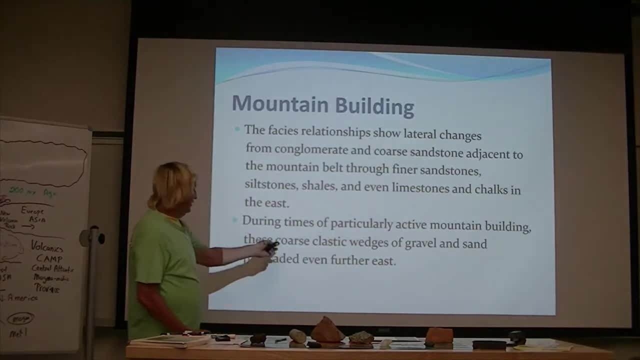 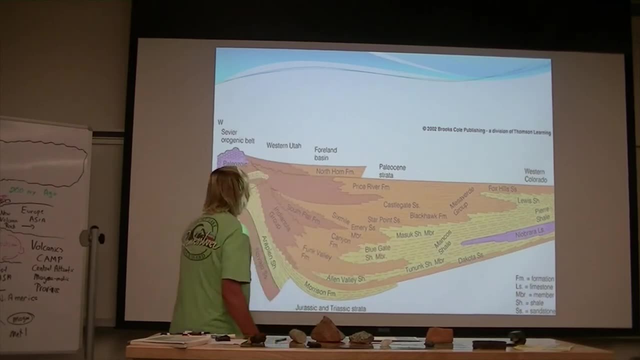 in the Santa Ana Mountains were formed in that different environment. There's gravel wedges, So sediments tend to accumulate and as they accumulate they're going to fold down into sinclines. A good example of a sincline is the entire San Joaquin Valley. of California, So from Bakersfield all the way up to Sacramento, there's this huge accumulation of gravel, because on the east side you have the Sierra Nevada Mountains, On the west side you have the coastal ranges and so the San Joaquin Valley. 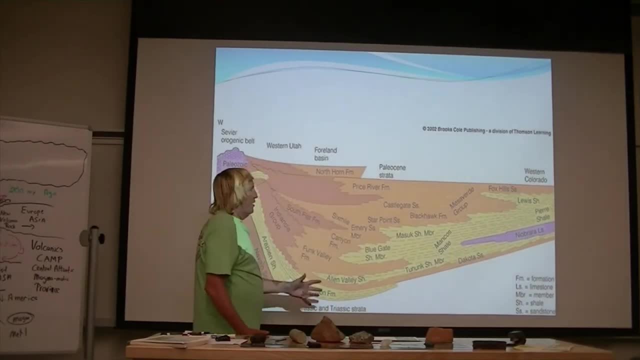 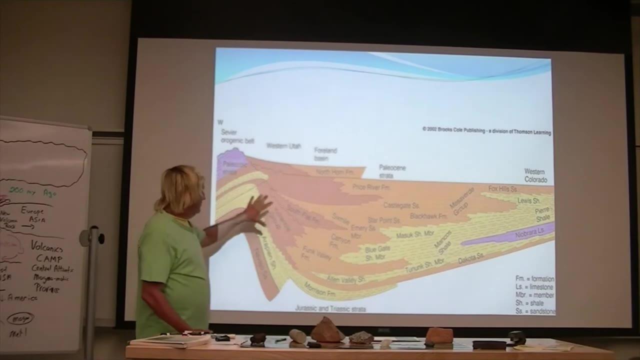 is going to be sandwiched in and these sediments are down-dropping, and we see this throughout the mid part of the United States. We see this in Utah. This is a repeated sequence and sometimes these formations are very important because they can accumulate hydrocarbons. 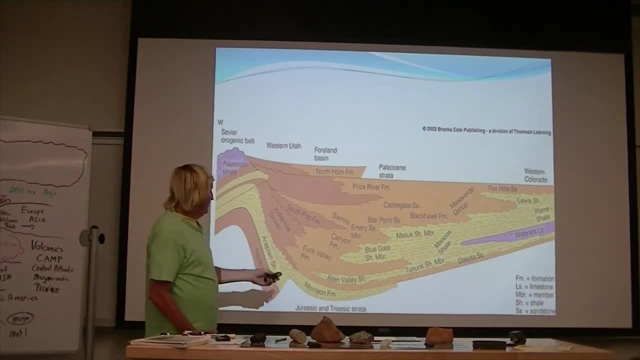 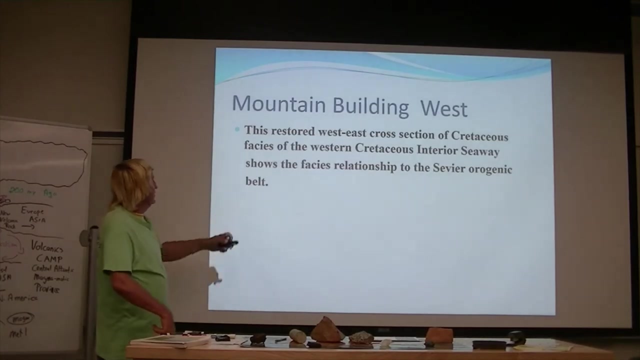 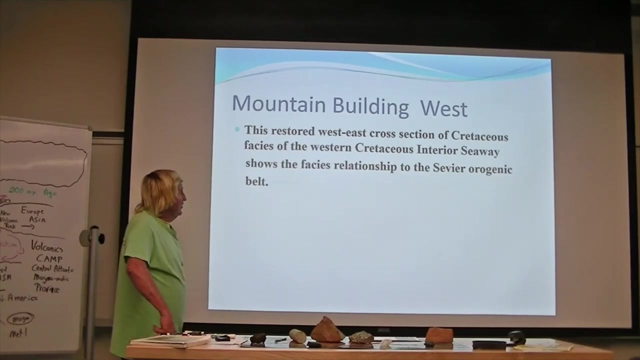 and you can actually see deposition of organic rich material, resulting in oil shales and coal deposits and even good strong oil. So a mountain building in the west, So the Cretaceous interior seaway slowly goes away And as the Mississippi River ended, 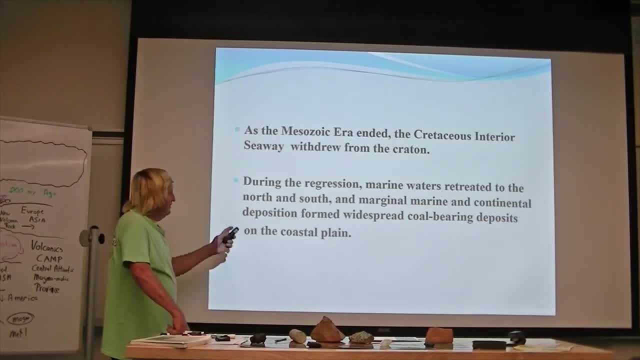 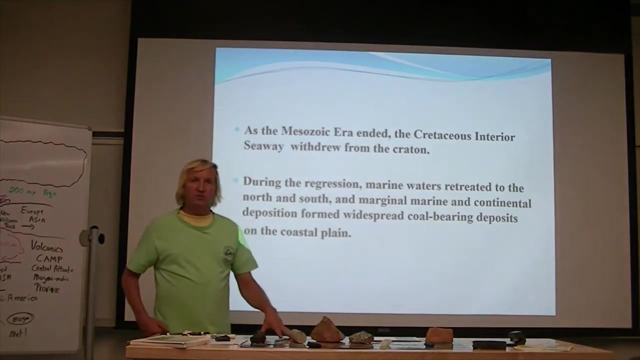 this Cretaceous interior Sundance Sea is going to leave, And this is actually in a very warm environment. So in order to have deposits like coal, you have to have an environmental condition where you have lots of organic material, So there had to have been lots of biological activity occurring and generally around equatorial levels, generally around equatorial plains and equatorial regions. you have sufficient energy and sunlight, photosynthesis and a huge buildup of biomass, And then those biomass, that carbon can migrate and accumulate in a sedentary trap. 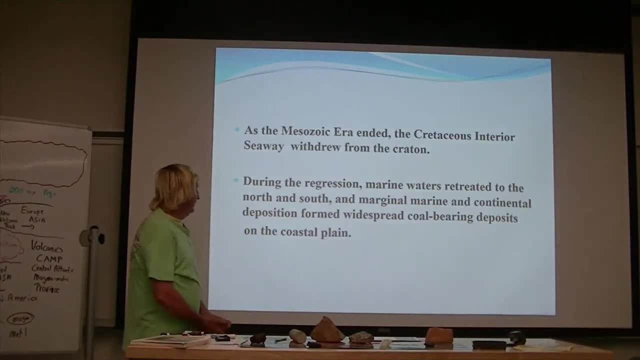 such as an anticline or a syncline, And this is why we find coal deposits in places like Utah. We find oil shales and oil in California. So these organic rich material were formed during the Cretaceous time, when the Earth 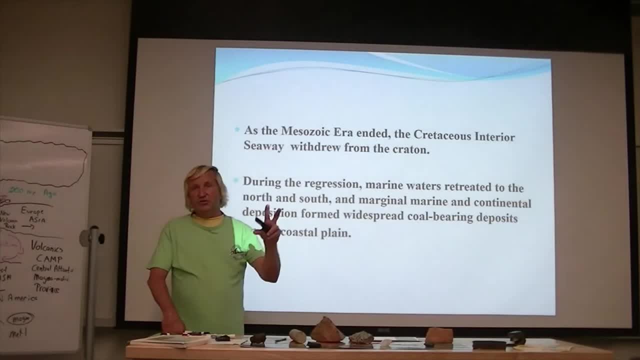 not so much the Earth but the North American continent was in a position to be further south than it is, and it warmed So during the Cretaceous. though continents are spreading apart, Continents are now beginning to move into more southern I should say up north and down south latitudes. So as Pangea breaks apart, that supercontinent that wants to occupy the equatorial plain, is changing And now you're seeing a little more diversification with respect to latitude. And so as you go north, 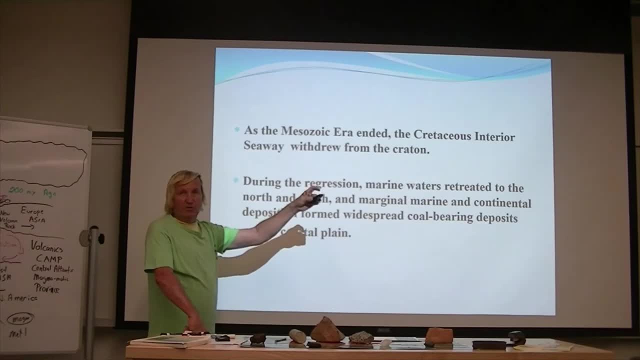 extreme north away from the equator, or extreme south away from the equator, your temperatures are going to change dramatically, and so continents actually start to see more and more of the same things. And so you know, continents actually start to see. 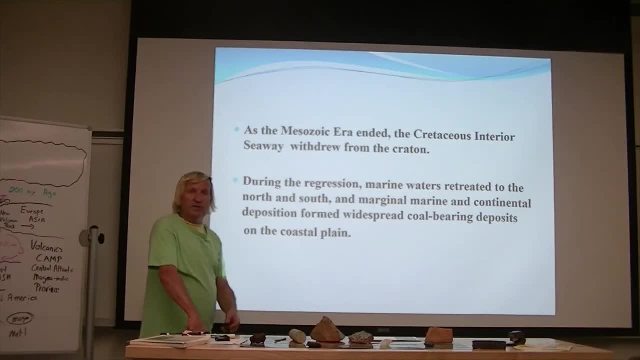 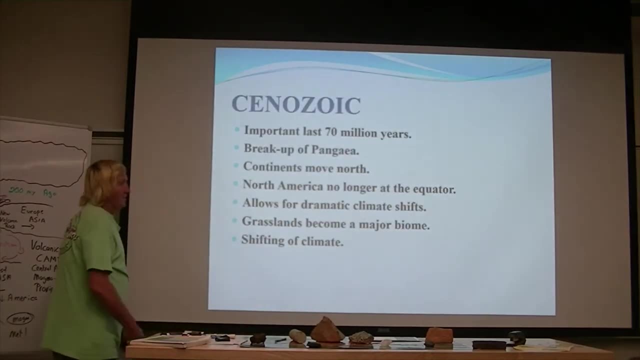 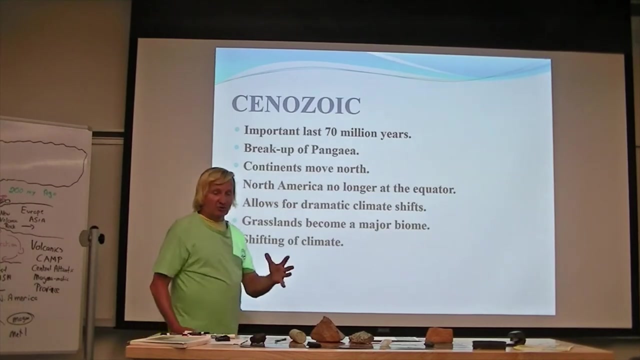 for the first time, very diverse ecosystems, all based on latitude. So the Cenozoic is probably the most important aspect of the last 71 years. If I were to ask you a test question- and I will- I'll write the pencil here. 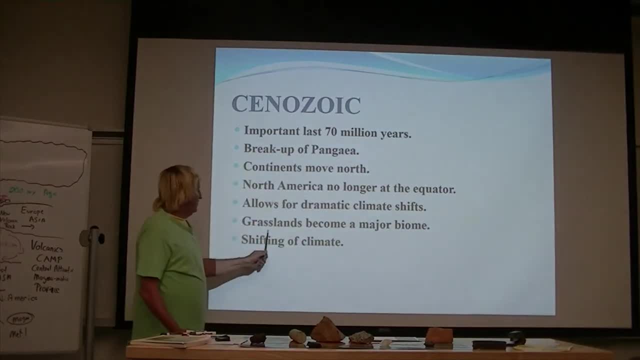 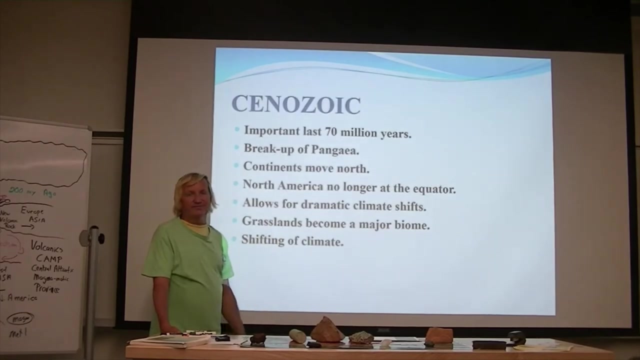 so I can write that down right. grasslands are probably the most important ecological biome to form during the Cenozoic. Now people mistakenly say that the Cenozoic was the age of mammals. Yeah, maybe The early part of the Cenozoic. 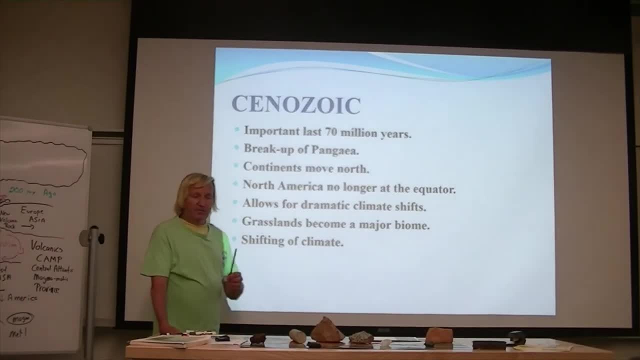 was really the age of birds, Because the direct descendants of the dinosaur die-off were birds, And birds just spread out Many, many species of birds, And that's primarily because at the end of the Mesozoic and the beginning of the Cenozoic, 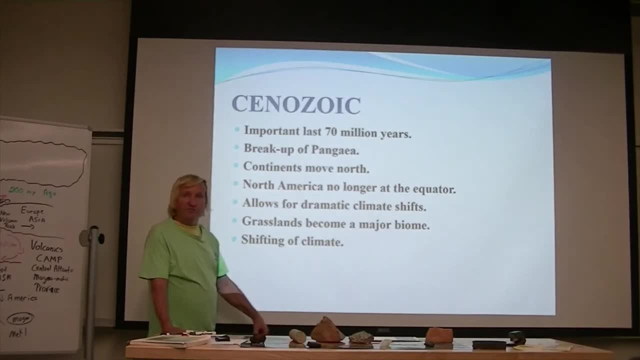 there was this huge void and birds filled it. The animals, the mammals, what we think of as large grazing mammals, aren't going to come along until the grasslands become developed, Because once the grasslands come in place, this is where the grazers 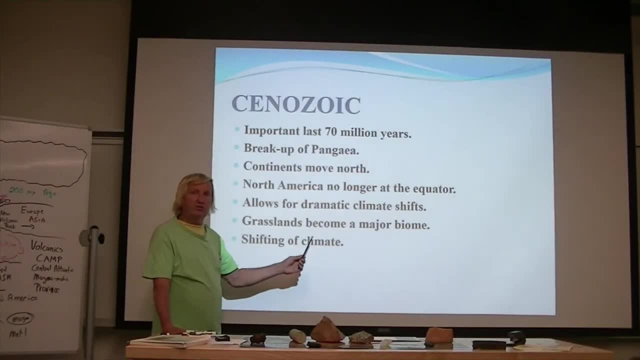 the elephants, the zebras, those sorts of animals are going to graze upon grasslands, And then what's going to follow them are going to be the cats and the dogs, the wolves, the coyotes, the lions that are going to prey on. 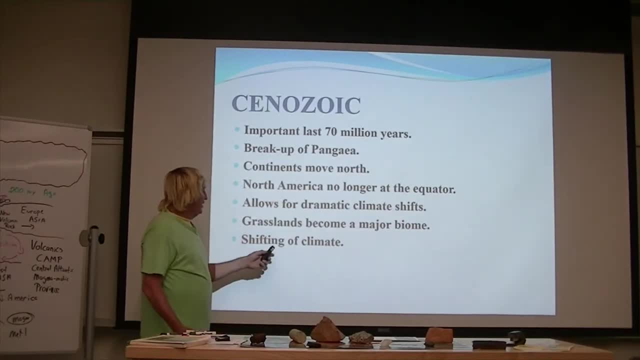 the grass eaters And the grasslands become a major biome because of shifting climate. Because now climate becomes more diverse, You start not to have like when they had Pangea. we had basically two biomes. we had rainforest and desert. 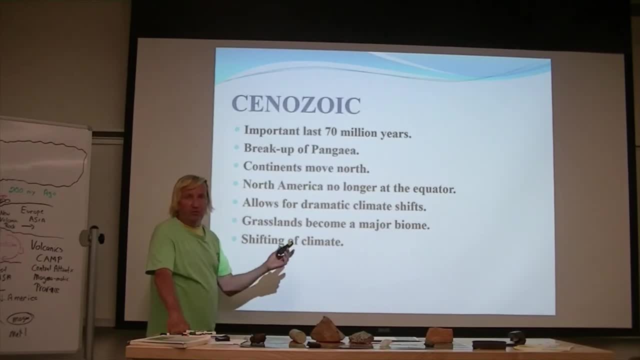 Both warm. Now we see deserts that are cool. We get to see tundras, we get to see savannas, grasslands. Climate becomes very diverse in the Cenozoic And the one species that is the most prominent. 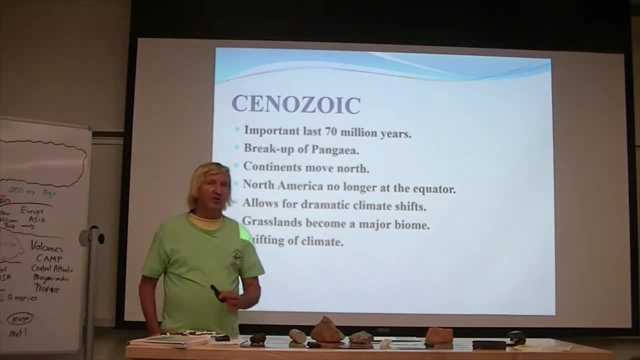 of all the species on Earth that take advantage of this diverse climatic conditions and these diverse ecosystems, are the angiosperms, the flowering plants. They become the most prominent. So think about it: today You can see flowering plants in the tropics. 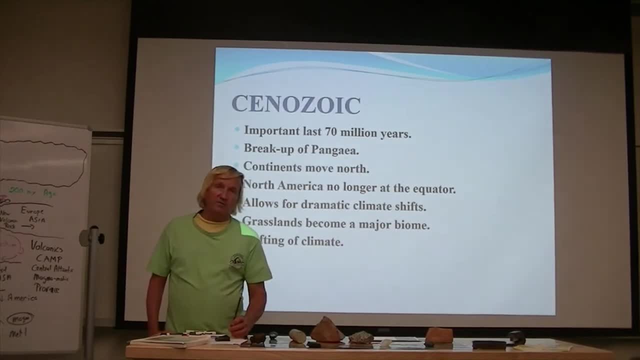 You find them in deserts, You find them in cold climates, You find them up in mountains and valleys and everywhere in between along the coast. So angiosperms flowering plants become the most prominent species. In fact, if you were to draw a graph, 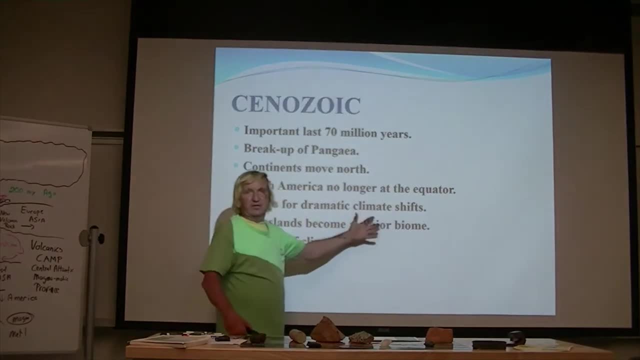 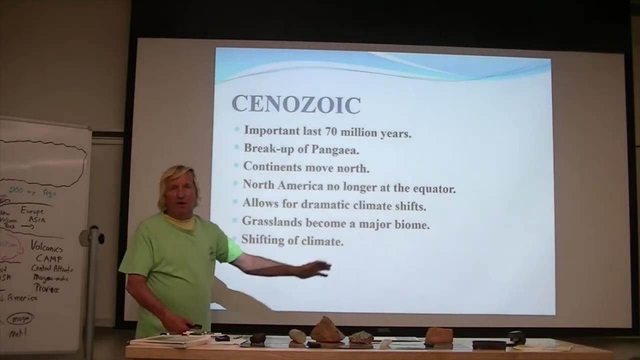 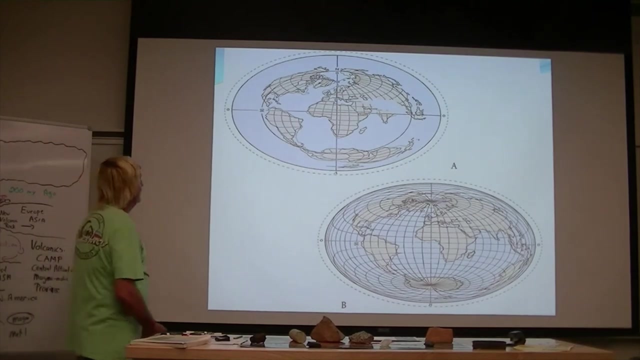 showing the distribution of, say, birds, mammals, humans, orangutans, monkeys, whatever the angiosperms by far number, all of those combined. So it's amazing that they are the most important. So what happens is: here's the equator today. 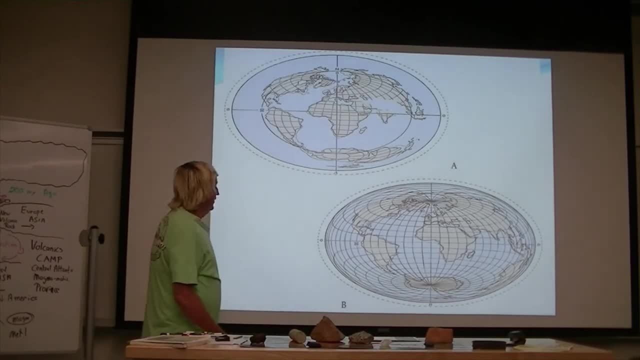 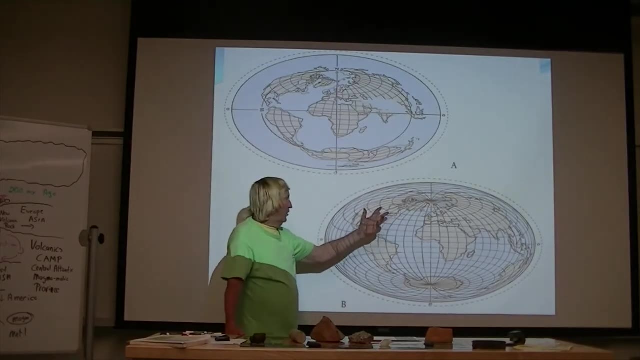 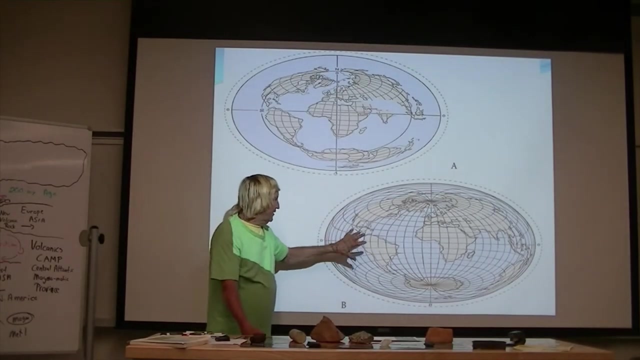 And so the continents start to drift away from the equator. More northern, I mean Canada. The Berger Shell is a good example of that. So the Berger Shell was formed when the Canadian continent was part of Pangea down here. Actually it was really pre-Pangea. 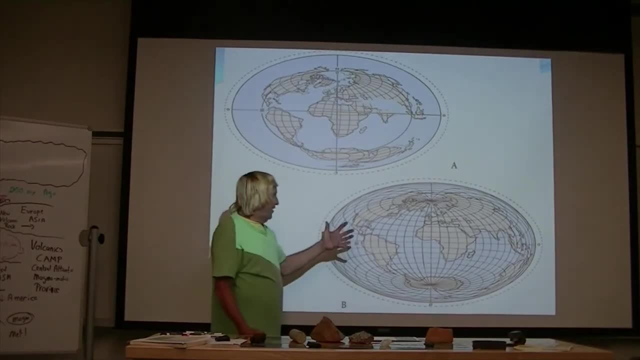 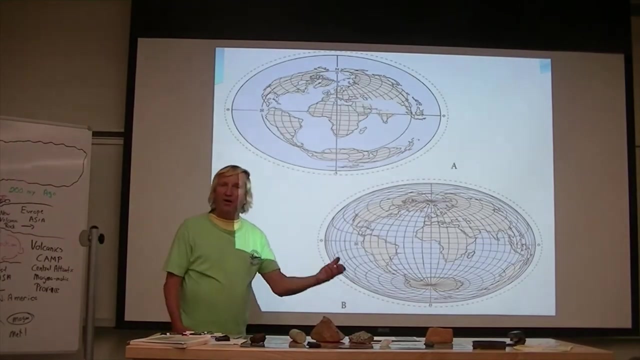 It was kind of as Pangea was forming, And this is marine organisms. And since then the Canadian continent, along Canada with the North American continent, has drifted north, And so now we find these marine fossils that grew in tropical waters, that we find now in a very cold. 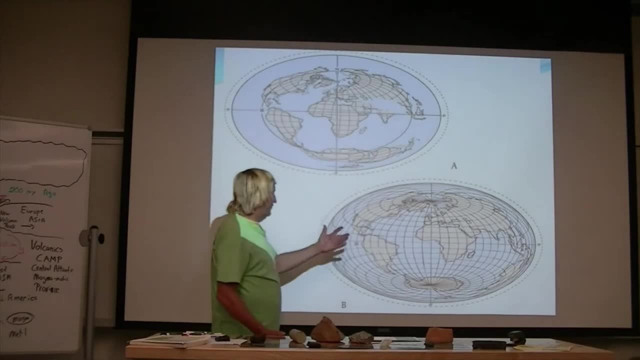 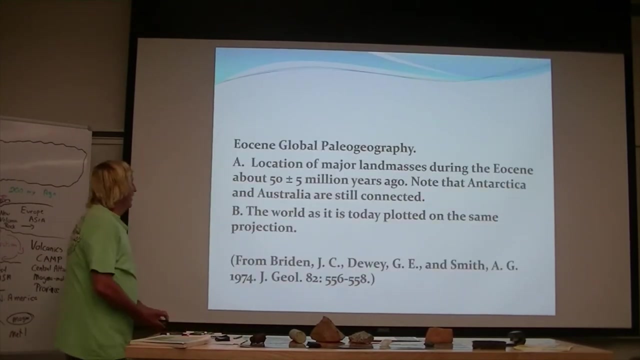 mountain climate. So that's what Wigner recognized. So Alfred Wigner recognized these fossils, because this does not make sense. These fossils don't belong here because they were formed. either the equator moved or the continents did, And that's where he came up with this. 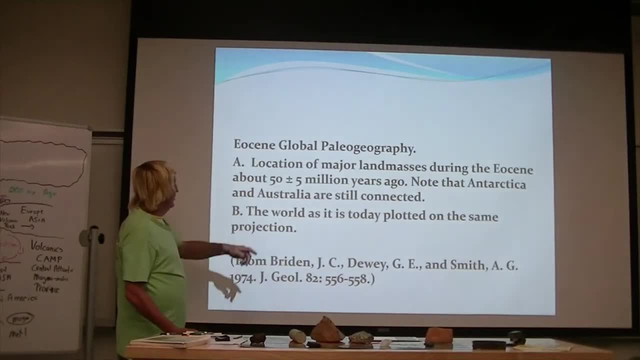 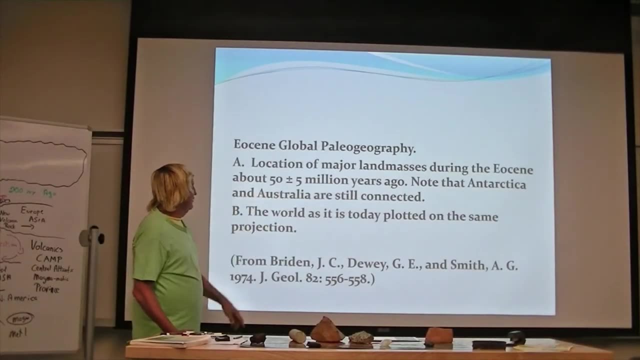 hypothesis of continental drift. So the Eocene, Kind of a neat time. So the paleogeography of that particular land mass in the Eocene about 50 million years ago, plus or minus five years. So Antarctica and Australia were kind of breaking apart. 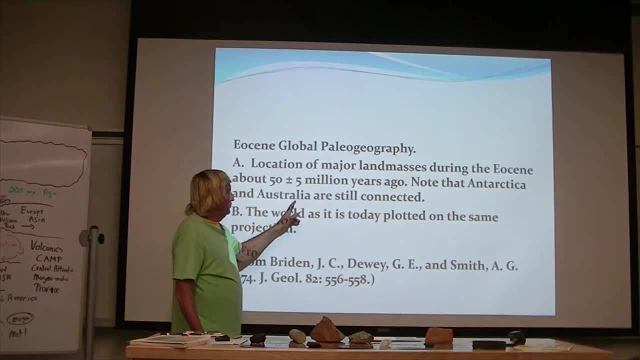 So really what once was Rodnia? So Rodnia was almost like a part of Gondwanaland broke away And then even that part breaks up into smaller pieces, So that part really consisted of Antarctica, Australia and India, And as India kind of drifted away, 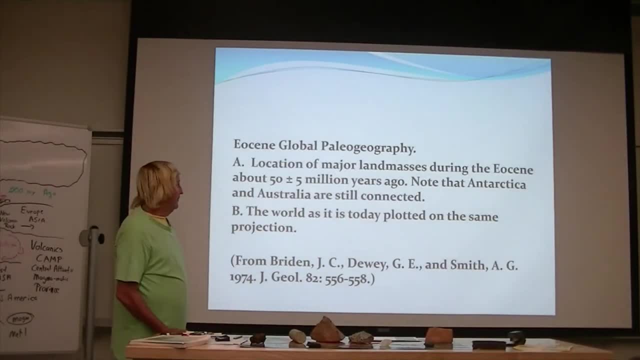 and broke apart. and then Australia and Antarctica are eventually going to separate, Parts of those microcontinents are going to move west- I mean east, along the Farallon Plate, And basically are going to accrete themselves onto the western portion of the North American continent. 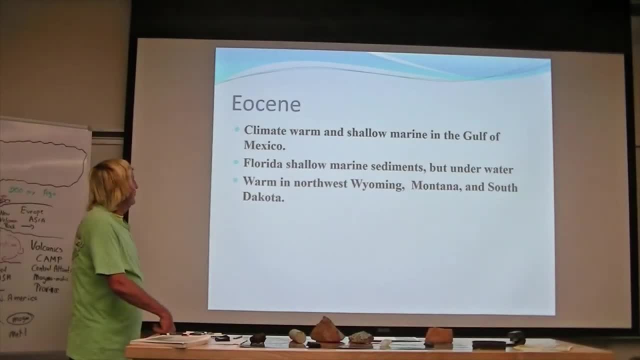 So Eocene Very warm. shallow marine Gulf of Mexico is pretty warm. Florida at this point is a very shallow marine sediment, But underwater, So Florida doesn't become a state until a little bit later. Basically today Wyoming, Montana, South Dakota are pretty warm. 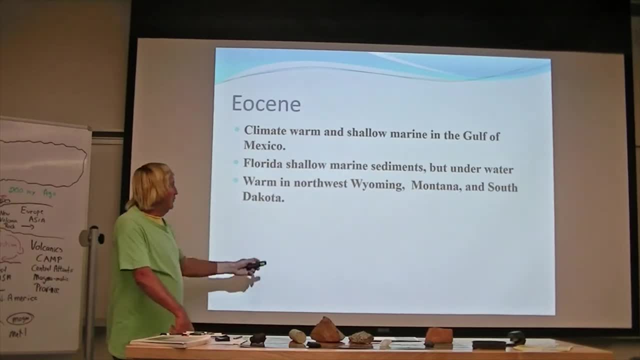 We find tropical fish in what we call the Green River Formation. The Green River is actually a river that feeds in the Colorado River system, And part of the Green River Formation is a shell that is full of subtropical fish. These are actually catfish. 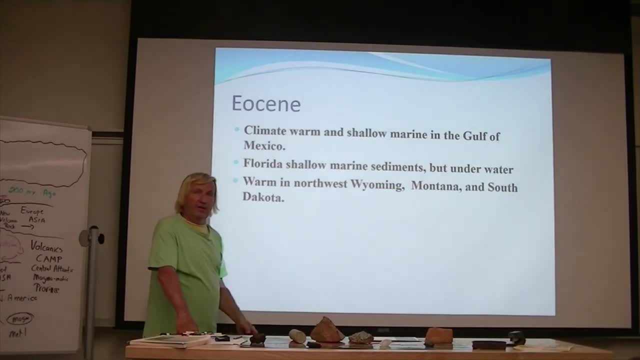 Very similar species live sitting off the southern coast of Florida. So we see these fish fossils up in today- Wyoming, Montana, Utah, Northern Utah- And we know that those areas at one time were pretty warm. So this is basically in the early. 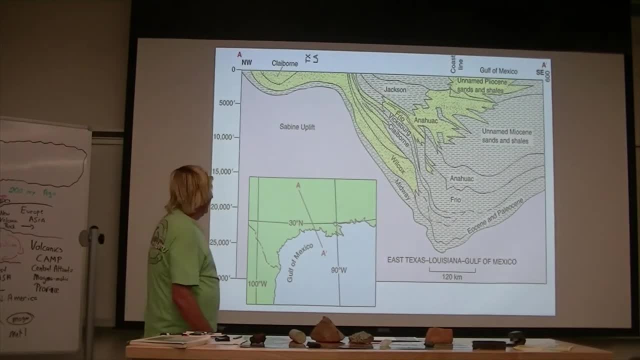 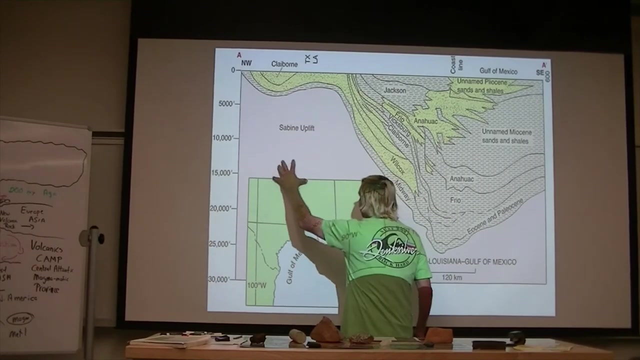 Cenozoic and near the Eocene. So what's happening in the Gulf of Mexico? here there is a huge because originally what happened when Pantino formed South America collides with what is now North America. This collision is going to result in uplifting of the Ozark Mountains. 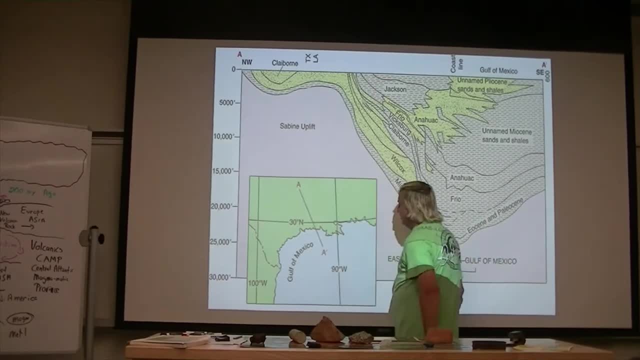 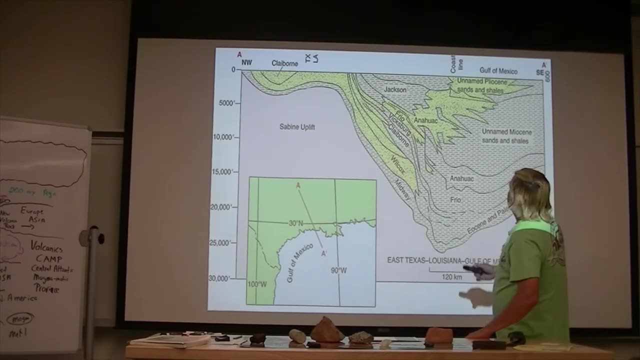 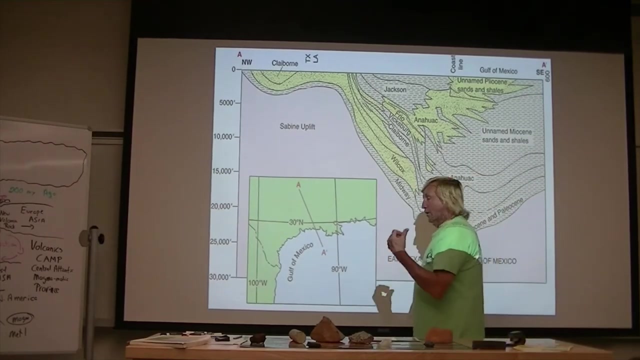 on Missouri And it's going to create a little warped basin in what is today basically Houston, Texas and Dallas, And so you get these huge accumulations and this is also going to accumulate a lot of hydrocarbons, which is why oil is found in Texas and Oklahoma. 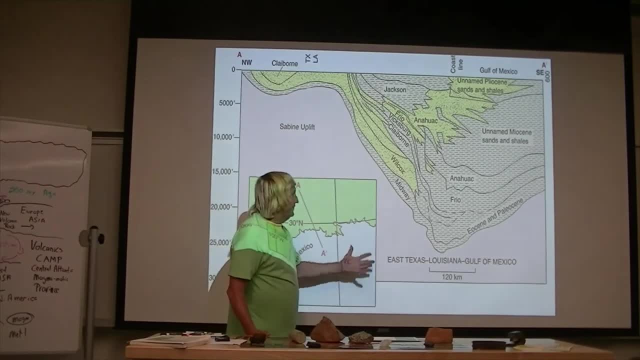 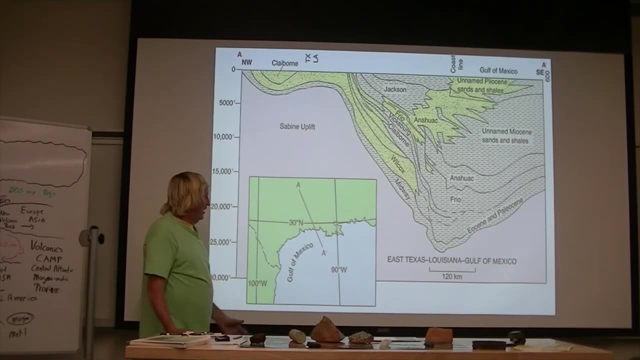 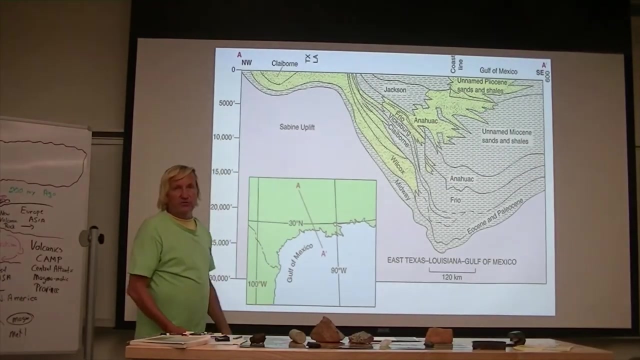 today Because of South America colliding, creating this little basin here. they said this is an accumulated and because this was pretty southern latitude, a lot of organic material was able to accumulate. So the oil deposits that we see today in Louisiana and into Texas and up into Oklahoma. 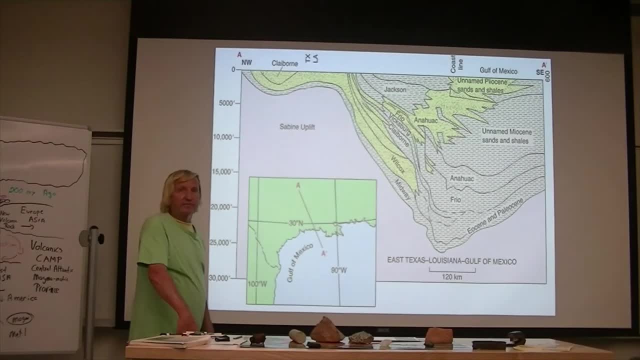 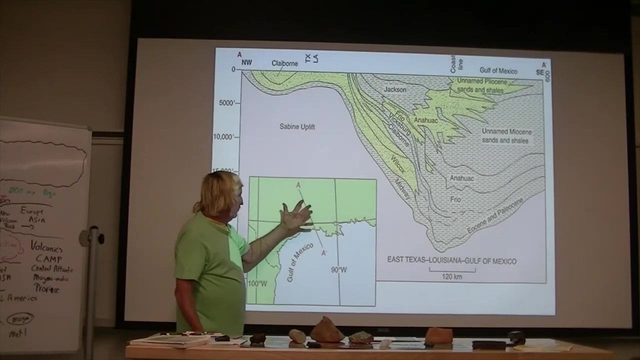 were all formed during this time, in the early Cenozoic, And it was due to a basin that was formed because of the continental collision. So when South America then breaks away from North America, when Gondwana land was formed and the peninsula was formed, 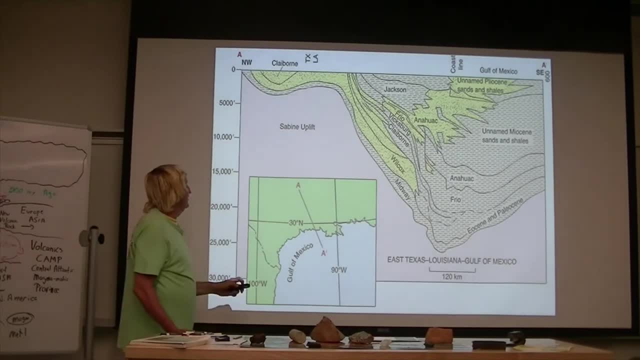 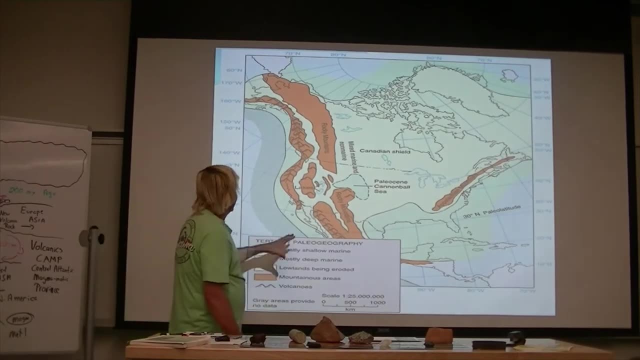 that wedge kind of filled up with sediment as erosion occurred. Now we start to see mountain building, certainly in the west. The Baja Peninsula is still part of Mexico- It doesn't get pulled away from Mexico- until about 20 million years ago, So that's a fairly recent. 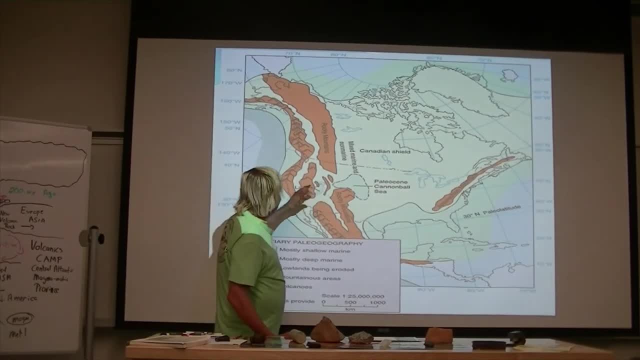 event. But what's going on in the middle of the distance between these mountains is there's some basins where water is being trapped. That water is very saline And you're going to see deposits of the gypsum, So some of the best gypsum in the 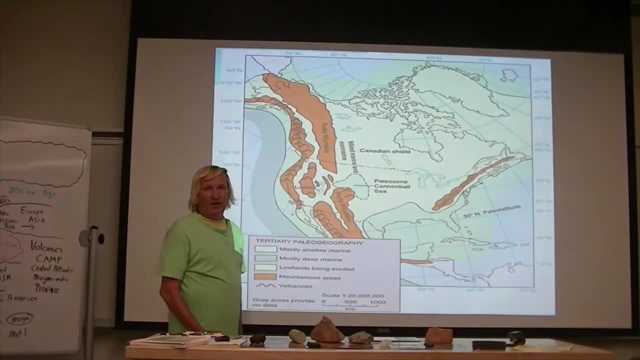 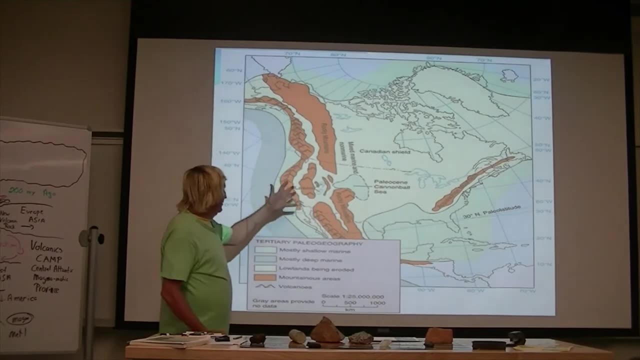 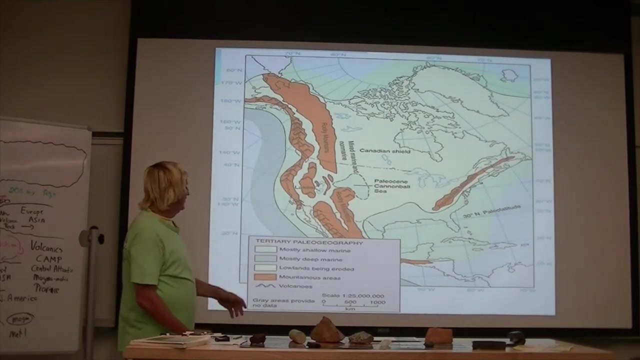 world. calcium sulfate is formed in Utah And these were trapped basins that were kind of almost remlits of the Sundance Sea, So these were basins that fill up with water. Very warm environments allow for the growth of a lot of gypsum. 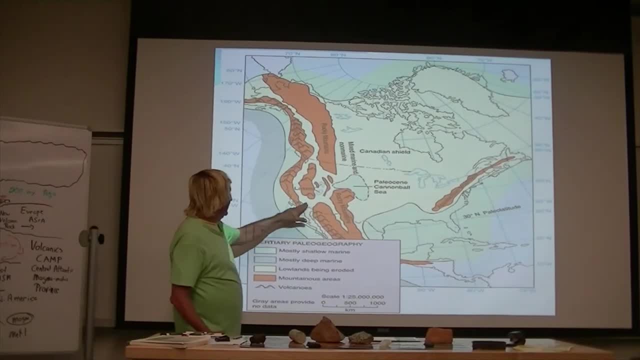 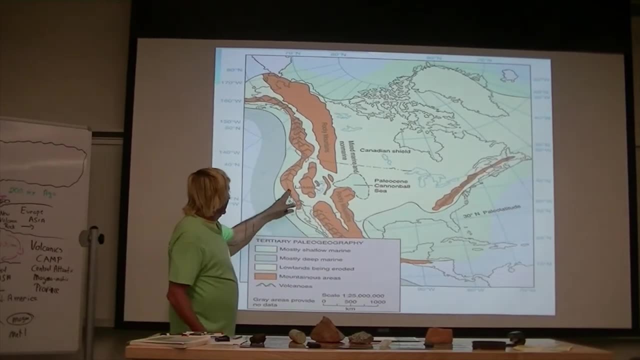 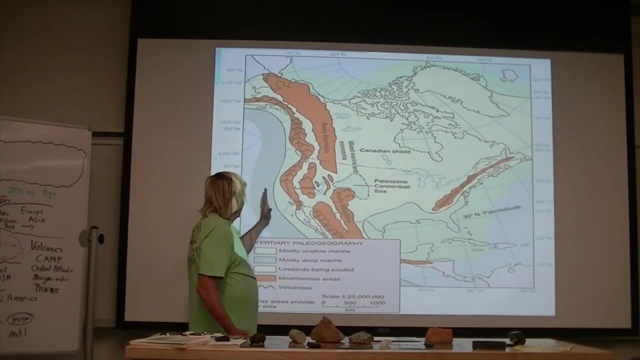 So in between the mountain ranges, this kind of green area, here are very shallow seas. Obviously the brown areas are areas of mountains, So you can see that along the coast of California starts to develop. A lot of these mountains are forming, not in place. They're forming because 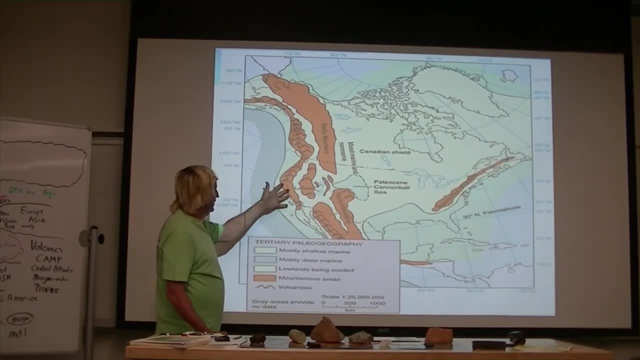 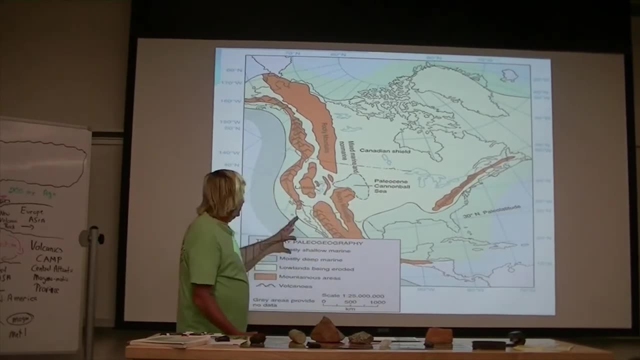 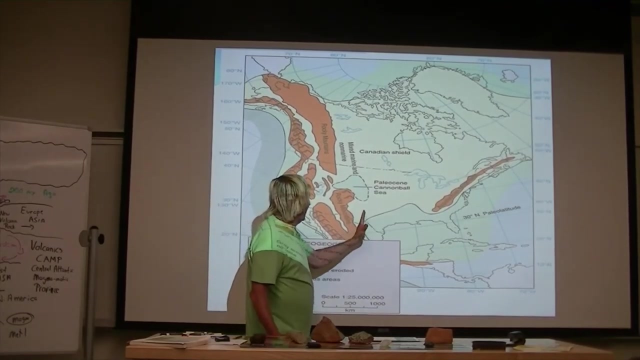 the Farallon Plate is pushing these new pieces of continent against the North African continent. It creates a rippling effect that goes all the way to Colorado. So because California is being accreted, all this terrain is being pushed onto California. it's causing a ripple. 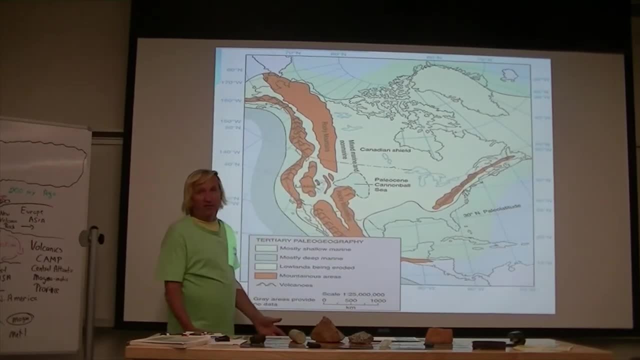 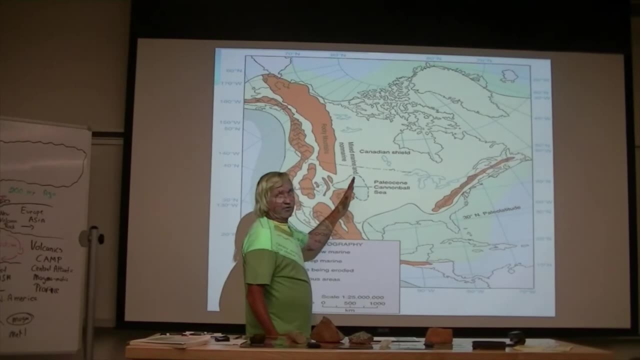 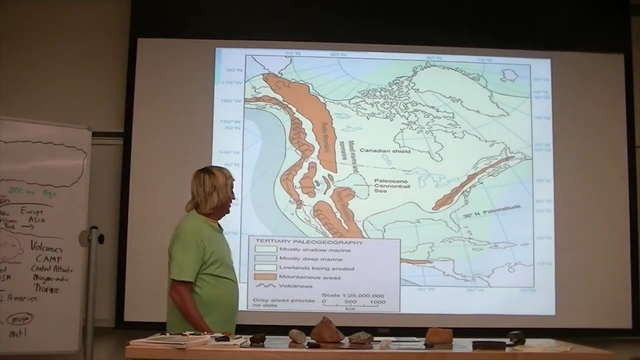 to occur right along where today Denver is the front range, And that was almost like a hinge. And so the North African continent responded by turning like this, Almost like an 80 degree turn, Creating what we call the front range, And that's. 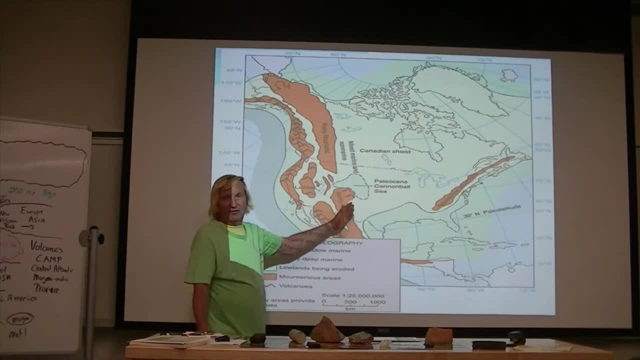 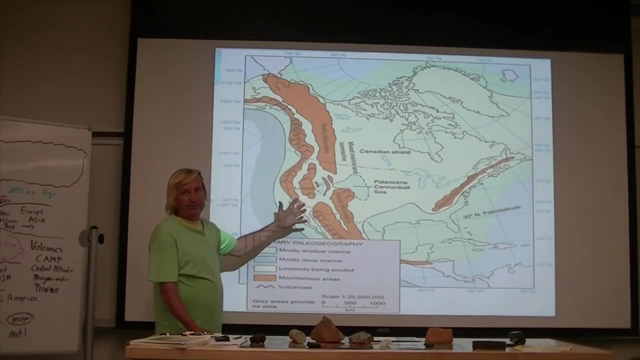 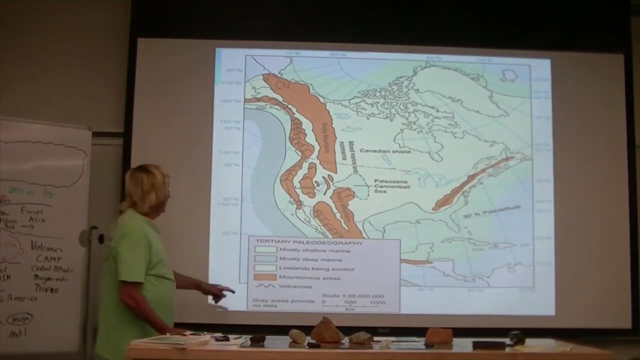 basically where the Rocky Mountains start. So the front range in Denver, Colorado, just to the west of Denver, Colorado, was formed because of continent to continent collision along what is today Eastern California and Nevada. So there are a lot of volcanoes occurring because that plate was subducting. 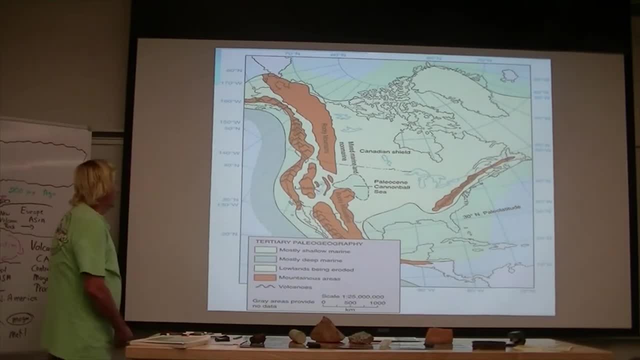 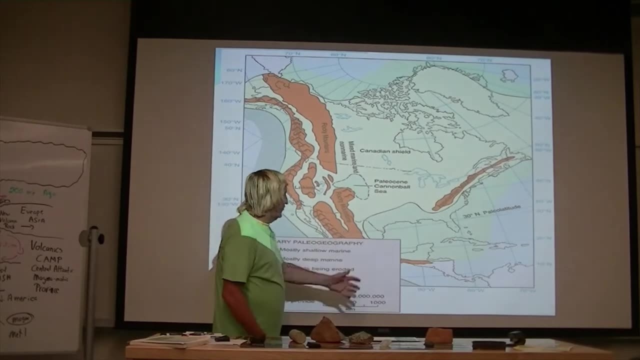 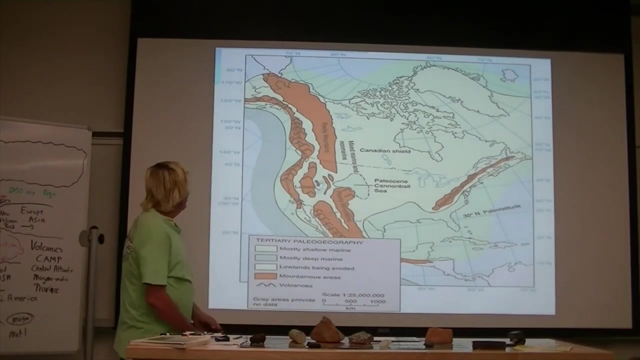 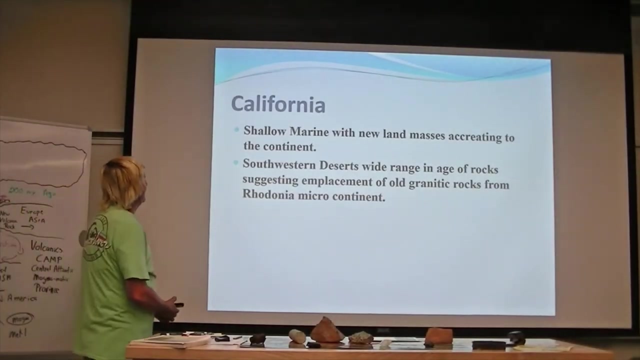 creating chains of volcanoes, And you have to realize at the time that this is still fairly subtropical. Here this is 30 degrees north latitude, so it's pretty warm, And so California has some very shallow marine sediments with new land masses that created the continent. 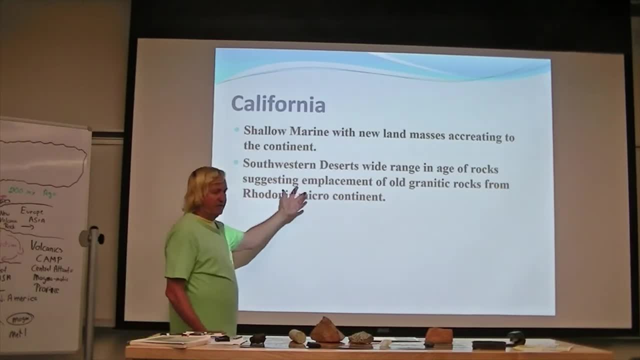 And so if you look at the southwestern deserts, you'll see rocks out there that are stromatolites. These are algal blooms that were formed in Australia and we find them in Eastern California, and those rocks are 1.3 billion years old. 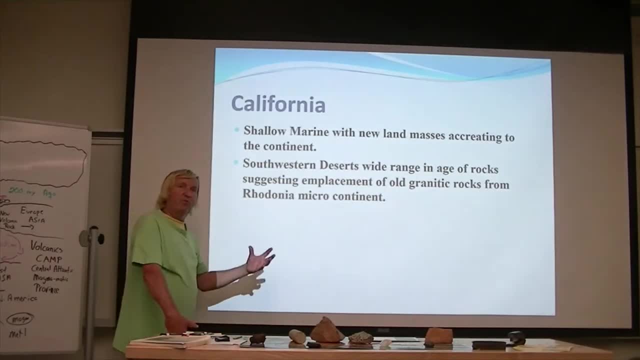 We find Ravikivi granites that are 1.4 billion years old, and they'll be right next to some paleozoic marine limestones that are Permian in age, that are 250 million years old, And so you see this 250 million year old rock next to a rock. 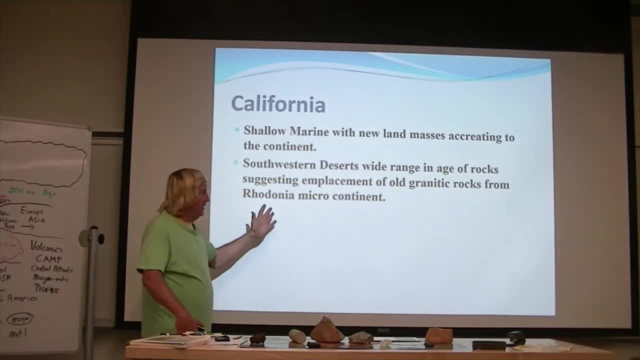 that's 1.4 billion years old. So you have a dramatic change from one mountain range to the other, which really explains that these granitic rocks and some of these rocks came from this microcontinent we call Rhodia, which broke away from Australia and was carried by the Farallon Plate. 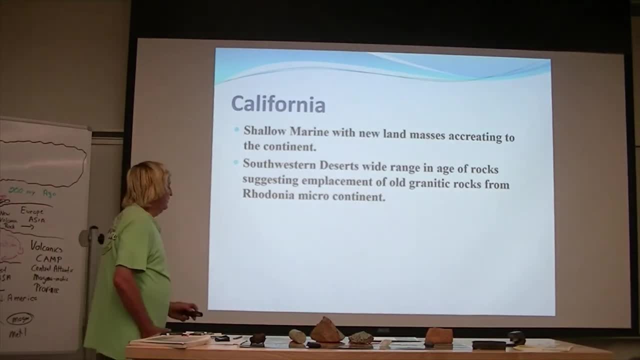 and all this material was pushed onto the western United States. So if you were to explain the western United States throughout the Cenozoic, you would classify it as accretionary tectonics. Accretionary tectonics. 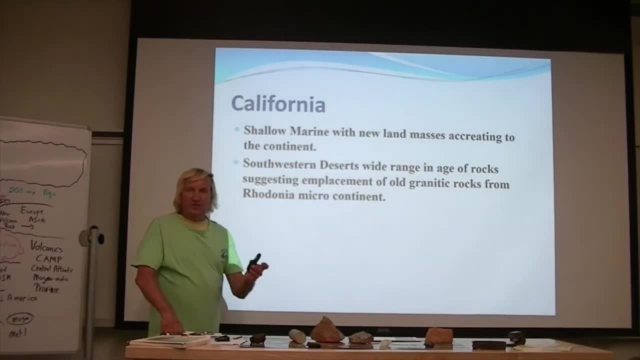 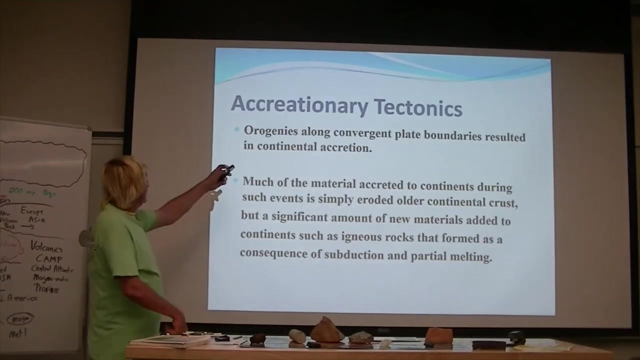 So we're basically a collage of a bunch of small little microcontinents that all plastered themselves onto the North American continent by the Farallon Plate, that act like a conveyor belt. Pretty interesting geology, Very complex geology too. So this accretionary tectonics- 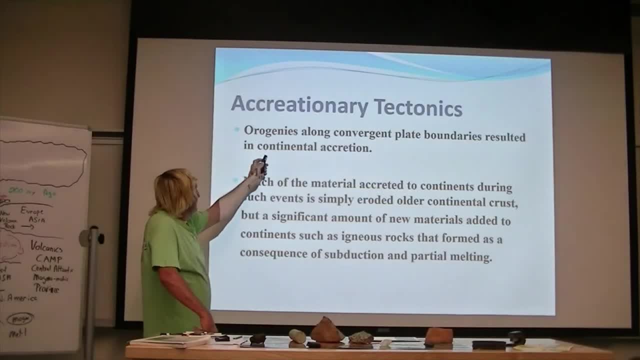 you know, it originates along this convergent plate boundary, resulting in a continental accretionation. So in the South Mountains we can see four distinctive belts of opalite rocks that are indicative of continental masses coming together and suturing themselves onto a continent. Pretty impressive. 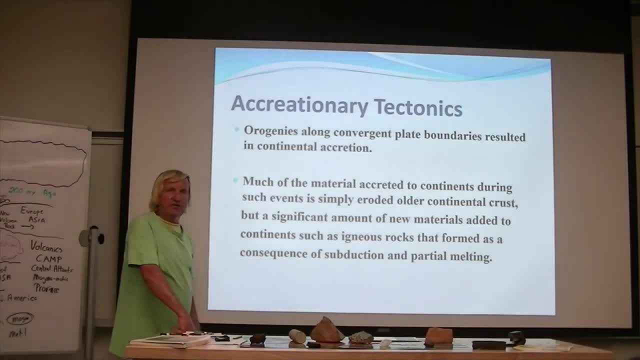 And as we explore the southwestern United States, the geology there is so complex because of the diversity of the rocks and the age ranges. nowhere else do you find rocks like you'll find a mountain range. that's rapid kiwi granite here And the next mountain range. 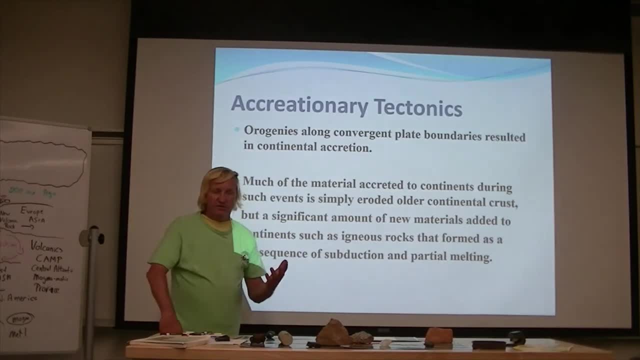 across the valley is going to consist of sedimentary rocks, marine rocks that were formed in a shallow oceanic environment, And this is why our geology is so complex, because we're just basically a bunch of ideas that just got stuck together and say: here, guys, figure it out what happened. 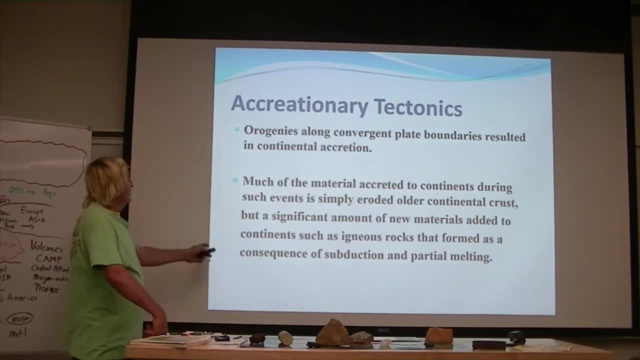 And it's quite a mess right now. So much of the material created the continents during events. you know we had older continental crust. we also had some new materials being added because rocks were weathering, they were being shed out into the oceans and then 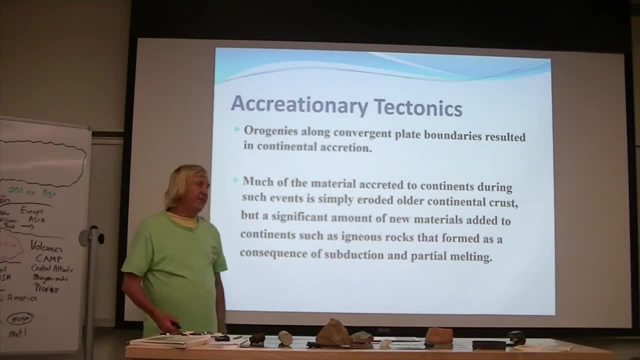 that material that was shed out into the ocean was then pushed back onto the continent. That explains the foothills of the Santa Ana Mountains where we went on that field trip- or I went on the field trip with my video camera- those rounded conglomerate sediments. 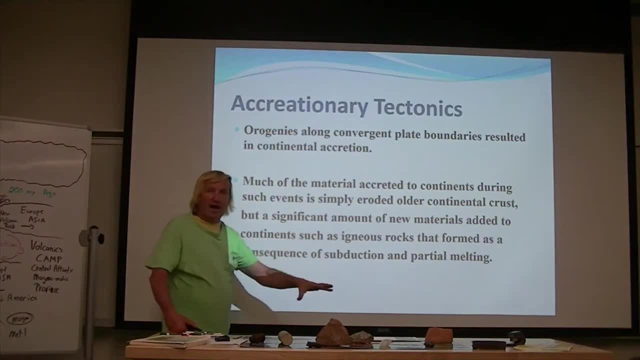 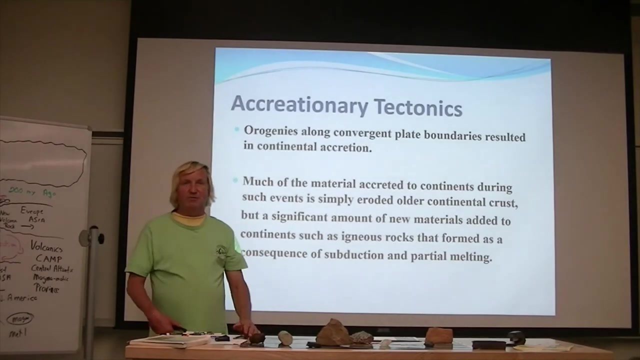 were material that was eroding off the continent, being shed out into the ocean and then later shoved back onto the continent again, Almost like a full circle. you know, Starts on the continent, goes to the ocean, is pushed back on the continent again, and now through the act of stream erosion. 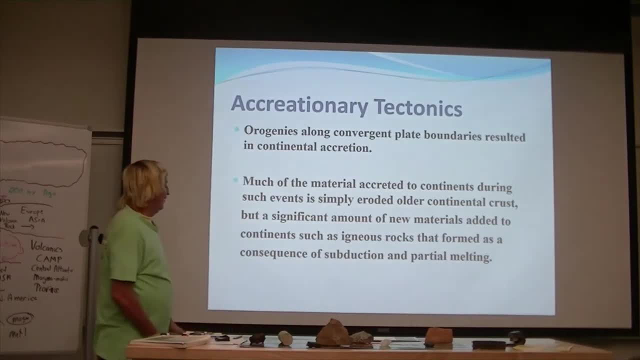 it's being eroded back down again. So it's amazing how that occurs. We have subduction going on. we have igneous materials, we have big batholiths that are forming underneath the North American continent. Those batholiths are going to slowly. 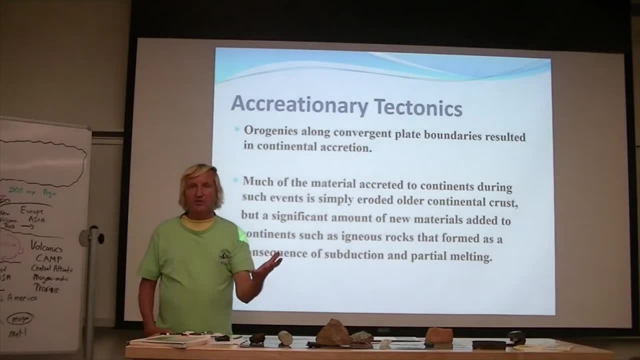 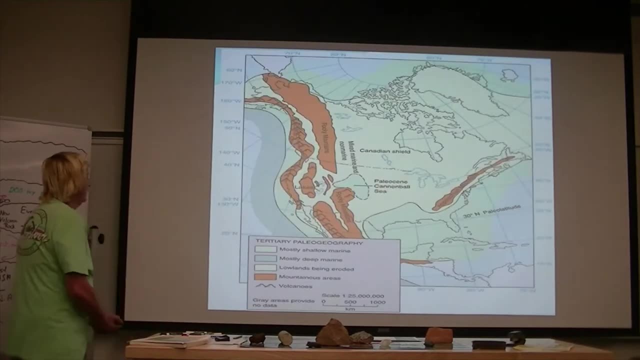 cool. eventually, as they cool, they're going to form granitic rocks and they're going to be uplifted into what is today the Sierra Nevada Mountains. So what's going on in the western United States is we start to uplift and, as we uplift, all these very shallow seas are just going to go by. 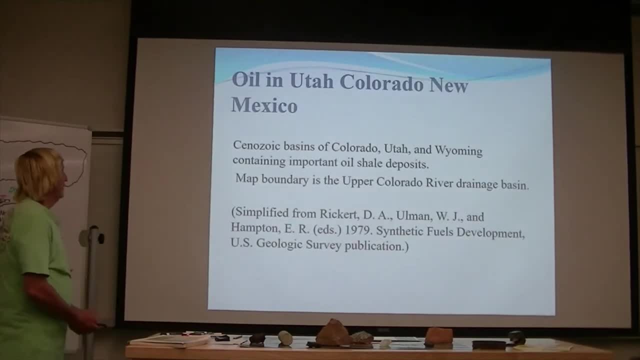 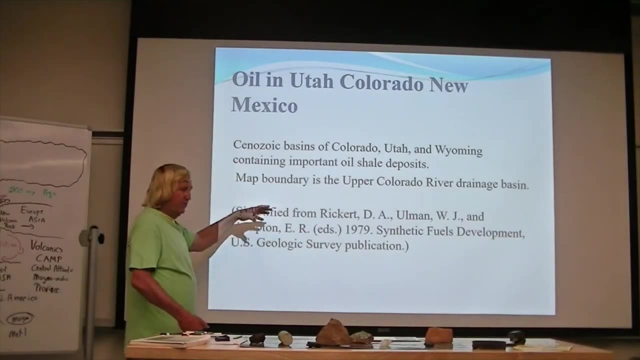 the way They're going to drain off the continent. So oil in Utah, Colorado, New Mexico. these are huge basins, cenozoic basins, so this is early to mid cenozoic. a lot of accumulations of organic material got trapped in these. 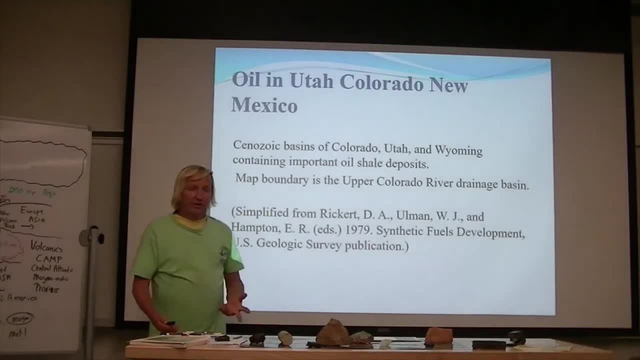 basins. So you need three things. for oil, You need a source rock. You need a rock that's rich in organic material. The second thing you need is a reservoir rock. That's going to be a rock that's going to absorb all those hydrocarbons. 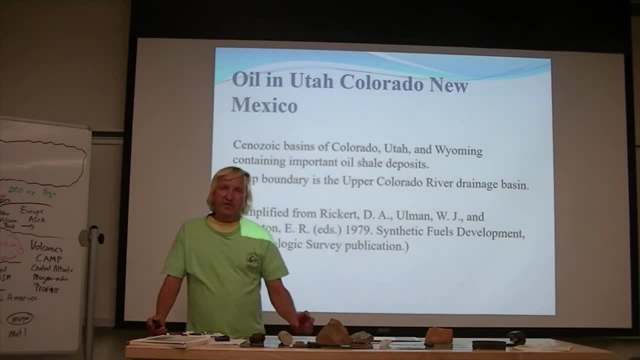 and sandstone is the best material for that. Sandstone is very porous and it has high porosity, so it can absorb a lot of those hydrocarbons. And then the third thing you need is a structural trap, A fault full of rocks, and that's where we find. 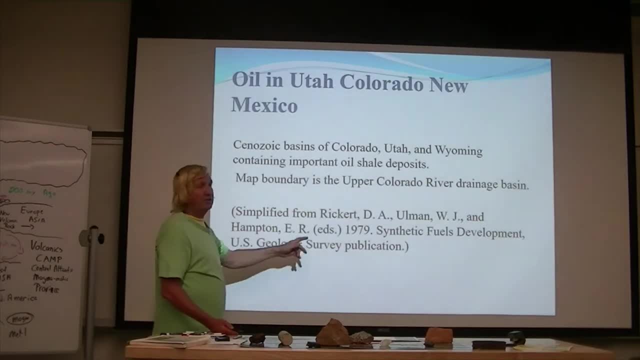 oil in Colorado. We find it in New Mexico. New Mexico's got some really good oil and they supply a lot of that oil- that refined oil, in the form of gasoline, to Arizona, Which is why gasoline in Arizona is a lot cheaper- It's like a dollar. 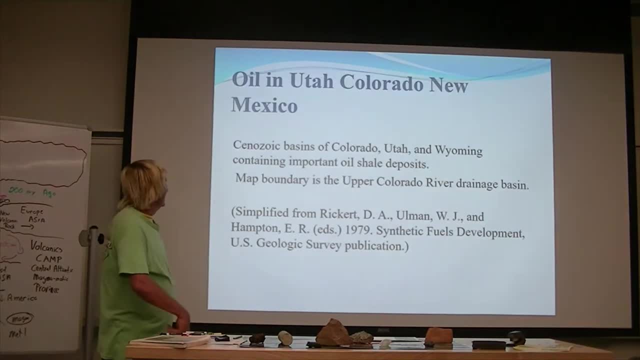 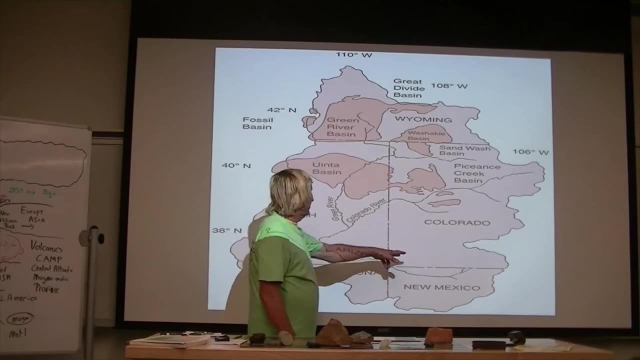 a gallon cheaper than California. So this is Utah, Colorado Four Corners area, And so we have these basins that just accumulate large amounts of hydrocarbons. Here's the Green River, which feeds in the Colorado River, And there's actually a 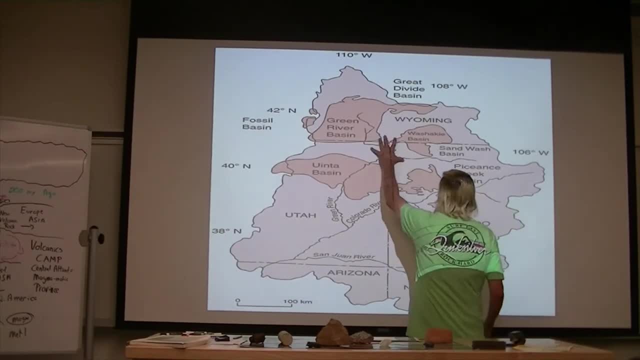 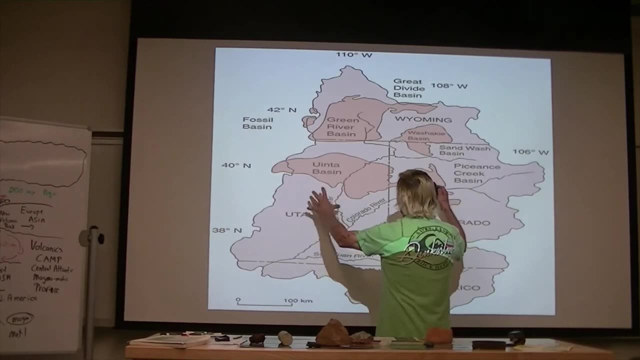 formation called the Green River Formation. So during the Eocene there was lakes out here. These lakes were then being polluted by volcanic eruptions, So there were dramatic volcanoes going off, shedding a lot of ash, And so the fish that were living in these. 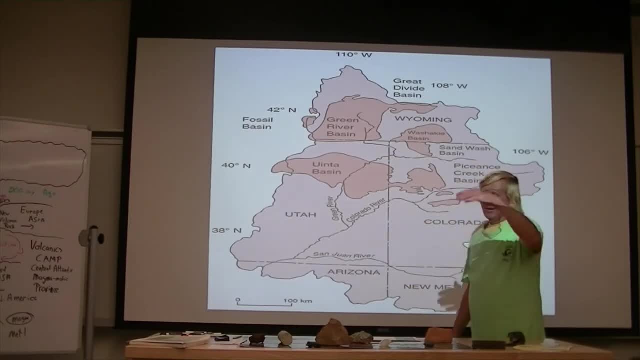 little lakes were being rained upon by volcanic ash and instantly buried. So remember, when we talked about fossil preservation bias, That one of the advantages is to be a small organism, An organism with hard parts, But no matter what, when it comes to the fossil preservation, you have to be. 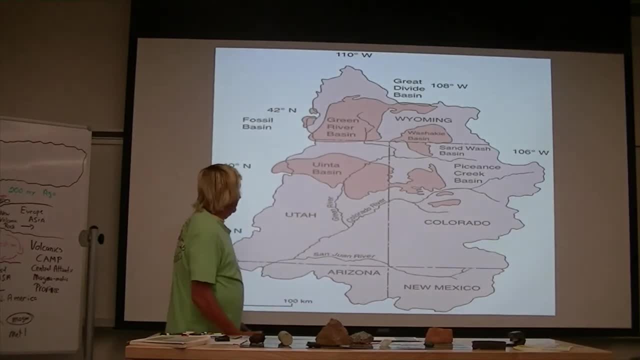 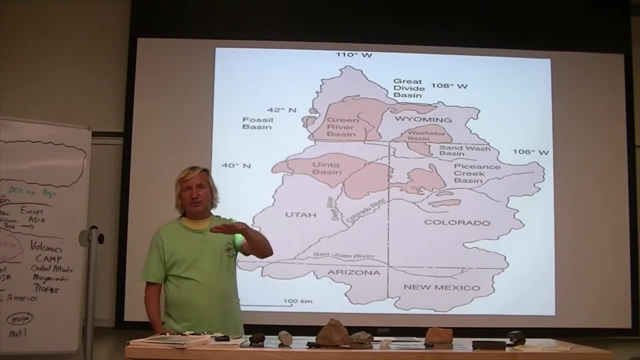 buried rapidly. And in the case of these fish in the Green River Formation, they were buried very rapidly because, as the volcano erupted, it emitted so much ash that the ash basically infiltrated into the lake, Super saturated the waters of the lake with all the silica rich ash. 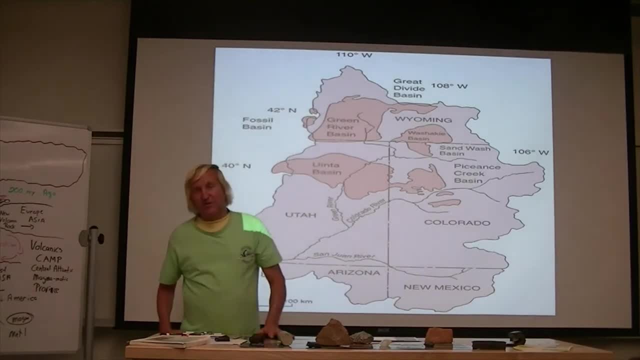 which was going to kill the fish. Fish sink to the bottom and then that ash is going to accumulate and bury the fish, which is why the Green River Formation has such a very good history of fossil preservation. So this entire area here, a lot of basins. 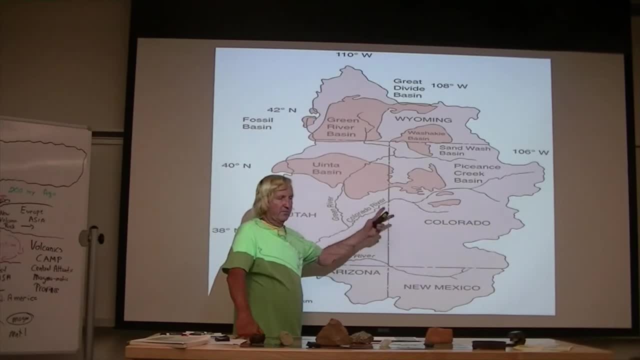 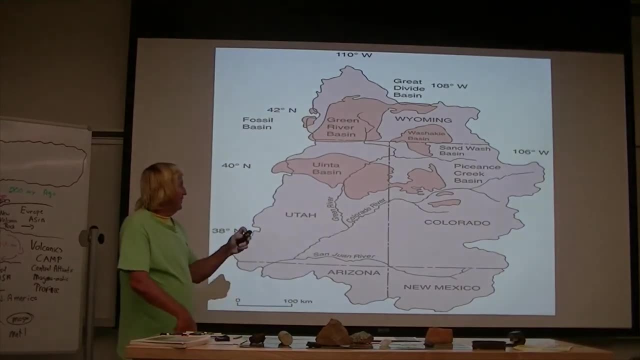 and then, after these basins develop things like gypsum and oils and salt, They're all going to be uplifted to very high elevations because of this continental environment where you just got one train after another train being created onto the North American continent. So here's another nice little. formation where we have the Green River Formation kind of sandwiched in that makes a birdie formation. So when we find these formations, these are very common throughout Colorado, Utah, into as far east into the Dakotas, And so we have all these accumulations. 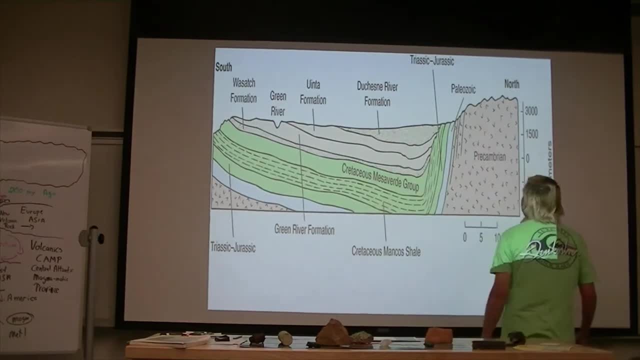 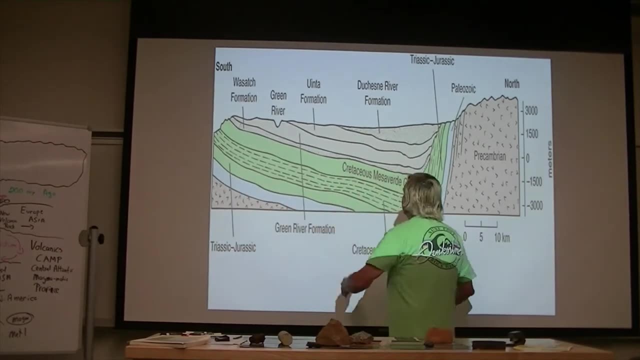 of basins. You have pre-capping rocks now being uplifted along the Rocky Mountains, So you have the Front Range uplifting, You have the Sierra Nevadas uplifting and in between of these mountains are these basins, and these basins are going to be huge hypercarbon. 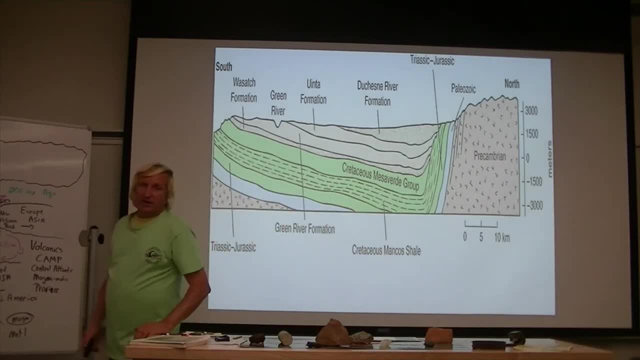 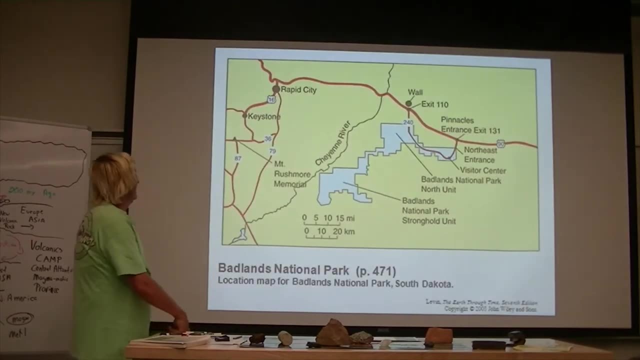 sinks and traps. Materials are going to accumulate there and then eventually form things like oil and oil shale. So this is Badlands National Park and the Badlands kind of. really, the reason they call it Badlands is because this is a sequence of sedimentary rocks. 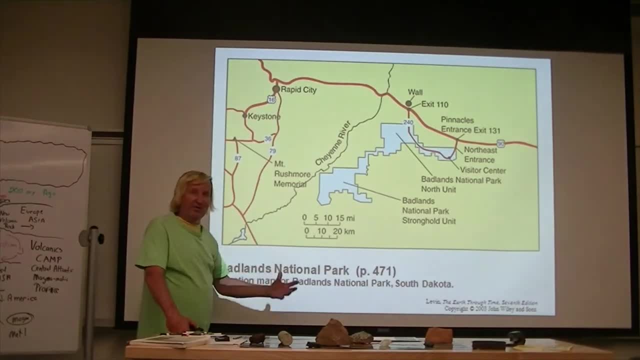 that erode into rills. So you can't really build on this material. so that's why they call it Badlands. You don't want to build there, So the Badlands, basically, are part of these sediments that later are going to be uplifted and then eroded. 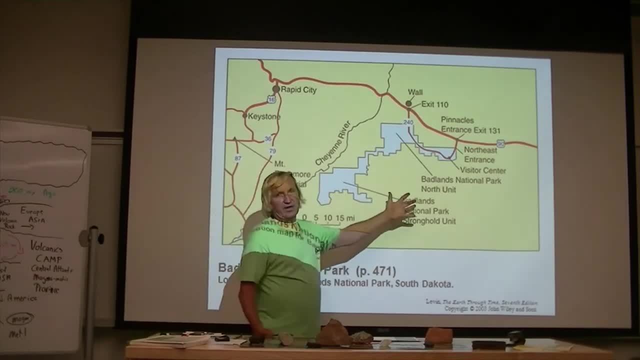 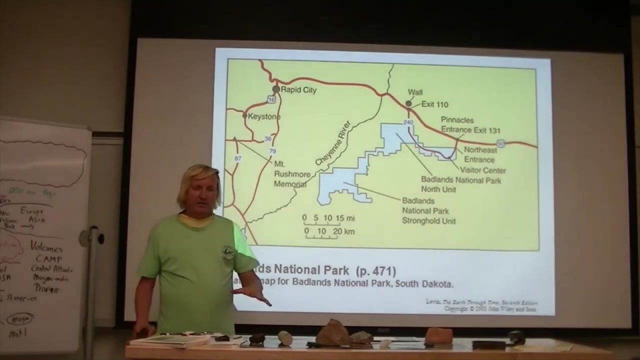 A lot of marine fossils within the Badlands, A lot of dinosaur fossils, Just a huge community of fossils. So this area suggests that, as these mountains are uplifting, a lot of sediment is being shed off of these. So you have to realize that Denver, Colorado, 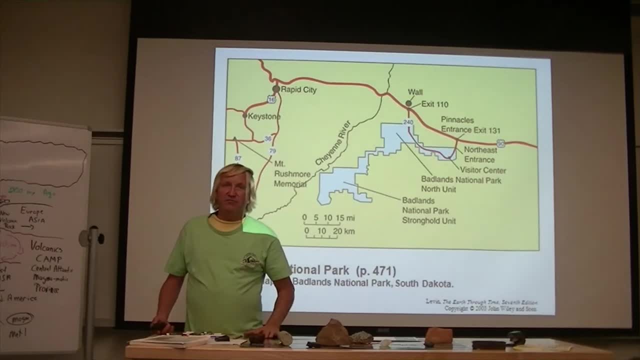 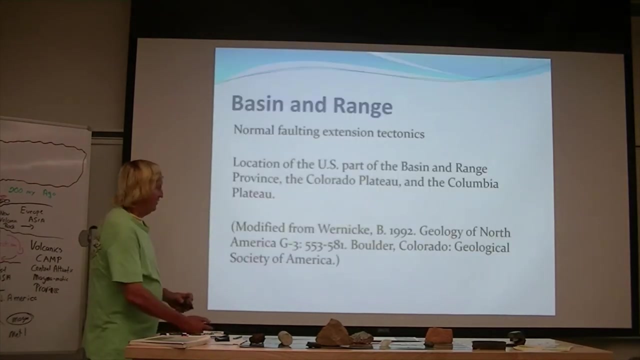 is a mile high in elevation, 5,280 feet. So even Denver Colorado has been uplifted and then filled in with sediments because of what happened in California. So California influenced Denver Colorado. Interesting point there. So basin range: 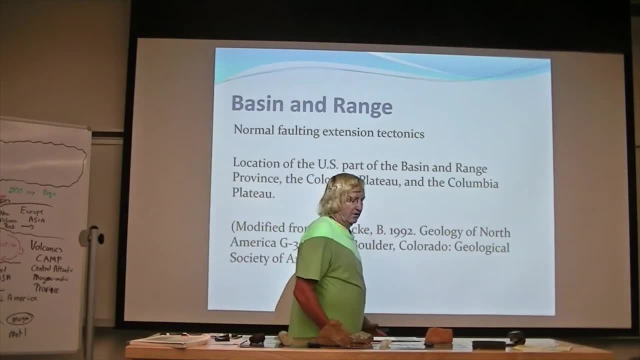 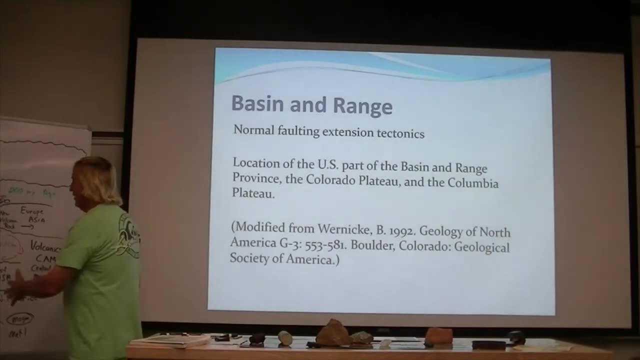 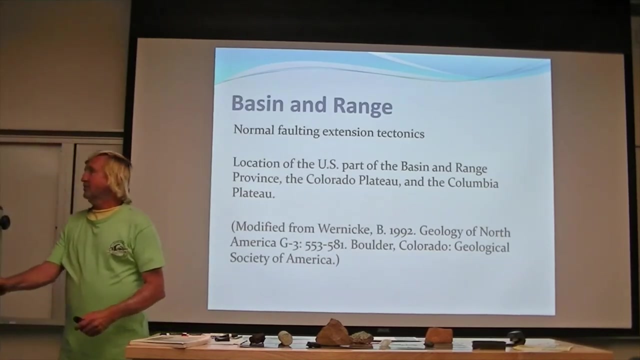 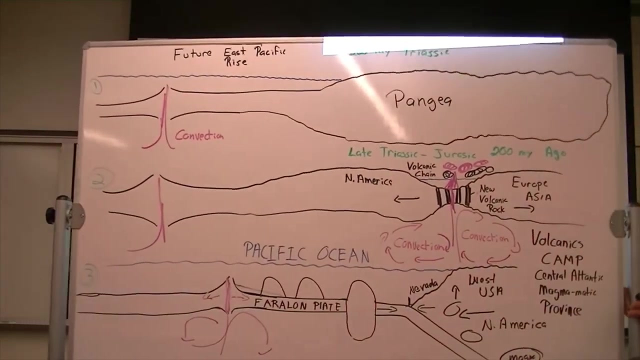 This is what's going on today. So after the Farallon Plague disappears, it goes underneath the North American continent. The North American continent now overrides that spreading center. So what happens is the North American continent overrides this spreading center here. So the Farallon Plague carrying 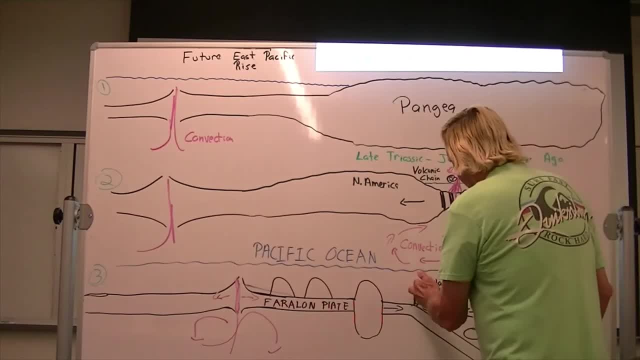 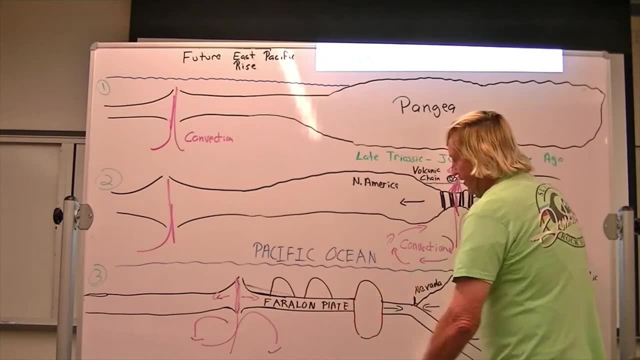 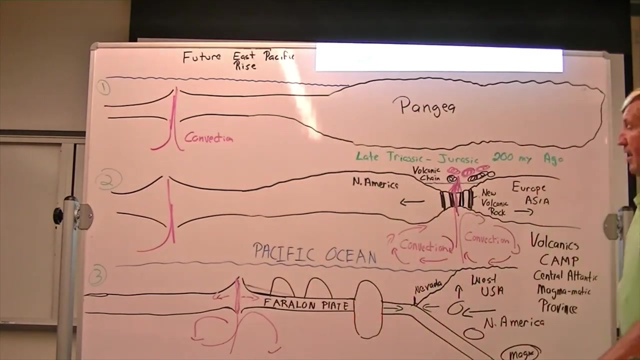 all these little microcontinents is going to stick everything on in California. So here's Nevada. at the time California didn't even exist, So California and Nevada kind of grow And eventually the North American continent is going to make contact with this center. And when it does. this is when the San Andreas Fault was born, And ever since then the San Andreas Fault has been moving to the east. So when it originally formed, 27 million years ago, the San Andreas Fault was right along the coast of California. It was a coastal California fault, Much like the Newport-Inglewood Fault is today. So our Newport-Inglewood Fault, which actually starts in Hollywood, goes through the Los Angeles Basin, through Long Beach and then down through Sunset Beach- actually Sunset Beach- and along the Pacific Coast Highway. There's a lot of argument and suggestions that that fault was actually the San Andreas Fault at one time. And it's no longer the San Andreas Fault, because the San Andreas Fault has now moved east And every time it does it creates a new fault. 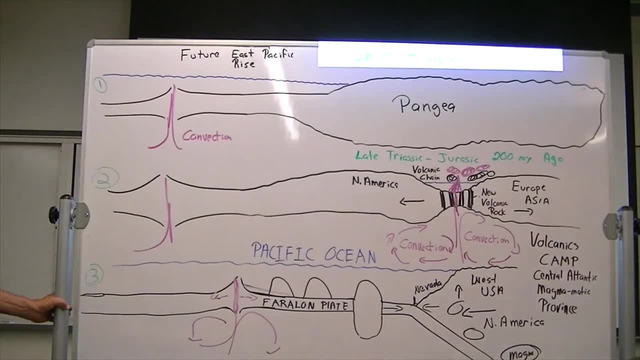 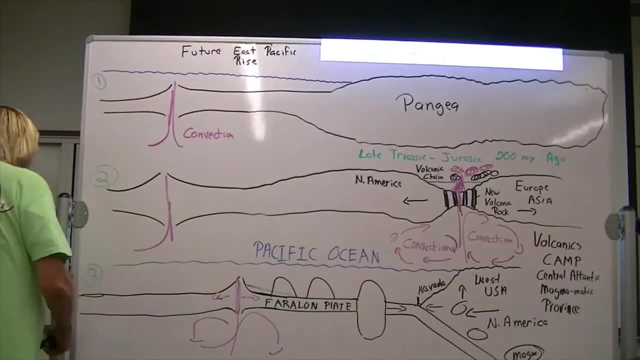 And so, as time goes on, the San Andreas Fault is moving east And, as the San Andreas Fault is now this brain center, what it's doing is it's stretching the North American continent. So the North American continent is being stretched, and as it stretches it, 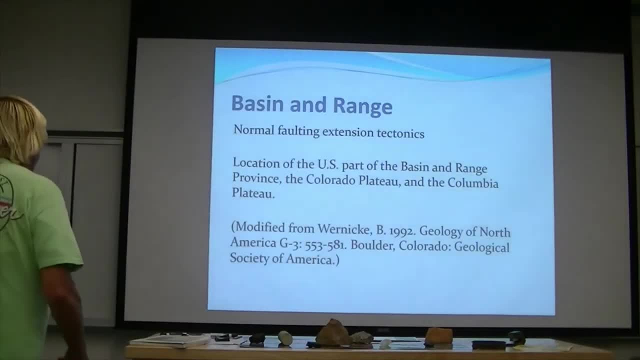 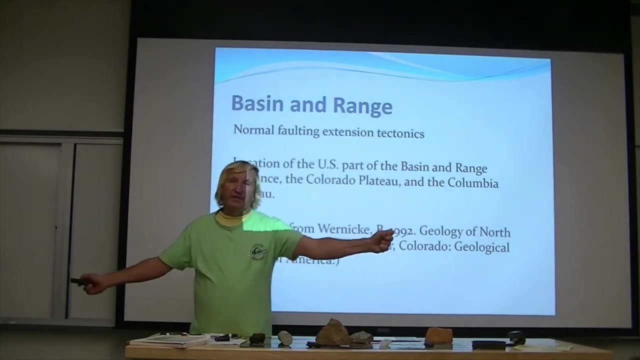 it subjects the continent now to tension. So when rhodium was colliding with the North American continent, it was creating compression. Things are coming together. They're folding Now that we compressed everything. the San Andreas Fault is going to pull everything apart now Tension. 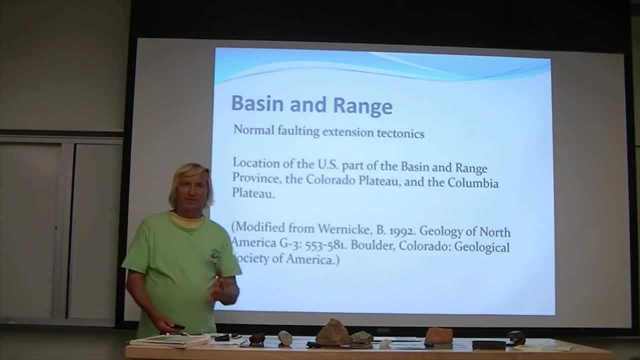 The absolute opposite of compression. We're going to pull it apart And when we pull it apart, rock is going to fracture. More pulling is going to take those fractures and allow movement to occur through it And this is going to result in the down-dropping. 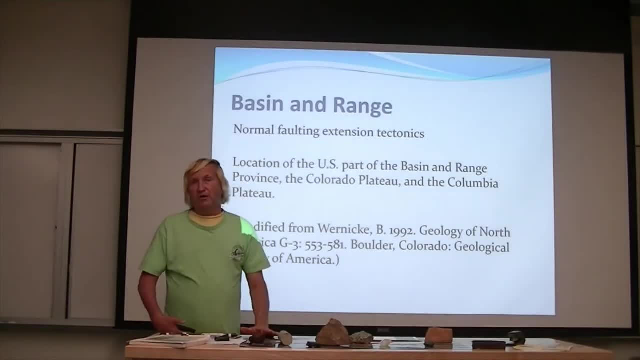 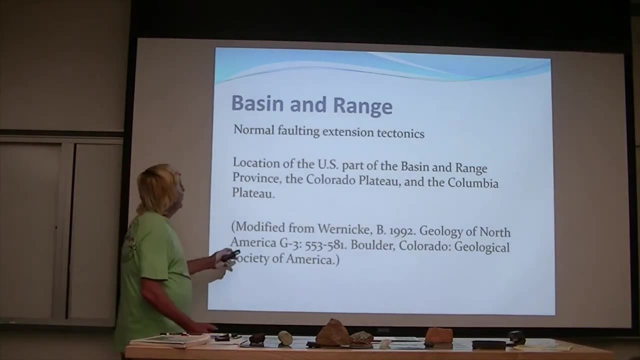 of basins like Death Valley to form a new topographic setting called basin and range or horse and grove. The funny thing about that is the one area that kind of divides, that is, the Colorado Plateau. And the Colorado Plateau is a sequence of marine sediments. 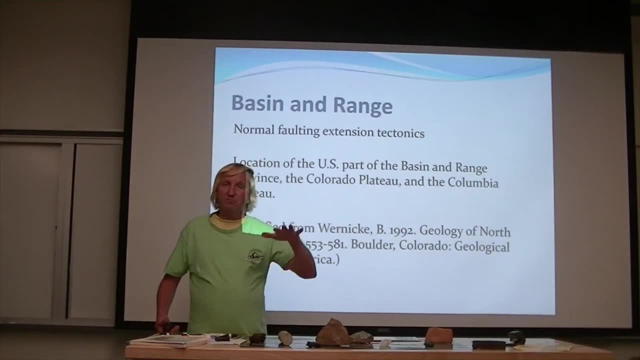 that are paleozoic, Cambrian to Permian, And those marine sediments, instead of tilting, instead of folding like all the other sediments around them, uplifted slowly and they kept their original horizontal positions, Which is very unique. Most of the rocks in the western United States. 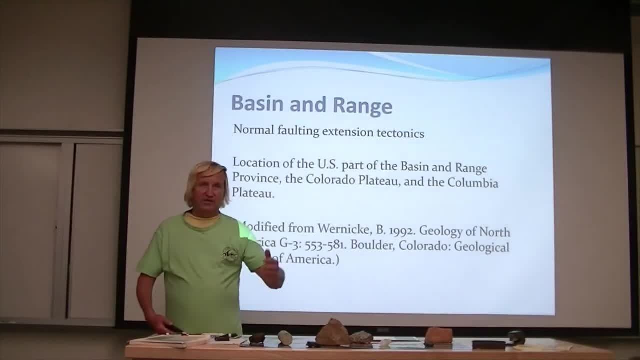 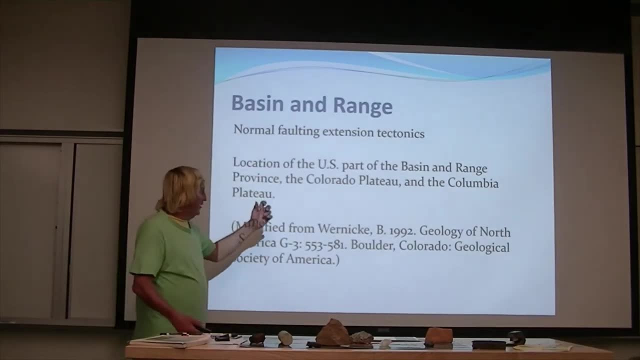 are folded. They're folded into anticlines or synclines, Or they're faulted, Or you have older rocks on top of younger rocks, But the Colorado Plateau kind of really survived, very uniquely, And I got some of this information out of some journals. 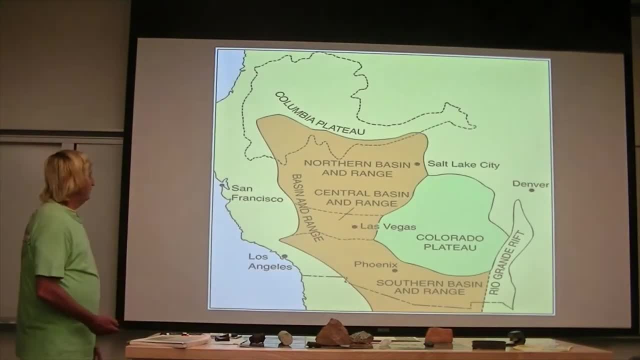 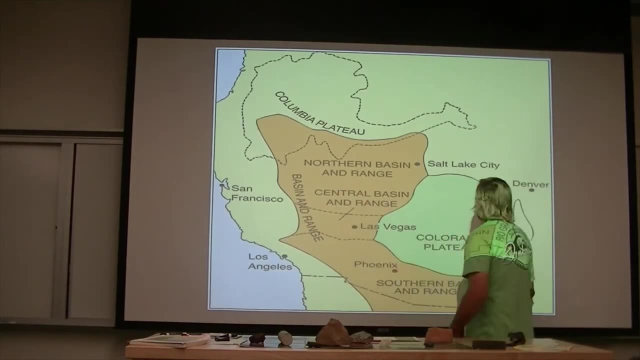 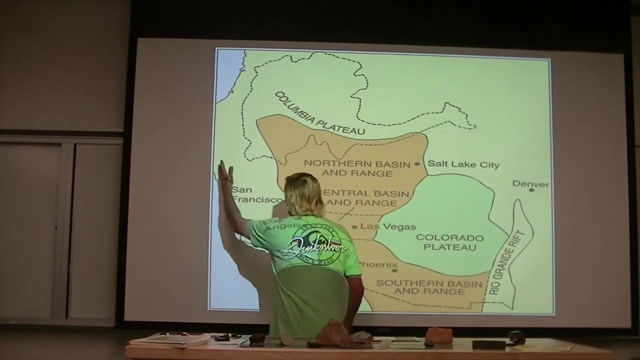 that I've been reading. So here, the Colorado Plateau. It doesn't fit everything else that's going on in the western United States. So over here this is being hinged and folded upwards. Everything over here is uplifting A lot of coasts. 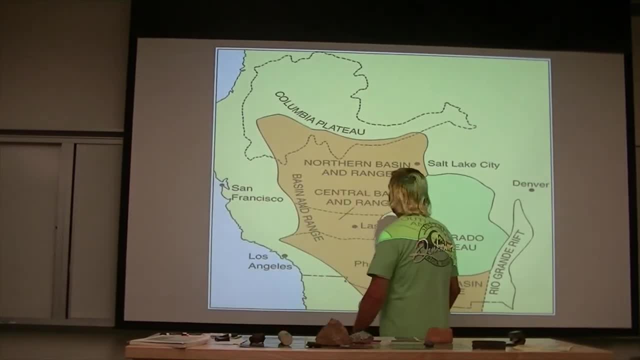 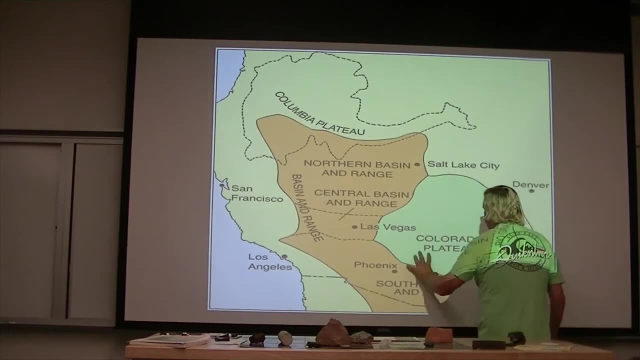 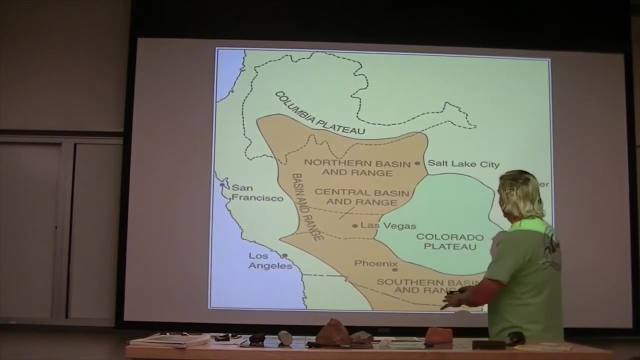 are uplifting. There's a basin here called the San Joaquin Valley. Now these mountains are being extended and stretched out, forming the basin range. But the Colorado Plateau kind of was independent, It kind of did its own thing, It didn't follow what. 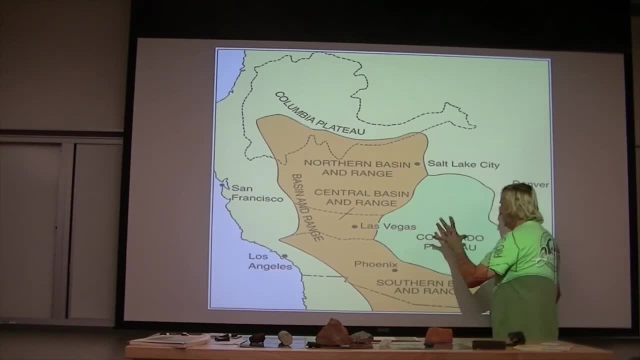 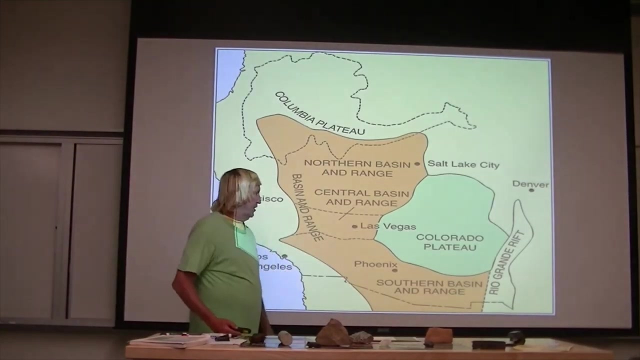 was going on geologically everywhere else. And it's kind of neat because the Colorado Plateau is really a good look back into the Precambrian, all the way up through the paleozoic, And it's kind of a rare view of the past. So the Colorado Plateau, 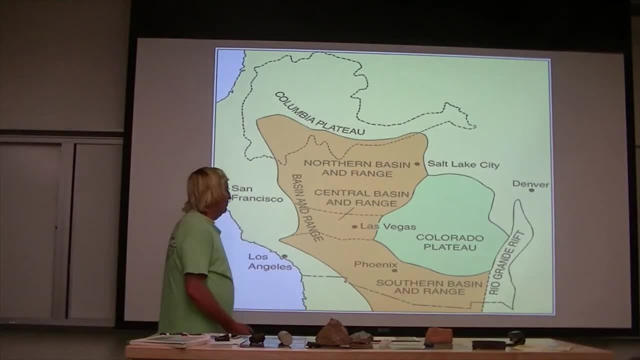 is kind of a unique place And so, within the Colorado Plateau rivers have cut down through us, showing the sediments, being the Grand Canyon formed by the Colorado River and other canyons such as the San Juan River out of New Mexico, are really exposing sediments. 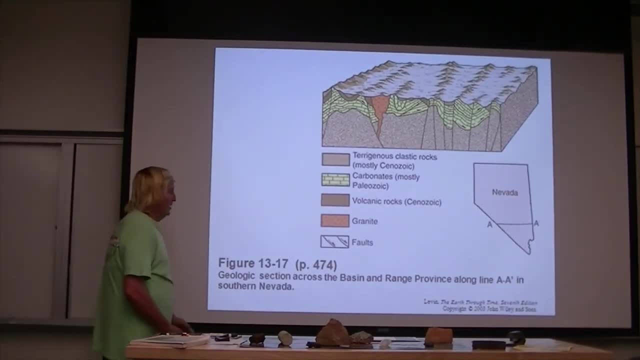 So Nevada right now is probably the poster child for extensional tectonics because it has been stretched And if you do a cross-section A to A prime across the state of Nevada you'll find you'll go from mountain range to basin, mountain range to basin. 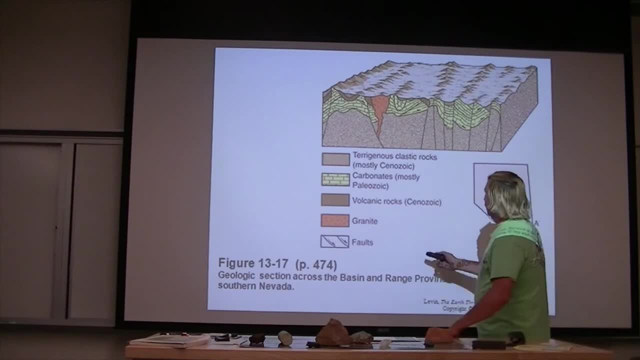 and if you look at some of the rocks that are in Nevada, you'll find a lot of carbonate, paleozoic marine limestones, shales, and of course then you'll find some very old granites, even some right bikini granites. Which suggests that Nevada was formed because there was marine sediments that were pushed up and then some other exotic material was added to it. So the geology is such a collage, a hot pot, that it is just really a very difficult geology. 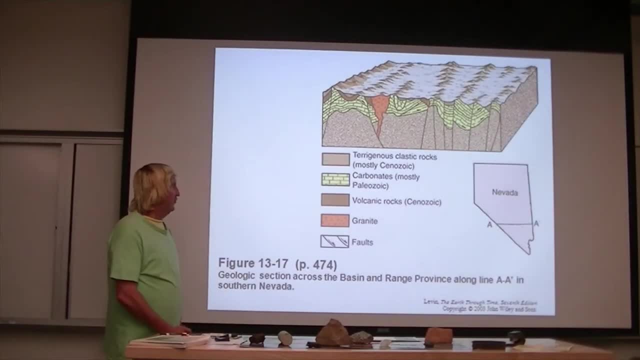 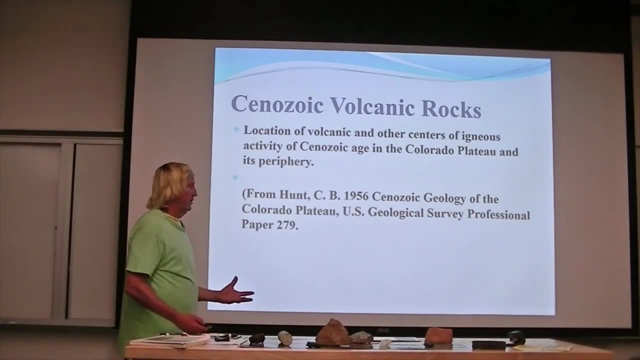 Nevada, California, the Washington State. geology is very difficult to understand. So Jared's a Cenozoic. because of the fact that we're now stretching the continent, we saw a lot of volcanic rocks forming, Even in the Grand Canyon, a lava flow. 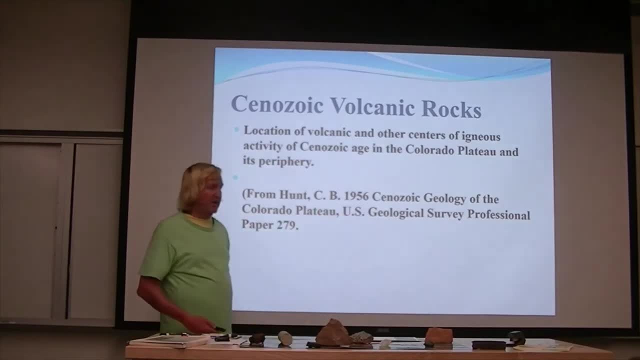 basically at one time flowed across the Grand Canyon and dammed the Colorado River. The Colorado River eventually cut down through those sediments and today those volcanic rocks are there and it forms one of the steepest lava flows and it also results in a very rapid. 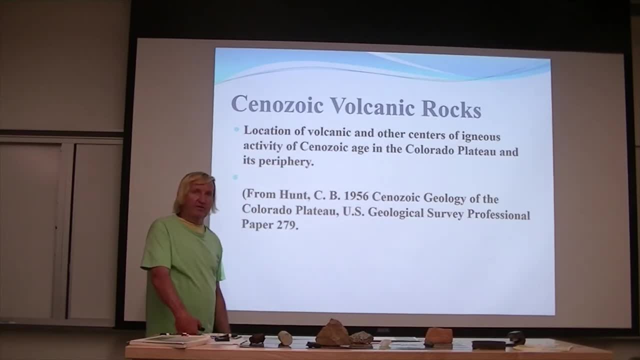 decrease in the elevation of the Colorado River. In fact it forms a rapid called lava, And it's the most dramatic. so if you ever do a rafting trip down the Colorado River, that lava is actually almost- I don't call it a rapid, I almost call it a waterfall. 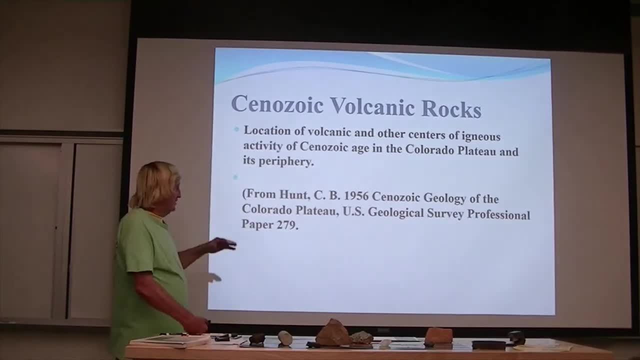 It's just amazing how steep that thing is, And that's because that lava flowed across that and then dammed the Colorado River filled up with sediment and then the Colorado River eventually breached the lava flow, cut through the lava flow, cut through all the sediments and went back down. 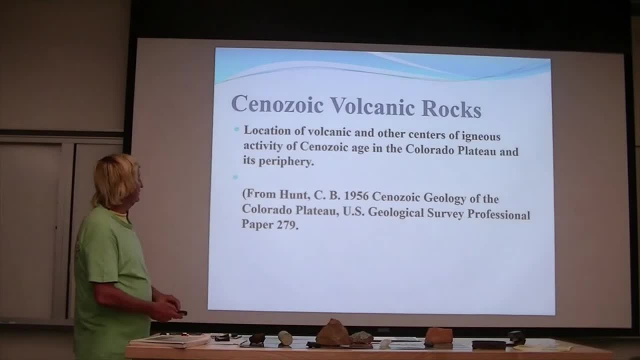 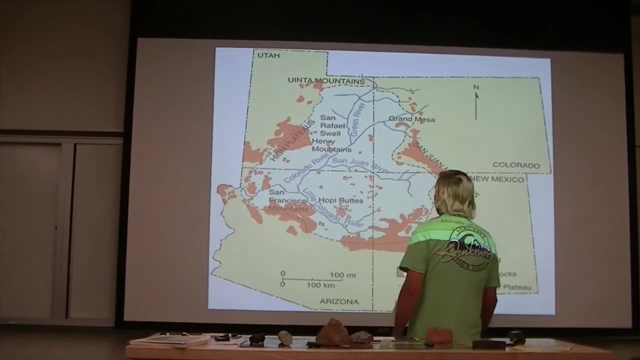 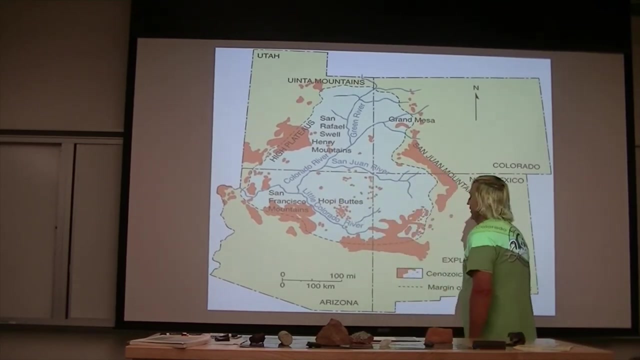 carving down to the Colorado River, again to the Grand Canyon. So here is our Colorado River, which is cutting down through the Colorado Plateau. The San Juan River, which flows out of New Mexico, is a tributary to the Colorado River, The Little Colorado River, a really interesting river. 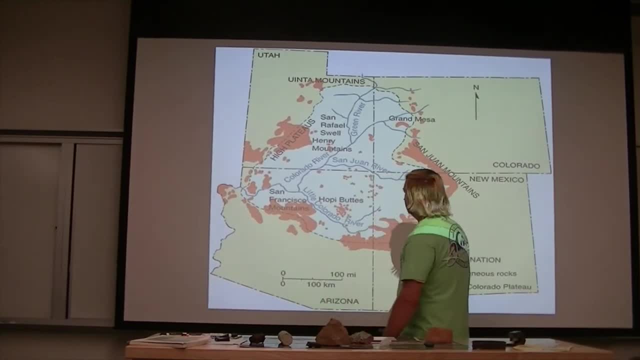 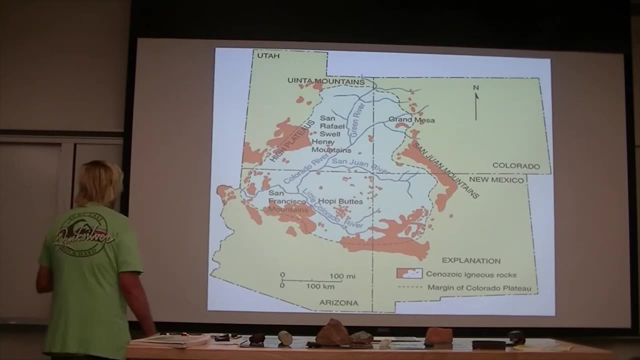 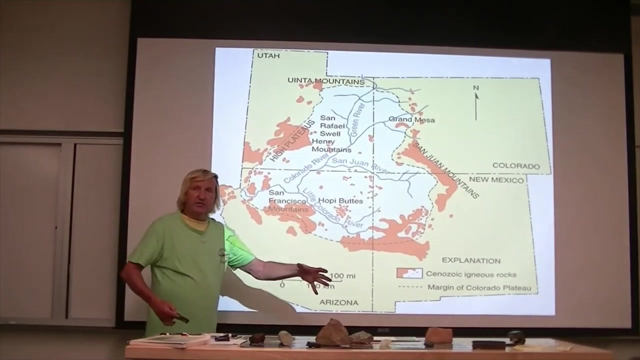 flows in turquoise color because of copper. All these rivers converge into the Colorado River And then the Colorado River has something very unique. At one time it flowed to the west, But because of this potential tectonics and these bases being formed, the Colorado River took a 90 degree turn. 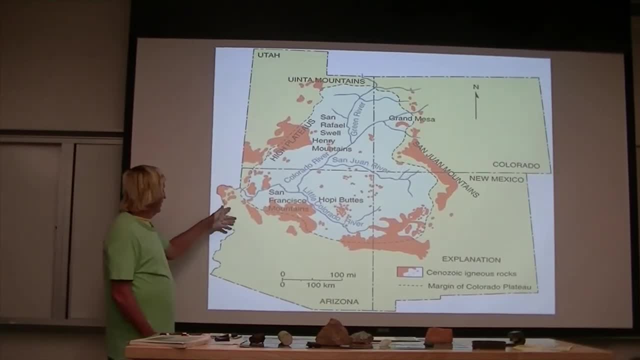 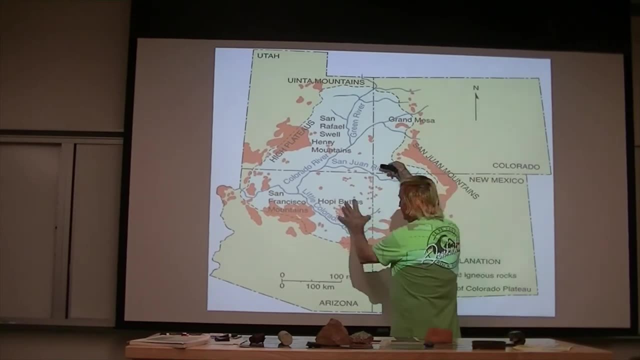 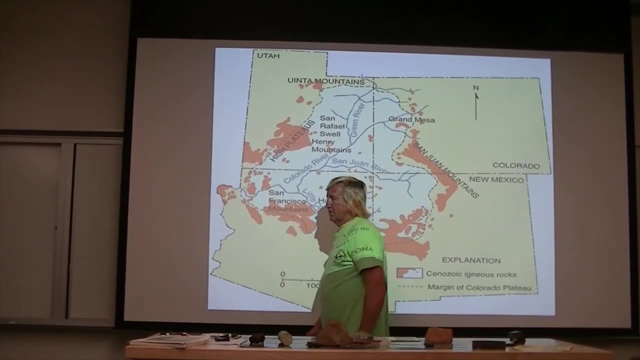 and flowed due south along the Arizona California border. So the Colorado River and its whole system is draining from east to west and then all of a sudden makes a dramatic turn and turns due south. And this is due to extensional tectonics, which really started. 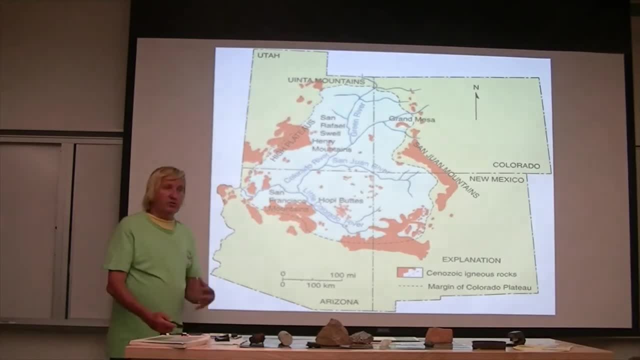 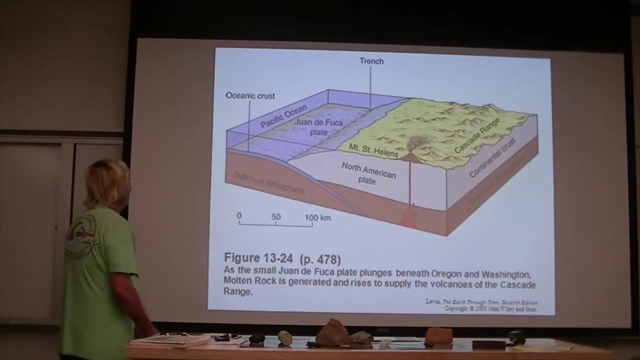 when we started to extend the continent and stretch it, which starts right around 22 to 25 million years ago, And this had a dramatic directional change in the Colorado River. So because of subduction to the north of us, sir, we still have a remnant. 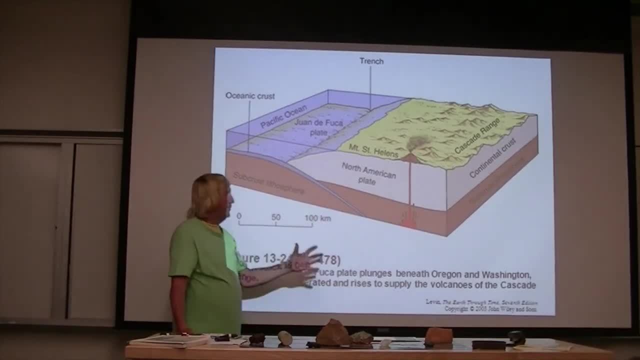 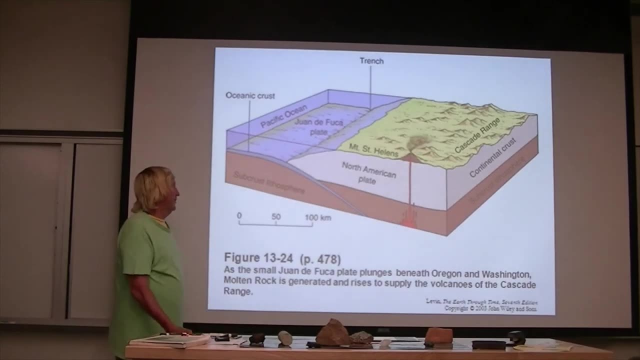 of the Farallon Plate, which we call the Juan de Fuca Plate. It's just ducking underneath what is today Northern California, Oregon and Washington And, as that Farallon Plate seduces that remnant of it which is called the Juan de Fuca Plate, 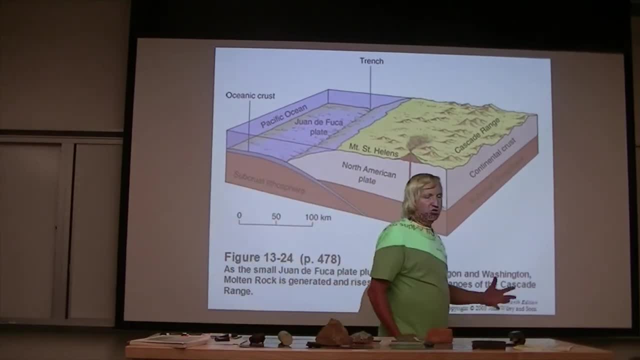 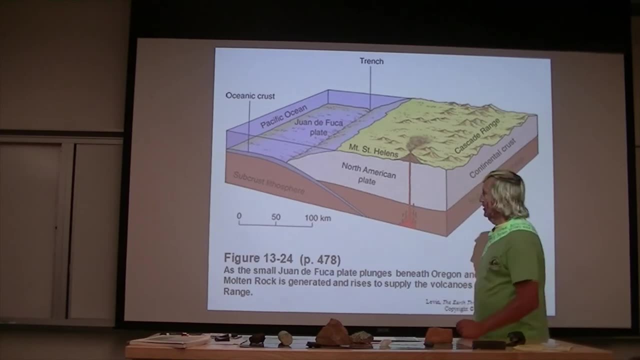 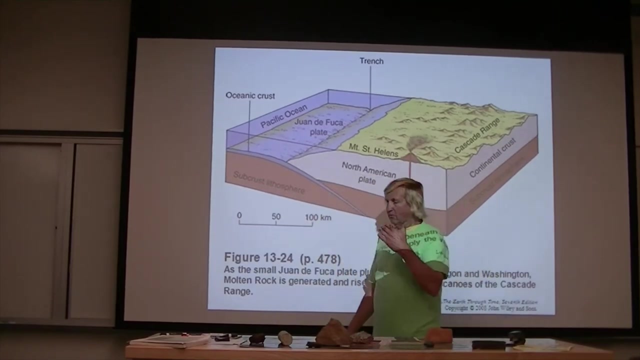 it's melting and it's feeding. today, a chain of volcanoes called the Cascades. Mount St Helens is a part of that chain of volcanoes. This is what California looked like. So if you go up to British Columbia, you go to Oregon. 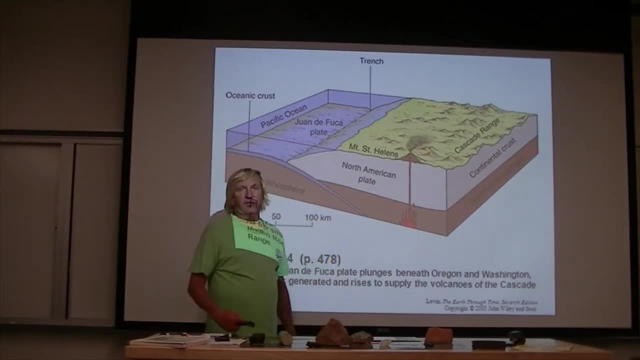 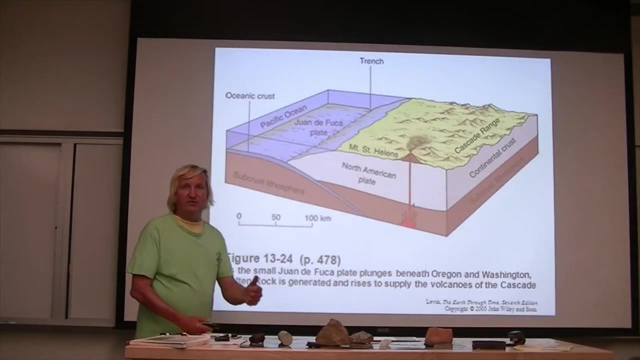 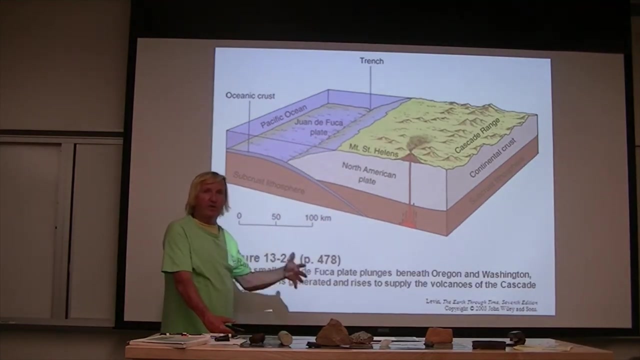 Washington, Northern California. This is what Southern California looked like during the Mesozoic. So if you want to see what Southern California looked like during the Jurassic and the Cretaceous, you go up to Northern California, Oregon and Washington Eventually. what's going to happen is that Oregon, Washington, Northern California are going to override that spreading center that's off the coast, and the San Andreas Fault- It's going to continue to move north. So the San Andreas Fault, which started in Los Angeles. has spread to the south. It has taken the Baja Peninsula away from Mexico. Now the San Andreas Fault is going to move to the north. It's going to consume Northern California, go through Oregon into Washington and then eventually up into British Columbia. 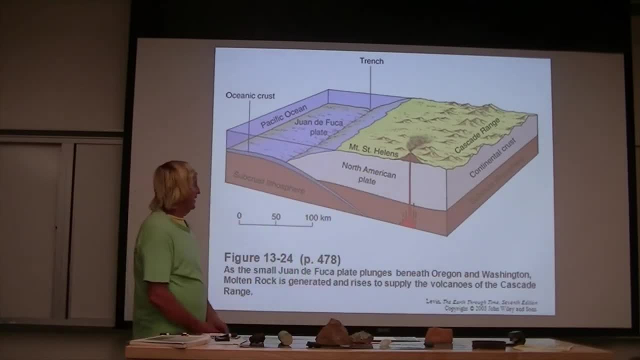 And eventually all the way up to Alaska. And the San Andreas Fault is going to move towards the east And eventually it's going to go to Nevada And then who knows, from there. So this is basically kind of a showing the California Fairline Plate. 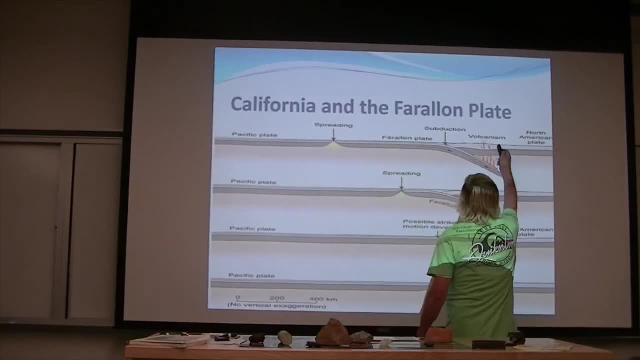 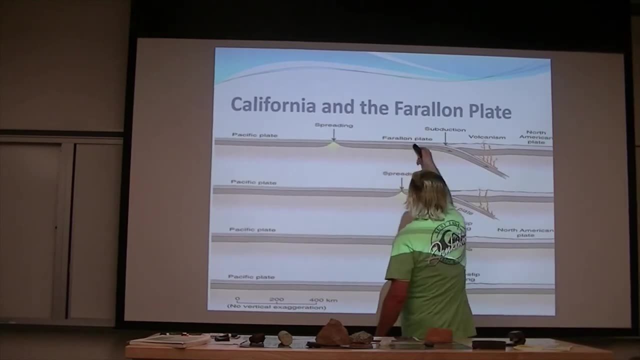 Here's the spreading center. Here's the North American continent. Here's that Fairline Plate. This diagram doesn't show all the microcontinents on it, So picture a bunch of microcontinents on there. Boom, boom, boom boom. 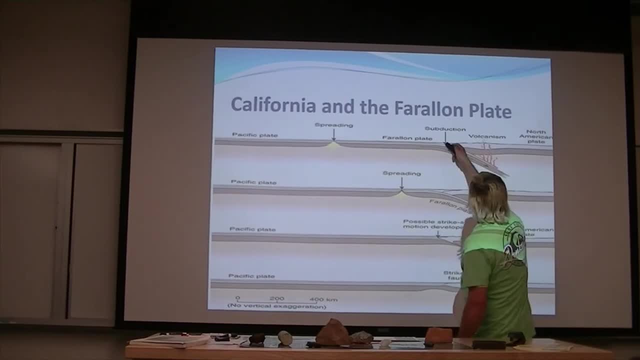 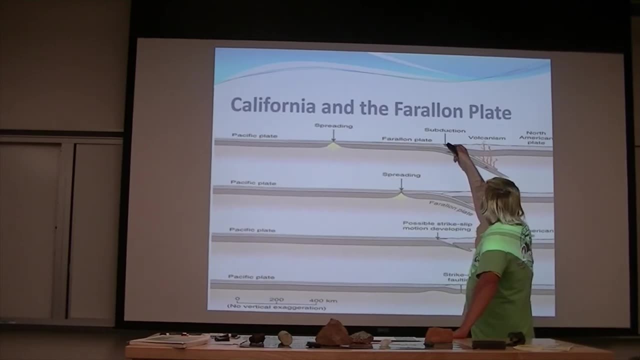 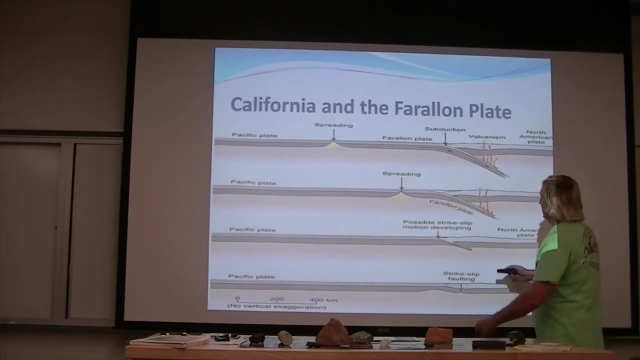 And they're all going to get conveyor belts pushed on. So this would actually be about the Nevada- Utah border. And then, as the North American continent moves north, the Fairline Plate gets consumed. So here the Fairline Plate is big, Here the Fairline Plate is smaller. 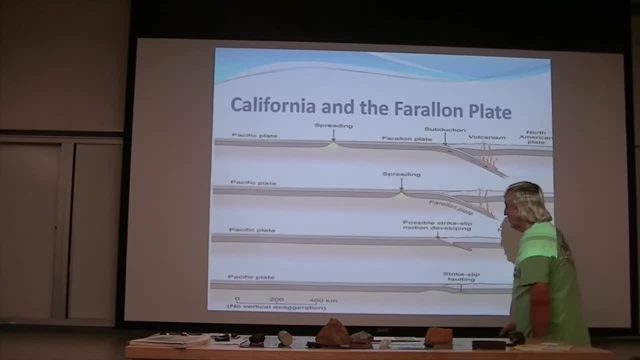 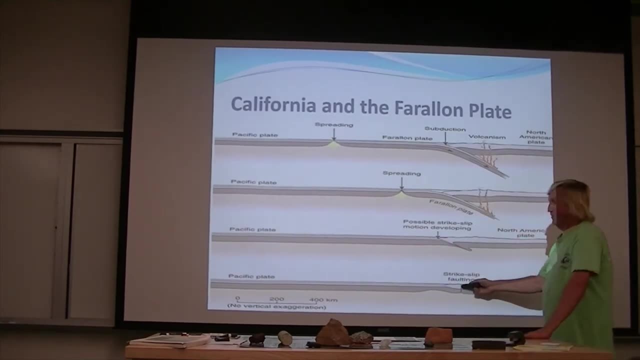 And then here, the Fairline Plate is very small. This would probably look like maybe 30 million years ago. And then, right when the North American continent overrides that spreading center, right there, that's when the San Andreas Fault is born. And, ironically, they think this occurred pretty close to where LA is. now They think of the San Andreas Fault, they think of LA, And I guess that's for a good reason, because that's where the San Andreas Fault really originates, in the state of California. 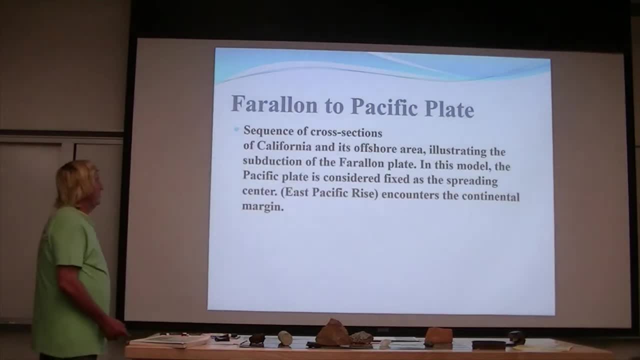 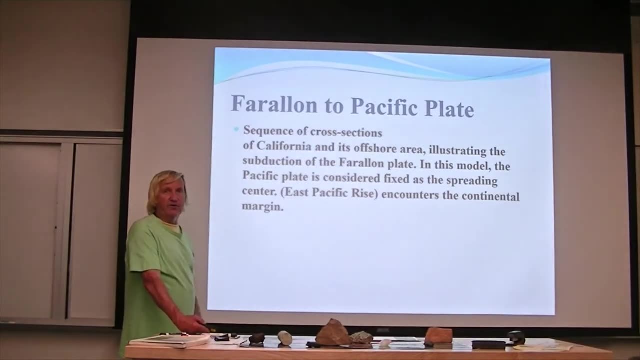 So the Fairline Plate to the Pacific Plate. The Fairline Plate, where is it today? Well, basically, it's underneath Nevada and Utah and Arizona, And it's still melting. The Fairline Plate. as it melts, magma comes up Out in the California desert there's a volcano called Amboy. It's right off of I-40.. That volcano erupted 10,000 years ago. There are cinder cones in SEMA, which is off of Interstate 15, between Baker, California and Las Vegas. 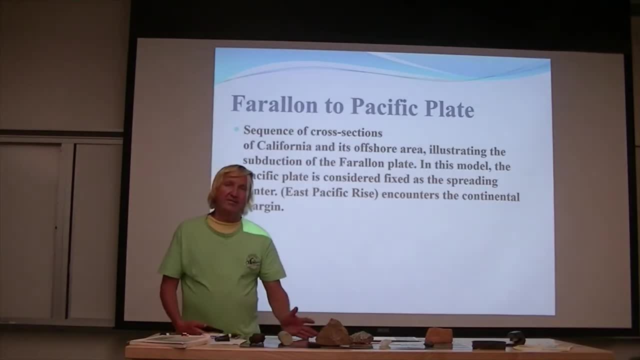 Actually closer to Baker, There's recent volcanoes on the east side of the Sierra Nevada Mountains, near Mammoth. All this is believed to be due to the result of the Fairline Plate melting, and then those magma bodies are then migrating up into the continent. 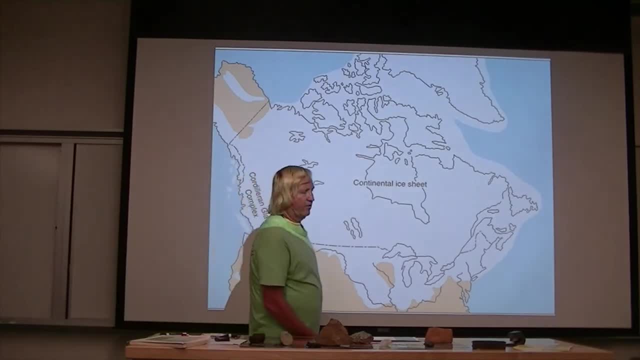 The most recent chapter and this is kind of an important one. so you have to realize we go in the Mesozoic from being tropical. so then we get into the latter part of the Cenozoic and for the first time, the North. 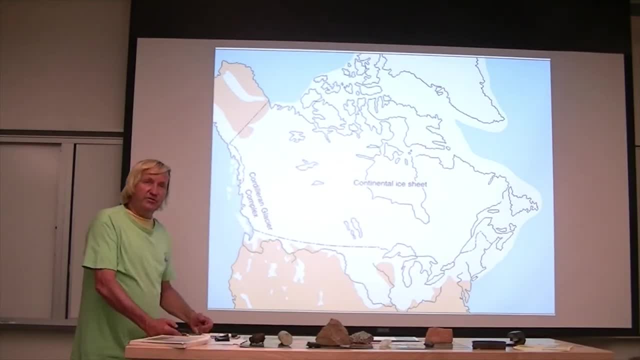 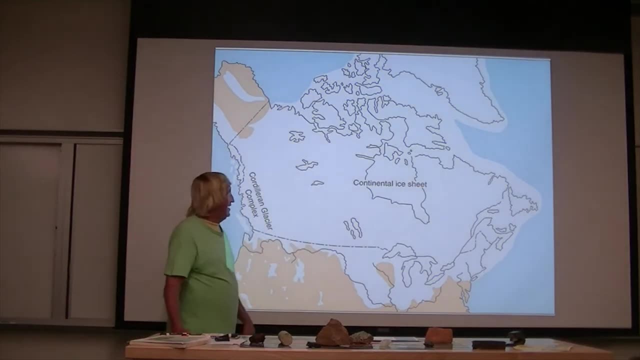 American continent sees glaciers, And so, starting up about 700,000 years ago, we see ice which originates in Canada, and that ice then moves to the south. Now remember what was going on in the Mesozoic in the mid part of the United States, The Sundance Sea. 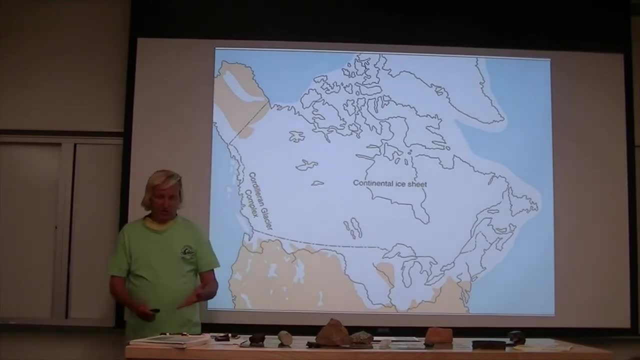 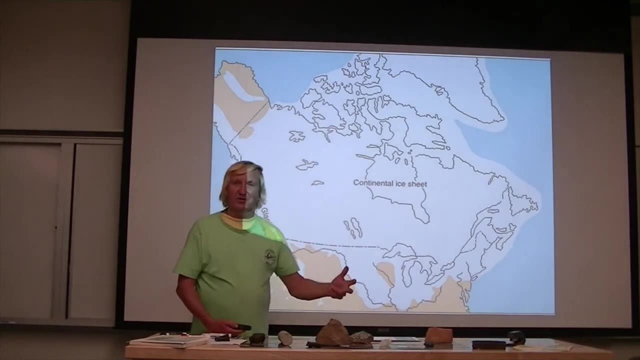 was there? What was the Sundance Sea, depositing Gypsum and salt? Gypsum and salt are not very good materials for farm soil, But we have great farm soil in the Midwest today, So we're going to talk about where that farm soil comes from. 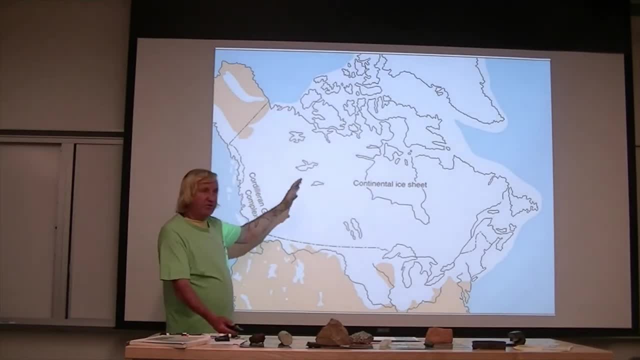 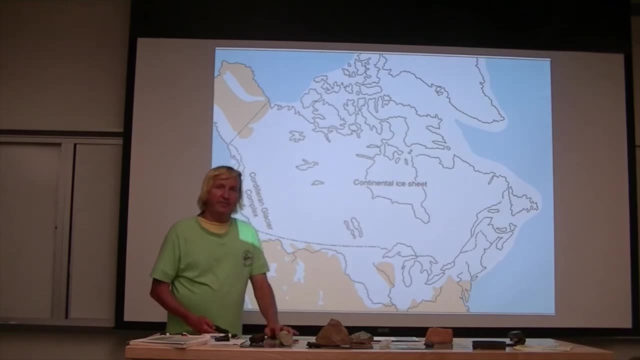 real, simply Up here in Canada. this is all granite. What's in granite? Minerals that contain elements like iron, magnesium, potassium. So what the glaciers did is they took this granitic rock and they moved it with it, They pulverized it, they ground it up. 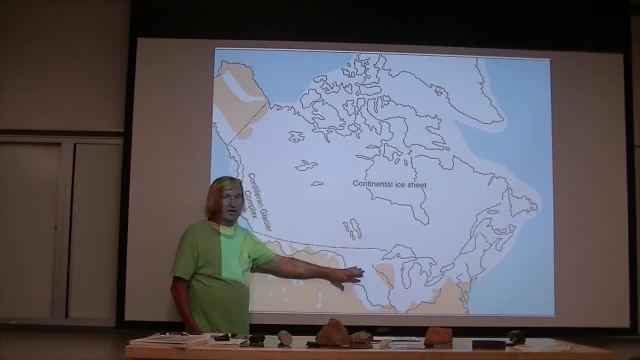 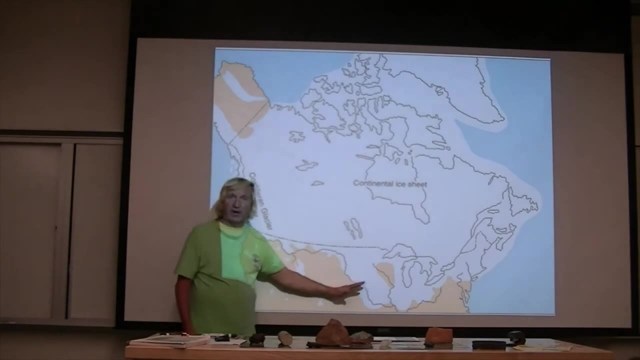 and they pushed it like a bunch of bulldozers, all this granite into the United States until it was a very inferior part of the United States- The Great Plains, Ohio, Nebraska, Kansas, Oklahoma- And when the glaciers retreated they left all that crushed rock. 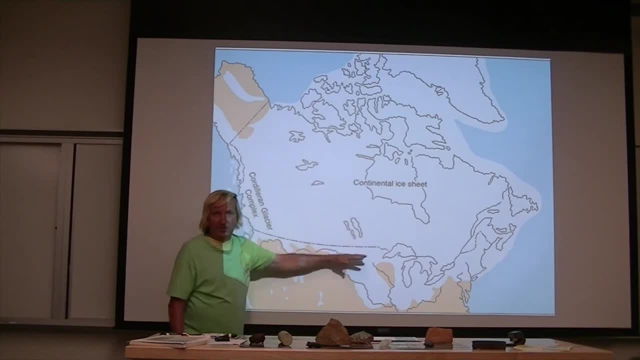 behind The glaciers retreated. Another glaciation, same thing: Bring more rock. climate warms, glaciers retreat. Climate cools again, glaciers advance. So there are four major glaciations And a minor glaciation, and we name these glaciations after states. 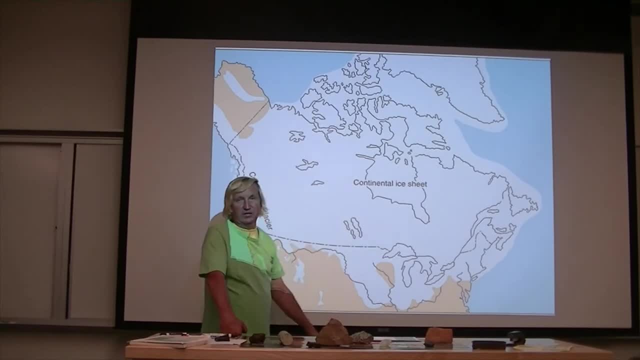 So the last glaciation was the Wisconsin, because that glaciation covered the entire state of Wisconsin. The most severe glaciation we encountered was that the western United States encountered was the Hansian glaciation. That's where the glaciers extended as far south as Kansas. 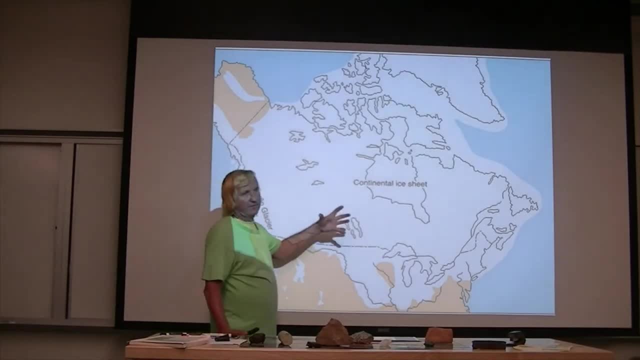 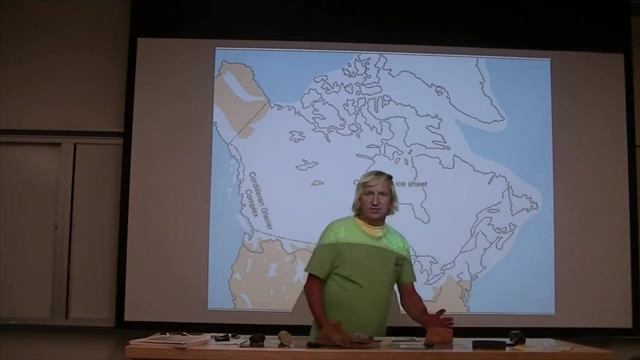 And every time they did, they brought with it granite which was crushed into fine-grained material, and that's why in the midwest United States, we have the corn belt, the wheat belt. So isn't it amazing how geology influences plants? So geology. 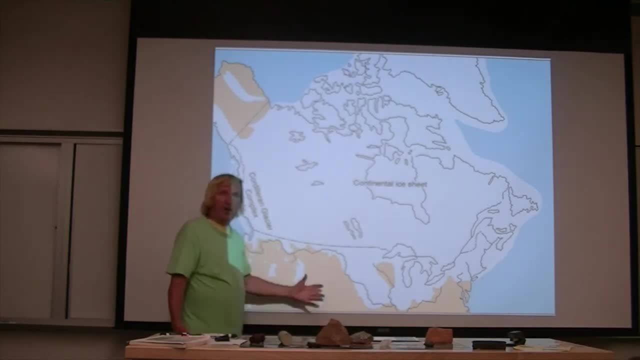 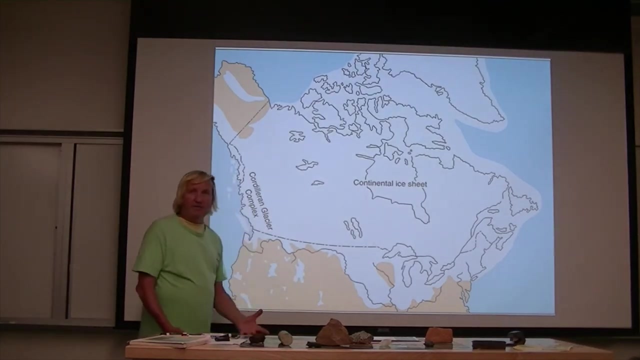 makes the soil for the plants. The plants are then going to respond to that soil, and then who's going to respond to the plants? The animals. So this is where plate tectonics and geology, climate, biology- it all is interrelated. 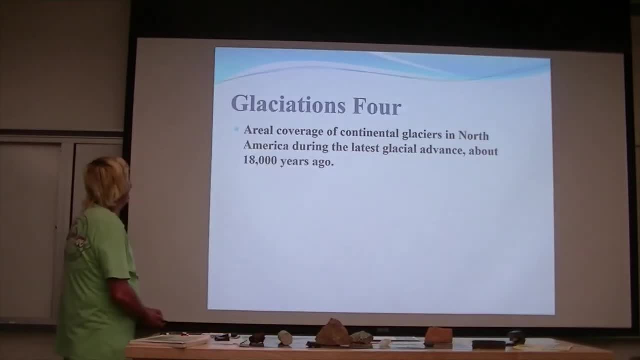 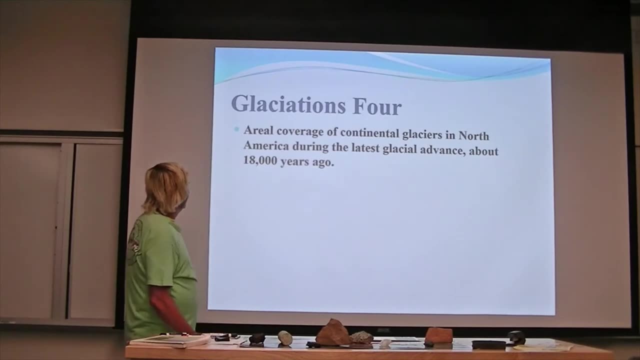 It's all tied together It's pretty neat. So there are four glaciations and a very minor one in between. So glaciers covered a good part of the North American continent about 18,000 years ago and about 12,800 years ago. 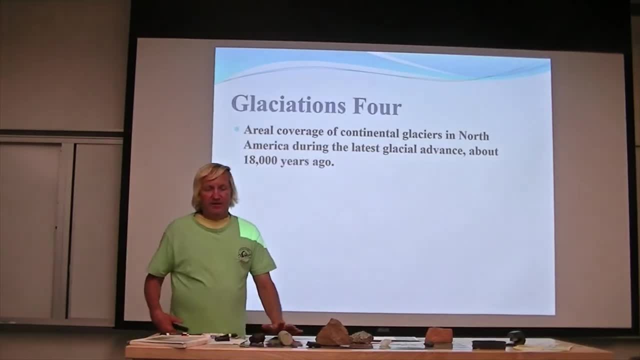 climate dramatically warmed and then it cooled real quickly and then we think that that cool down was because a meteor impacted today was the Indian Ocean. this wiped out the woolly mammoth. Now a lot of people have written that the woolly mammoths were hunted to extinction. 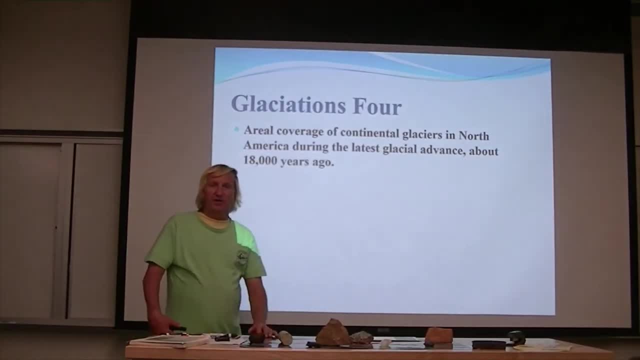 by the nasty humans, and that's because archaeologists actually found a site in Northern Europe where a woolly mammoth was found with a obsidian point in it. So because of that, fine, right away they jumped on the speculation place and bandwagon says: 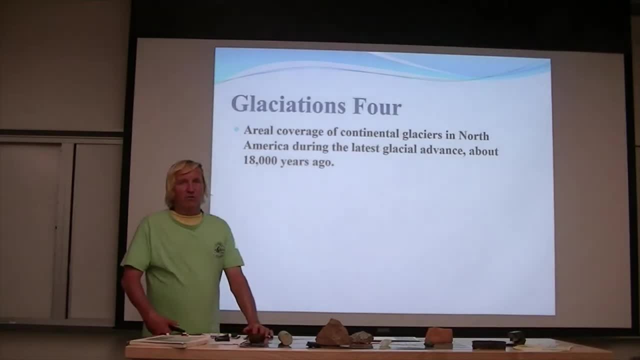 humans. humans actually caused the death of the woolly mammoth because we over hunted it, And it makes sense. but what probably makes more sense is that the woolly mammoth demise was met 12,800 years ago. And why 12,800 years ago? 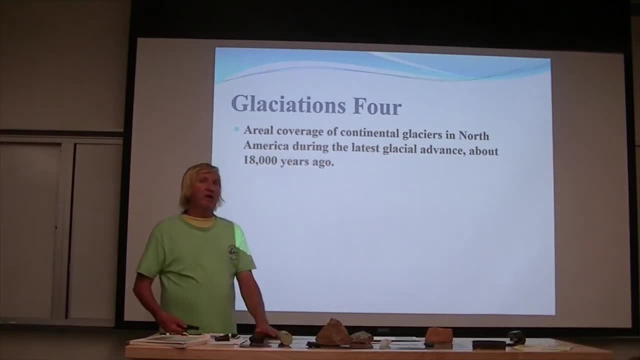 That's when a meteor hits Earth and we basically have pretty good evidence of that impact. We do have some iridium and we have some carbon 13 anomalies and that would suggest- and that happens to coincide with the woolly mammoth, So that kind of cooled Earth down again. 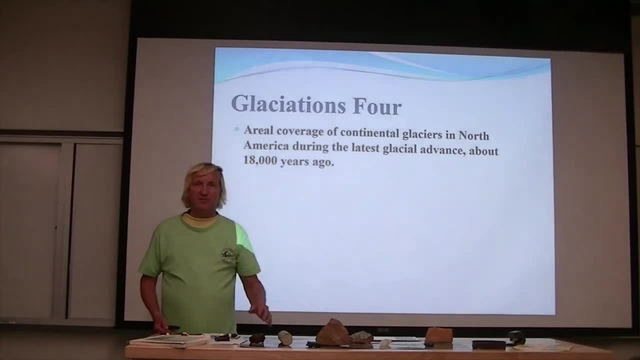 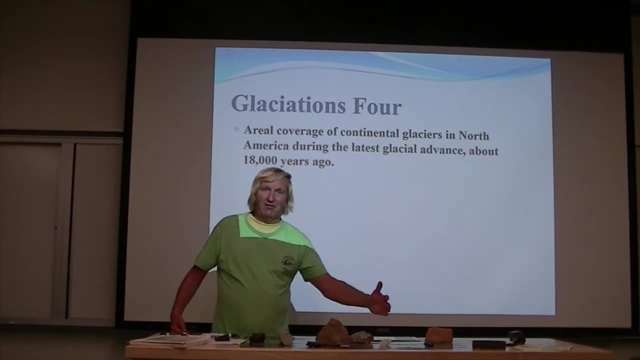 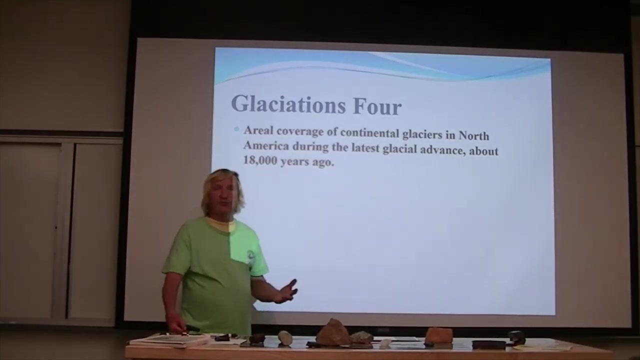 for a while, because of all the particulate matter was injected in the atmosphere and then Earth warmed. so from about 12,700 years ago to now, the Earth has been basically warming, although within that warming there's been some cooling periods during the medieval times. 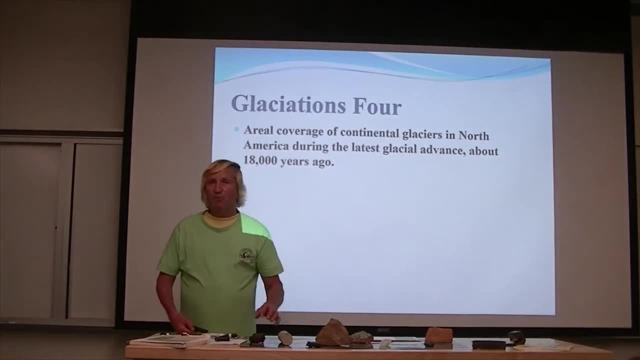 there was a cool down. prior to that, there was a big warm up. so a thousand years ago Earth was warmer than it is today. Greenland was actually green. the Vikings discovered North America because they were able to sail across the Greenland, because the climate was warmer. So there's been 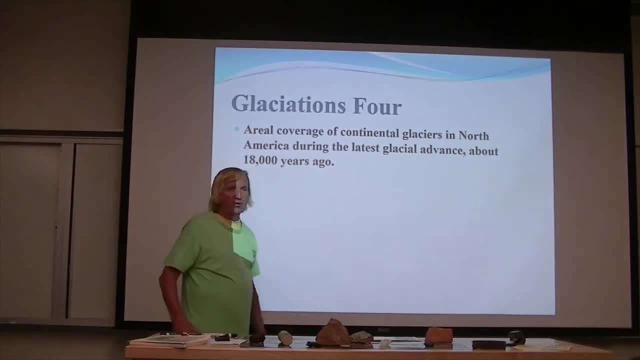 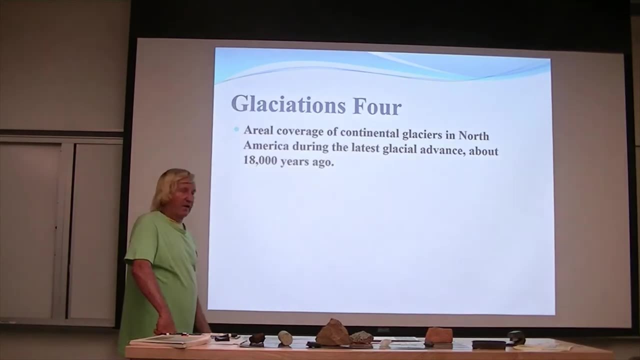 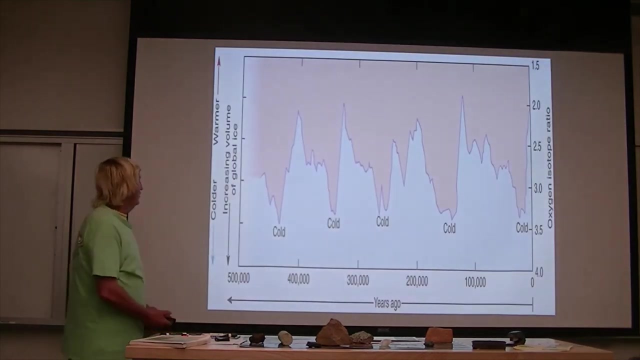 some fluctuations in climate, but for the most part it's been warming dramatically since about 12,000 years ago, and then there's some good arguments that suggest that humans are speeding that process up today. So this basically shows these glaciations: very cold climates. 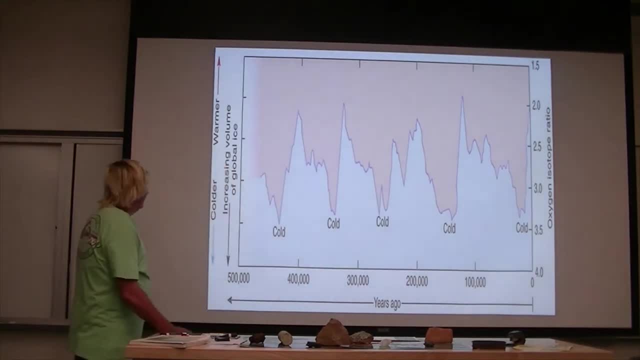 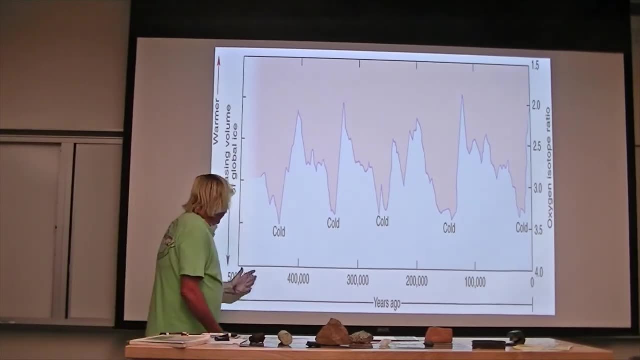 warm climates to cold climates and we have a really good record. this number is kind of outdated. now because of ice cores and because of good isotope analysis, we kind of push this back to about 650,000 years. we think that's when the first 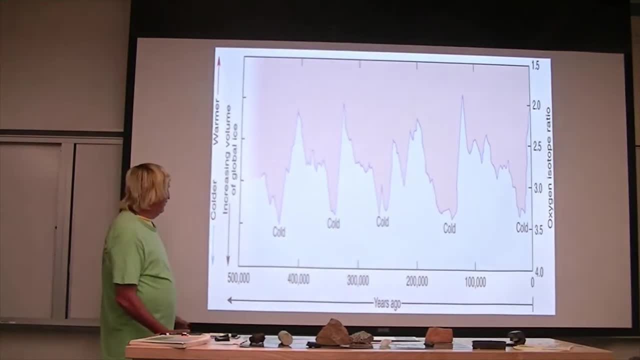 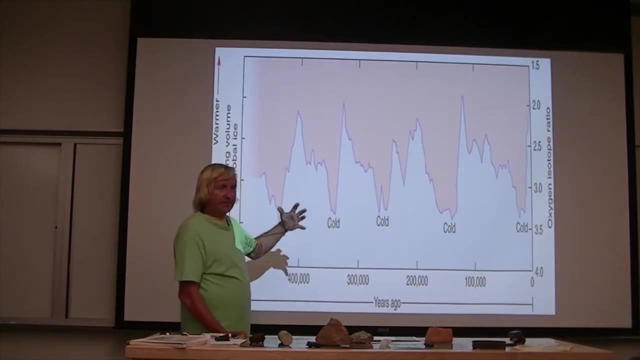 glacier hits about 650,000 years ago. so we hit very cold periods with lots of glaciers. Earth's warmed up again, glaciers retreated and then Earth cools down again and we've seen this cycle which we call periodicity and, on average, the northern hemisphere. 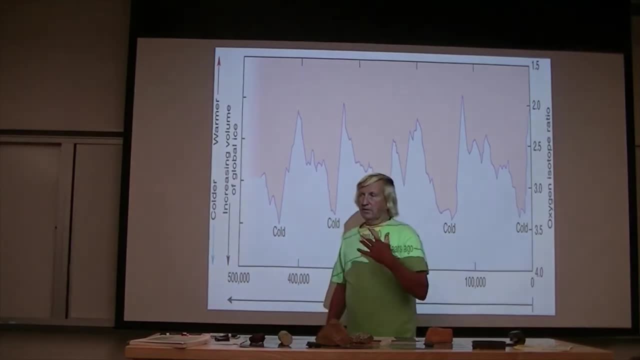 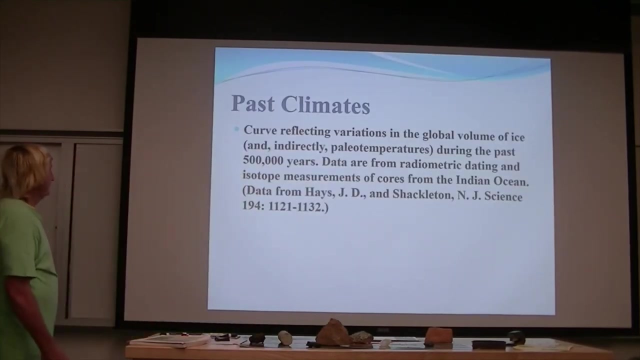 of the Earth- the United States, Russia- experiences a major glaciation on average every 100,000 years. so past climates. we know that because of isotopes, because isotopes of hydrogen and isotopes of oxygen, delta 18,, delta 16 ratios we can pretty much reconstruct. 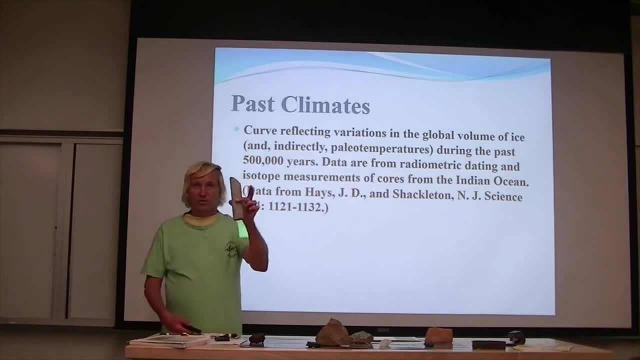 what past climates were like. so we can extract ice cores. so this obviously is not an ice core, but they look pretty similar a little bit wider. and within these ice cores there are bubbles that contain isotopes of hydrogen- delta 18 and delta 16- and we look at that ratio. 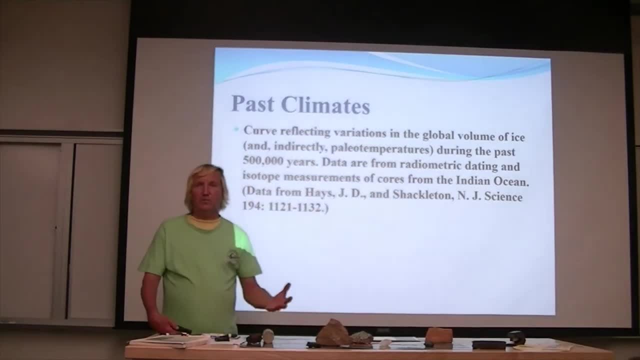 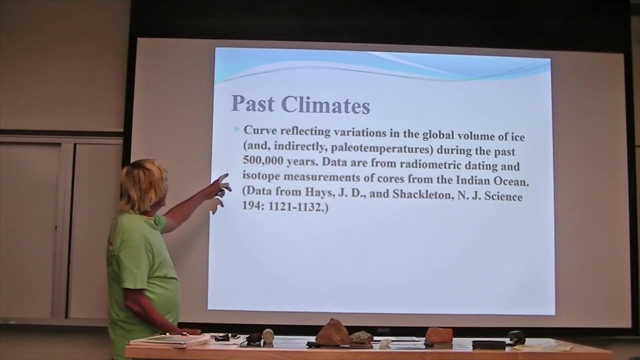 between the 18 and the 16 to determine if climates were warm or cold, and they're pretty reliable for reconstructing past environments and temperatures. so these curves reflecting global volume of ice and so paleo temperatures really during the past 650,000 years basically. 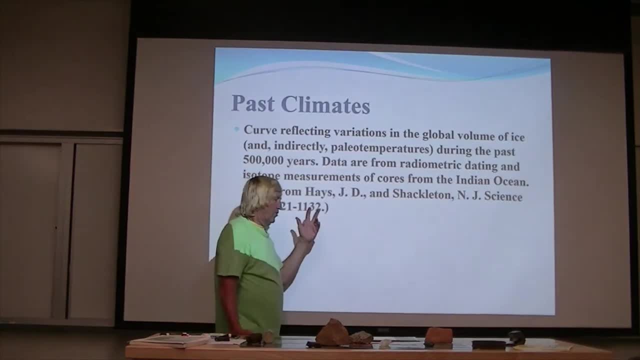 there are lots of isotopes that come from ice cores. those isotopes are the same, they match from ice cores that were taken from ocean sediments. we can also extract those isotopes from a fossil called foram and they all correlate very well and they're very good. 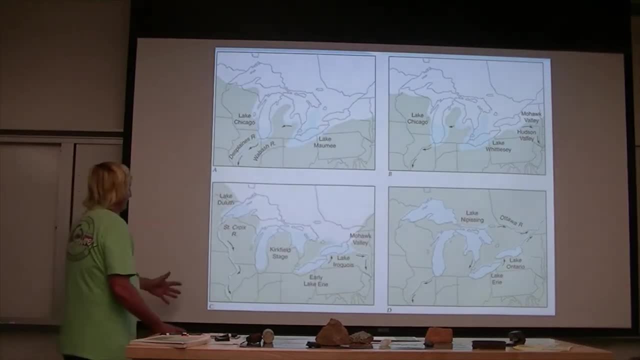 for climate reconstruction. so the great lakes were actually carved out by glaciers. so the last glaciation in Wisconsin actually carved out the great lakes, which completely changed the landscape. so here's a good example where these are all micro-environments along these lakes. so this is where geology, glaciers, 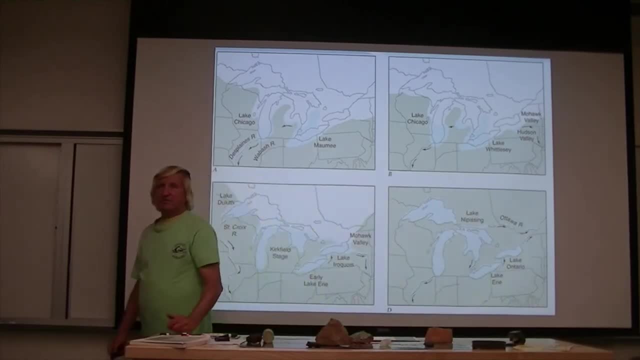 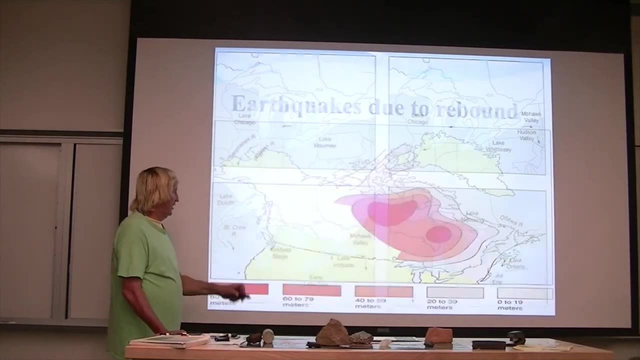 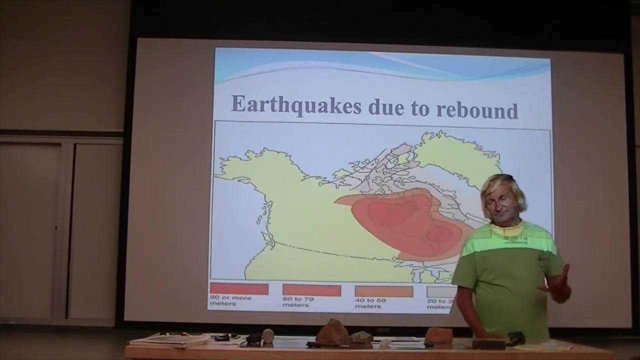 creates these great lakes. these great lakes then impact the climate and the climate then impacts the biology. so everything is certainly related. interesting thing is, the history of the United States is subject to earthquakes and they attribute these earthquakes because all this ice, volumes of ice- had compressed the rock. 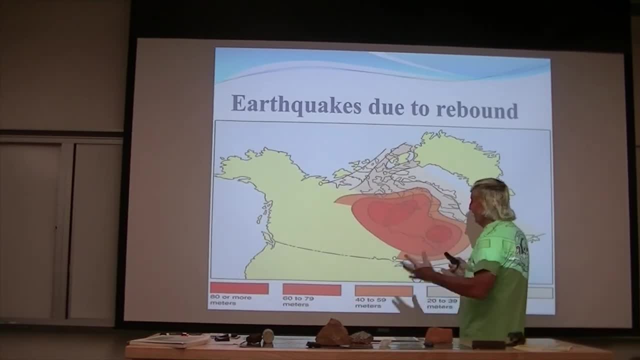 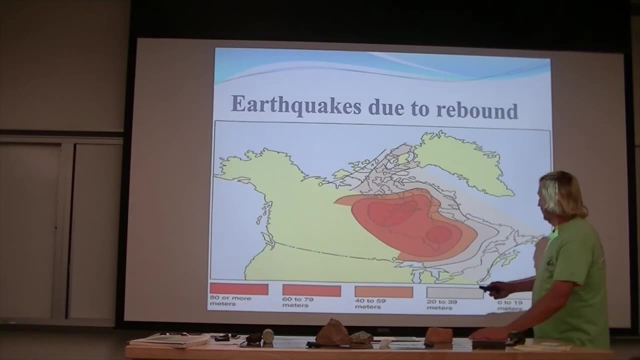 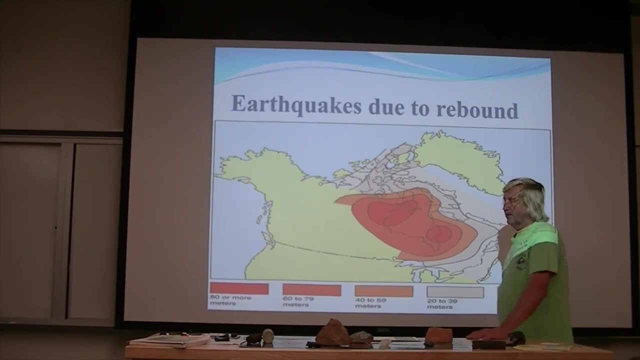 and then, when that ice melted, the rock began to rebound, and as it rebounded, it has earthquakes. so not too long ago, there was actually an earthquake in the Washington DC area, and that earthquake was attributed to the continental rebound, where the continental is actually rebounding because of all the 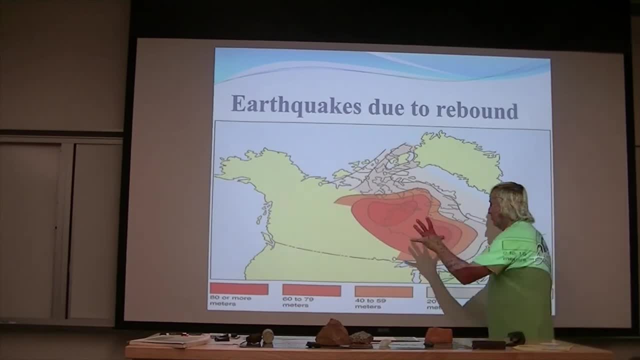 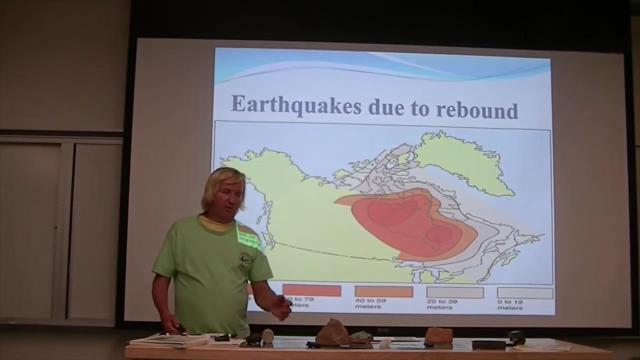 glacier's material actually compressed. so the most seismically active place in the world was not too far from us: Lake Mead National Recreation Area, which is just to the south of Las Vegas, Nevada, right on the Nevada-Arizona border. Hoover Dam was built there. 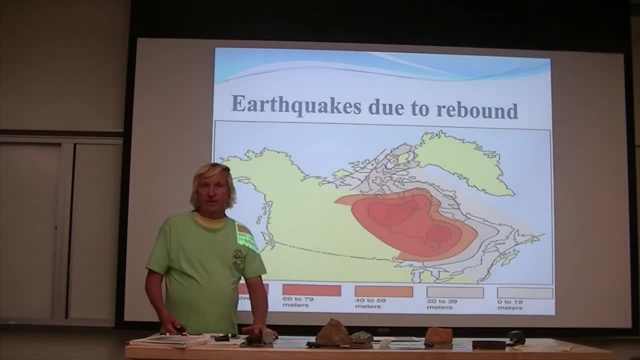 and as Hoover Dam filled up, it became this man-made lake in the world at that time, and that volume of water compressed the sediments so much that it created micro-earthquakes on a daily basis. so Boulder City, Nevada, which overlooks Lake Mead, 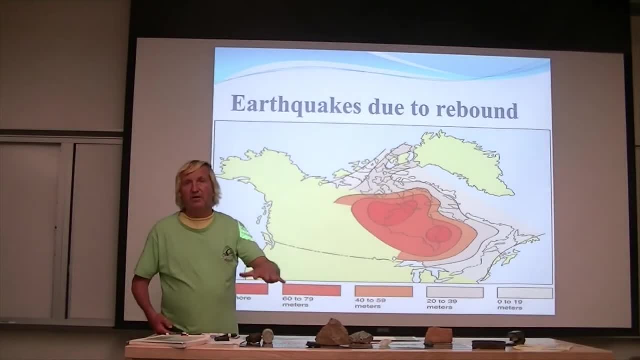 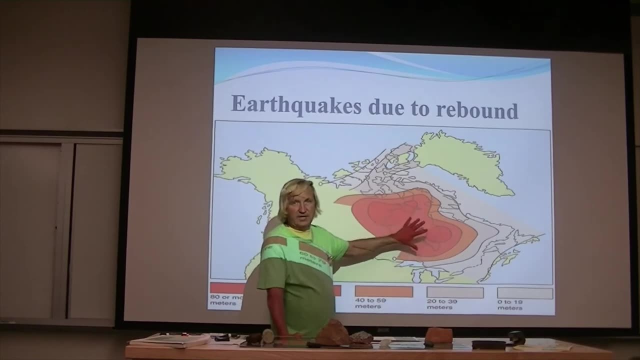 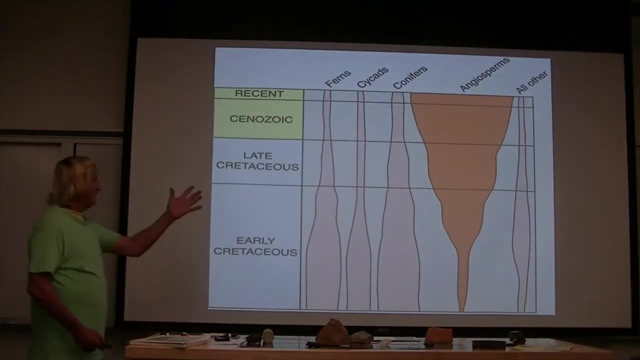 was the most seismically active place in the world because of the volume of water pushing down on the sediments. the same thing happens with ice, so ice compacts the sediments. when the ice melts those sediments and cause earthquakes. so this is actually a good diagram. 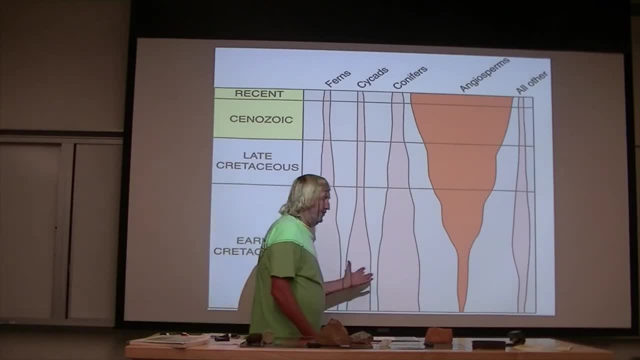 that shows the species that radiate out throughout the Cenozoic, and look at this. so here. so these are plants. so look at this. cyads, which are like a palm looking ferns, conifer trees. look at angiosperms. so angiosperms, the first. 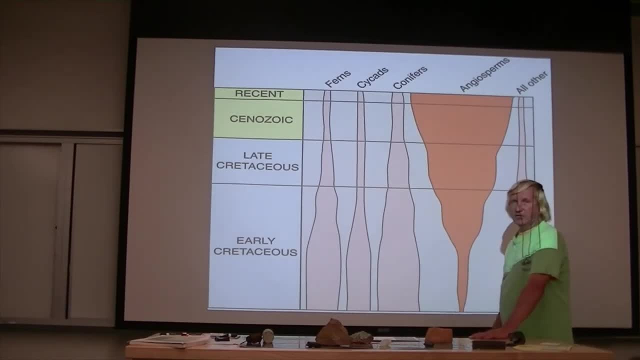 flowering plants were now found in the Jurassic. so the latest literature says that the first flowering plant that was discovered was in Jurassic age rocks. and people are trying to find that flowering plant in the Triassic and you know that's a big push in paleontology right now. 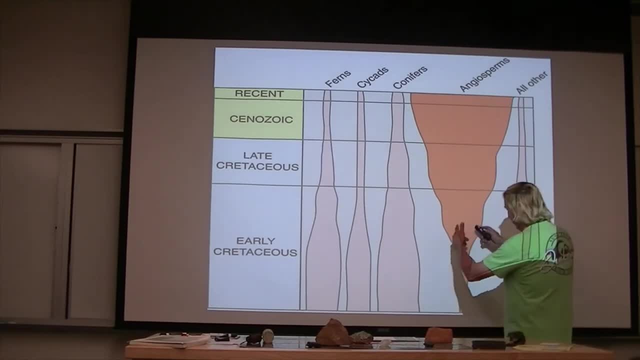 but look at the angiosperms. they don't do a whole lot here in the Mesozoic. they don't do a lot until they get into the Caucasus. and why? because this is the time when grasslands appear. so when the grasslands appear, 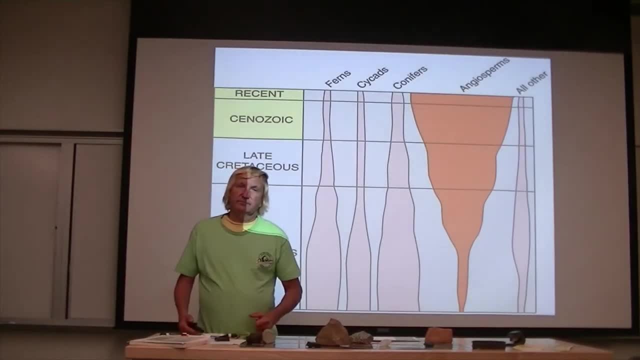 you're going to see the large grazing mammals: horse giraffes, elephants, zebras, those sorts of animals. what's going to follow? those animals are going to be the cats and the dogs. the dogs are interesting because a species of wolf is going to go back into the ocean. 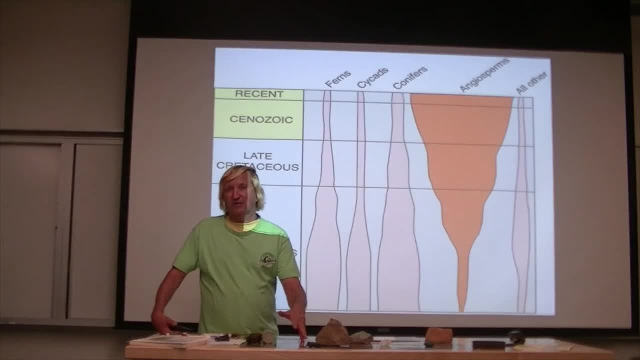 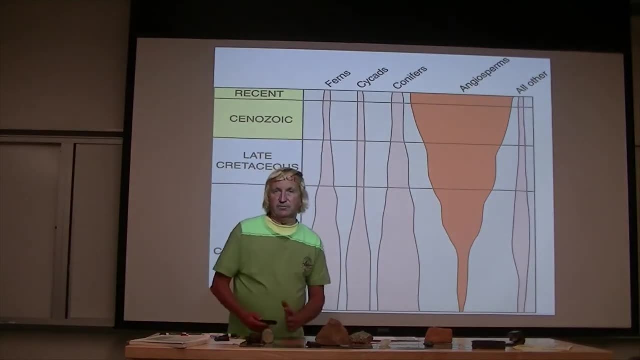 and become a whale. very interesting. there's a place in Morocco called the Valley of the Whales and they have like seven whale fossils- different species, and that shows this transgression. so this wolf is not like the wolf we see today. this wolf was kind of a long snouted wolf. 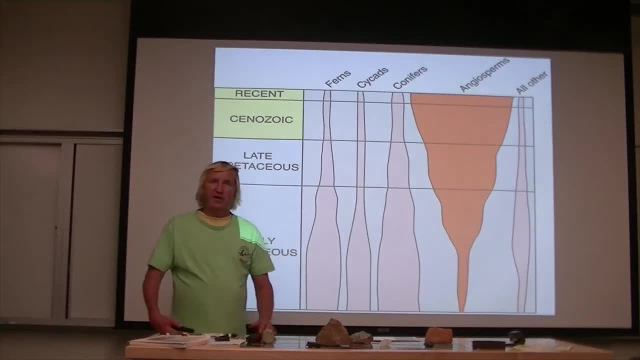 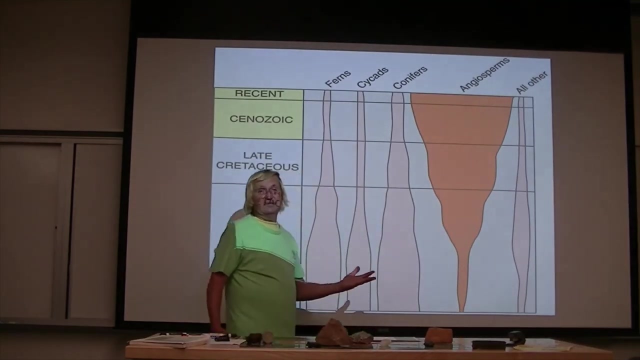 and it basically lived along the coastal environment and eventually migrated back into the oceans. so we have whales with shoulders that are that of a wolf, jaws and head very similar. imagine. ironically, one of the whales is going to come back out into the land to form a hippopotamus. 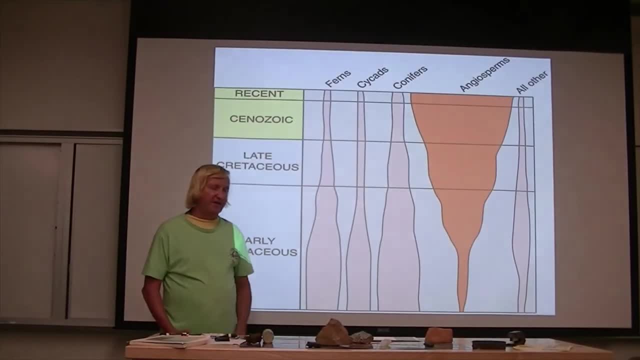 so hippos came from whales, whales came from dogs. so it's interesting that we learned that during the Devonian that fish, those five species of fish kind of evolved into land tetrapods and those land tetrapods are going to form the reptiles and eventually the mammals. 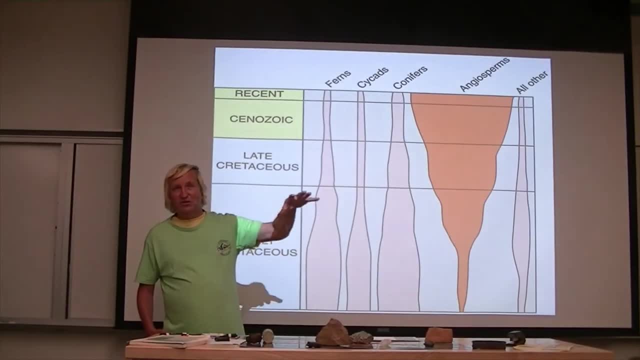 and then the dinosaurs, and we go through all that huge evolutionary progress and one of those four legged tetrapods, a wolf, is going to go back in the water, basically become a whale, and then that species of whale is going to come back out of the water. 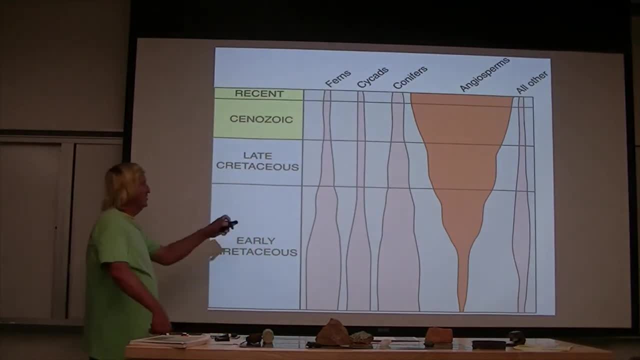 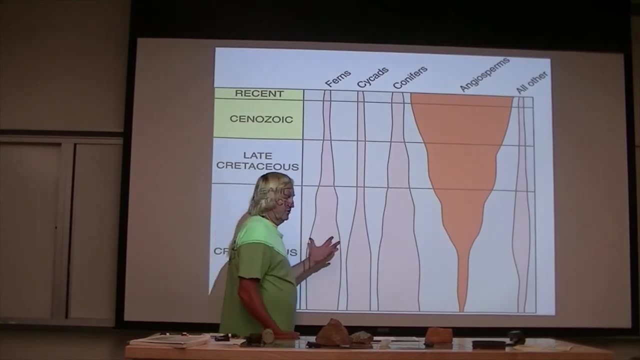 to form a hippopotamus. so it's kind of interesting how that worked. but angiosperm is the most prominent plant of all. so I think the two big events of the Cenozoic, actually probably three: diversification of climate, because the continents drift into more. 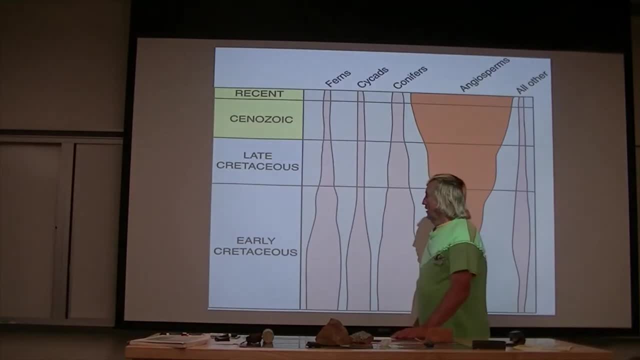 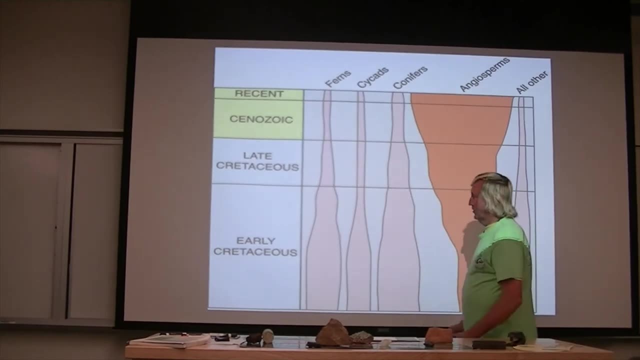 southern latitudes and more southern latitudes, temperature swings, so because of that, continents drifting, temperature and environmental conditions become very diverse, a lot of diversity with respect to climate, and the species that seem to take advantage of that are angiosperms, because you find flying plants just about everywhere. 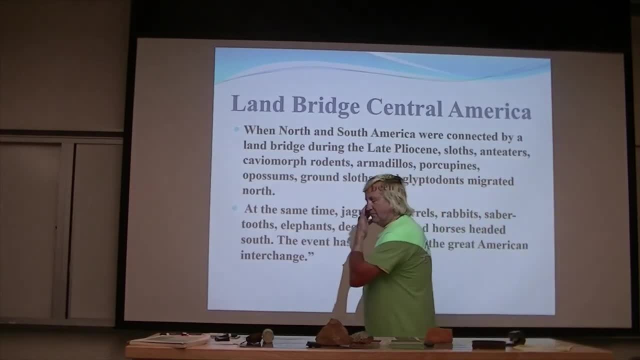 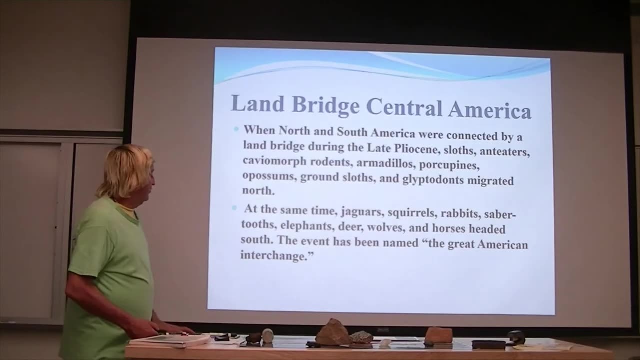 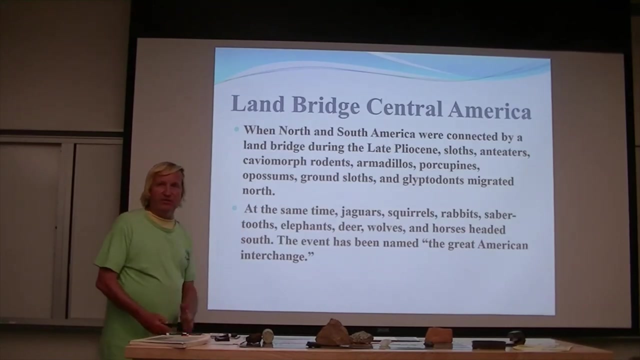 so a land bridge. so most of South America and North America have been separated for the longest time. they've always been separated and it wasn't really until recent that a lava flow occurs and formed a land bridge. Central America was then connected with South America and when that land bridge was formed, 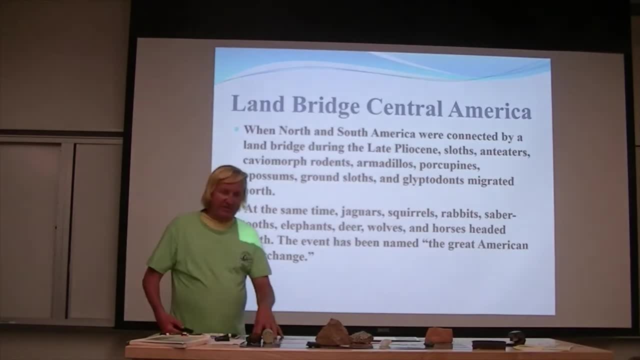 we had a great interchange, so species that lived in South America used that land bridge to migrate into North America. one of those most prominent is the armadillo, and armadillos are probably the most successful of all the species that came across the land bridge and then species that lived in Central America. and North America migrated south into South America. so when North America and South America were connected by a land bridge during the late Pliocene, sloths, anteaters, carnivorous rodents, armadillos, porcupines and all sorts of ground sloths- this is supposed to be possums. 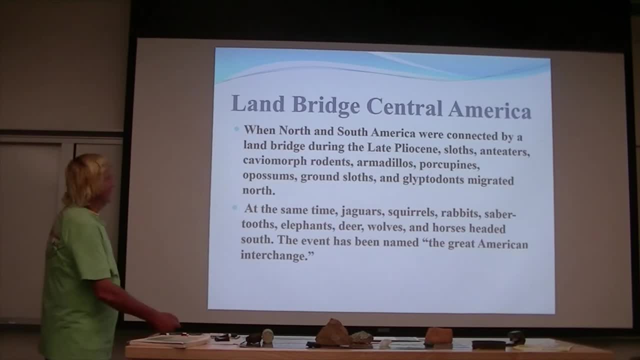 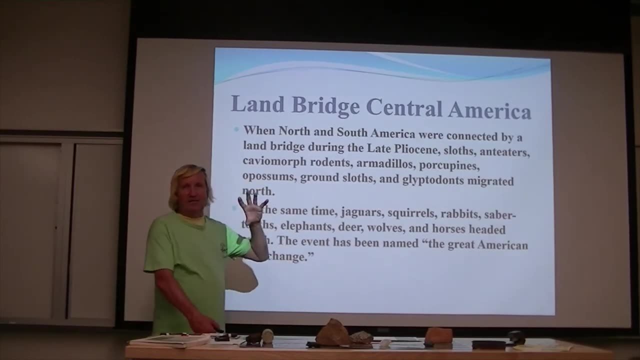 so, yeah, not little possums sounds like an octopus possum right. when I say this, it gives me that little warning that I'm moving along to the school computer and it's like a more updated Microsoft and some fonts get changed. I think this is what happens. 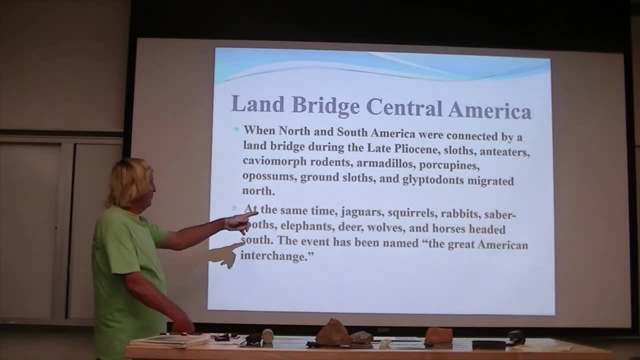 also ground sloths migrated north at the same time- jaguars, squirrels, rabbits. so squirrels are on campus. we can blame on South America. elephants, deers, horses. they headed south. this is called the Great American Interchange. so armadillos went north. 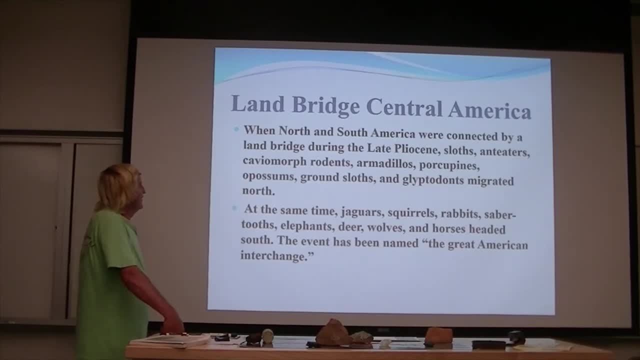 I got that backwards. so on campus we have actually a brown squirrel, which is not native. really, California has a gray squirrel, which is a native squirrel. the ones we see on campus here are the red squirrels. they're not native. so things have really gotten mixed up here. 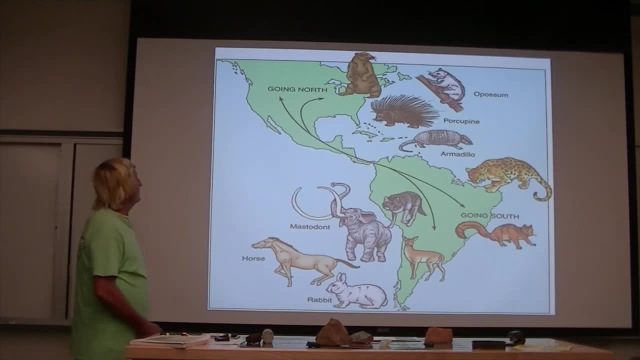 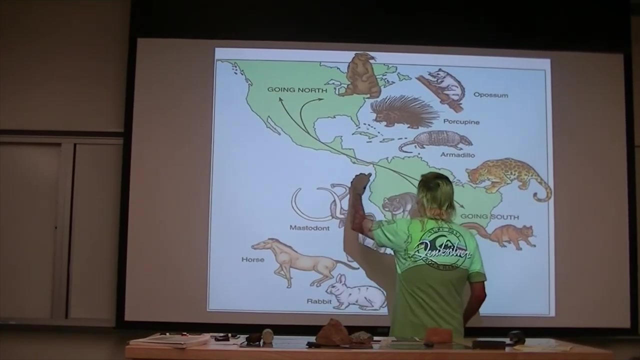 with the species. so this kind of shows. you know, people going north, people going south, and it's all because of the lava flow here. so this is actually where the Panama Canal is. Panama Canal, basically, is a seaway, an artificial seaway that allows ships instead of going all around South America. 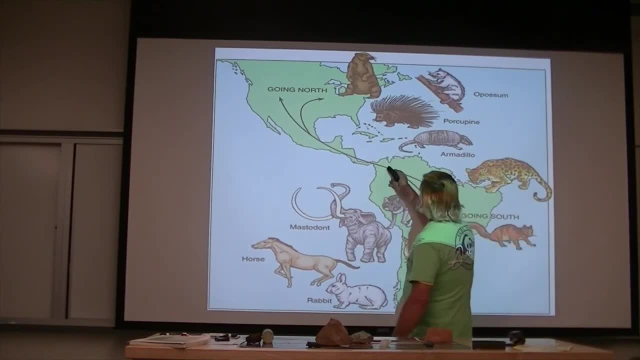 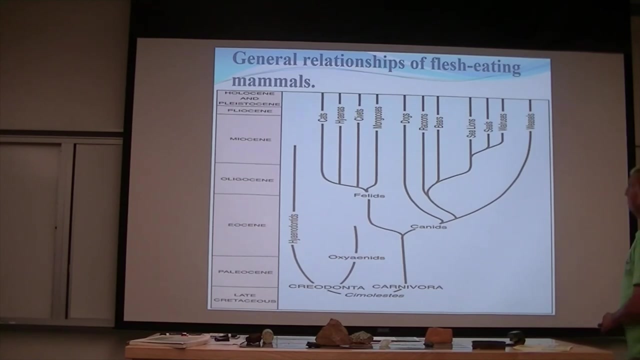 to go through the canal, and this land bridge here was actually formed by a series of volcanoes, and these canyons are actually connected to the point that allow these animals to do this Great American Interchange. so this is kind of a neat diagram right here. 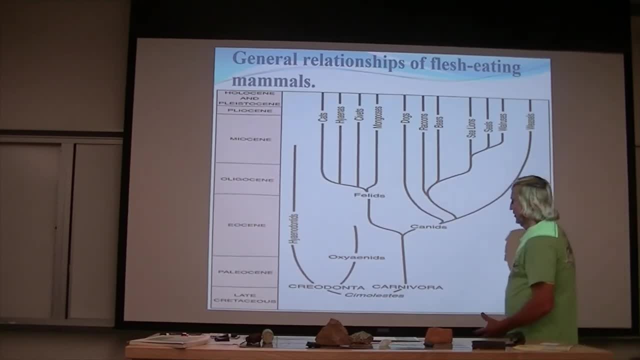 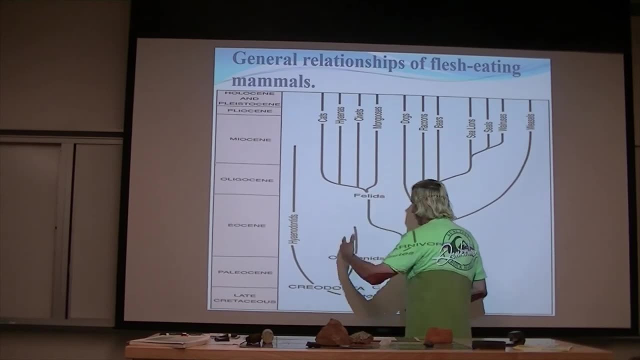 this shows. you know these splits. so we talked about this in the early Paleozoic with plants, and how plants split from ferns and hornworms and all that into vascular and non-vascular plants and all these splits, and so this basically shows what goes on. 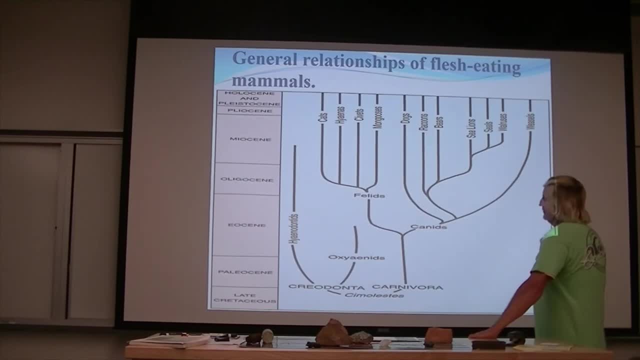 with the mammals, and the interesting thing is that there seems to be a huge radiating out of animals right at the end of the Eocene and into the Ligocene, and this is because climate really becomes more diverse at this time. so remember early part of the. 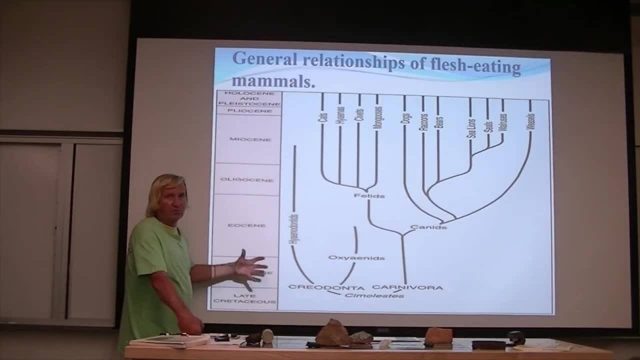 Paleozoic, 70 million years ago. Earth is still pretty warm. so as we go up through the scale we get into some warm periods, but then again, every now and then we'll see a warming period. so the Miocene was one of those where it kind of cools down the Ligocene. 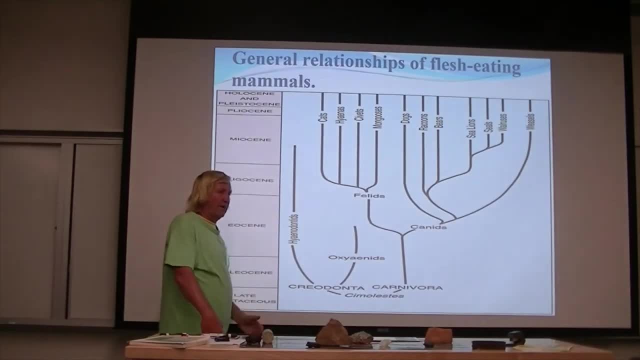 there's a huge warm up in the Miocene and the Pliocene. there's a warm up and then dramatic glacier start to form right at the Pliocene, into the Pleistocene, into the Glaciation. so the last glacier ended about 12,800 years ago. 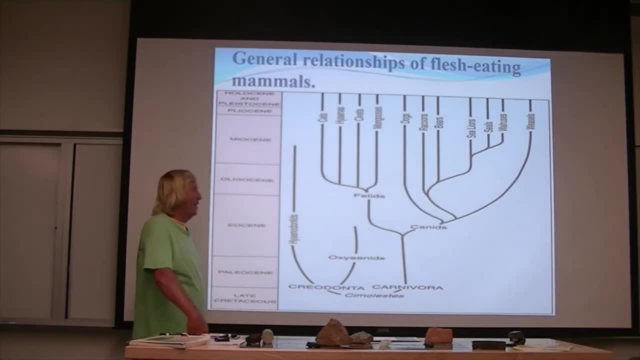 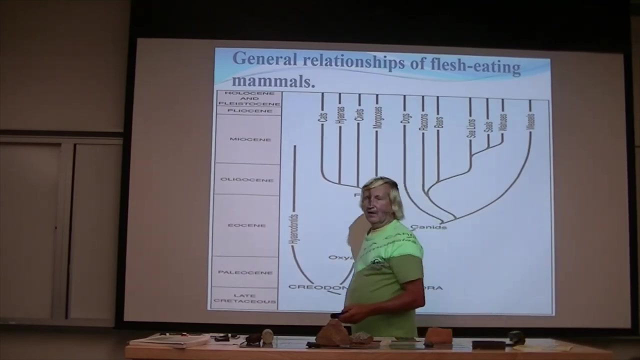 started melting, started warming about 16,000 years ago, and so the Holocene is named for Homo Sapiens. but what's interesting about this is we just have such a huge splitting of these species- and this splitting is being directly attributed to diverse climate- that these species 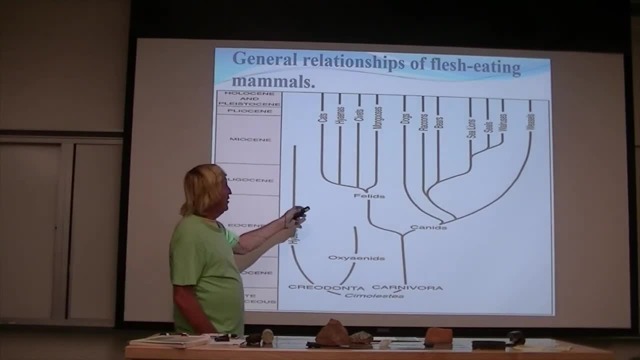 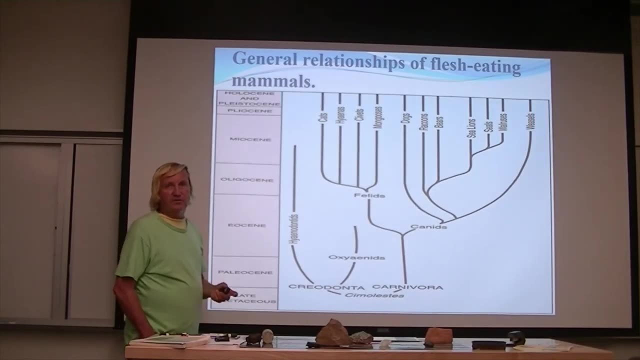 each adapted to environmental conditions and because there was such a diverse environmental conditions, so many different environments, that this led for these splits of many, many species. it's kind of like vascular plants and non-vascular plants, so the vascular plants have to have their roots right in water. 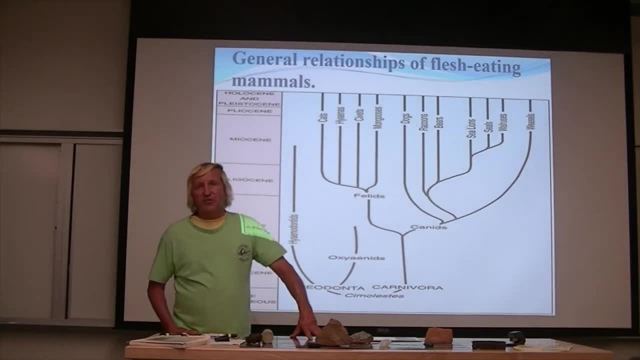 they're very limited where they can grow and when you see that a third of the earth is land and most of that land is not near the coast, this basically was an environmental condition for vascular plants to move on the land, and the same thing happened with the animals. 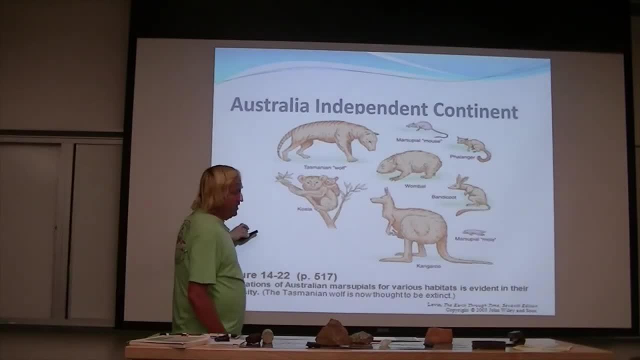 so Australia, this is that Wallace line. remember we talked about the Wallace line at the beginning of this semester where Wallace had basically draw a line that separated basically southern Indonesia and Australian species from Asia. so this 8 Australia, it basically was an independent continent and Bader kind of recognized. 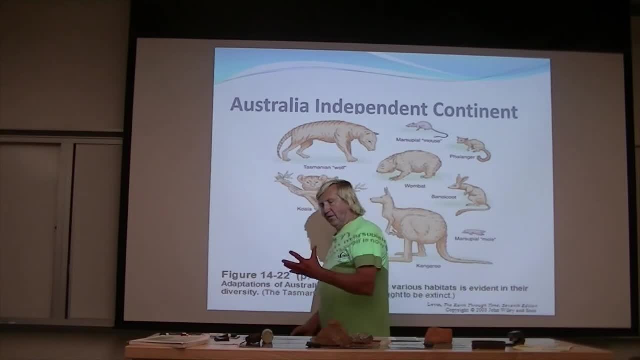 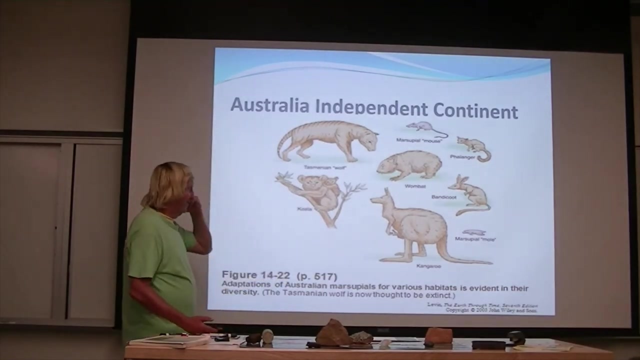 that continents are independent, but of all the continents that are probably the most independent with respect to species is Australia. as it turns out, Australia has the highest number of poisonous spiders, snakes and animals than any place in the world. they have actually a brown spider that is far more deadly. 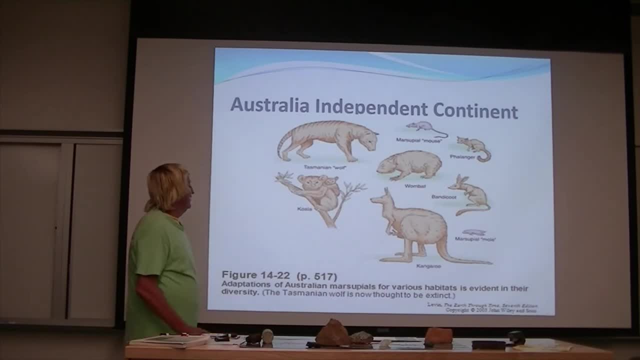 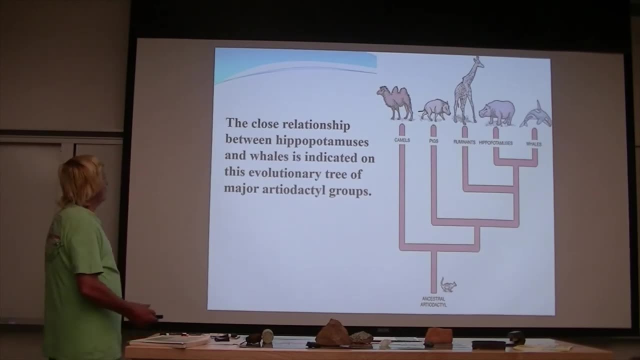 than the black whittle, and Australia has some very unique animals. okay, so the closest relationship between hippopotamuses and whales is indicated on the subluxated tree. so here we have the ancestral tetrapods, camels. we start from camels and then the pigs. 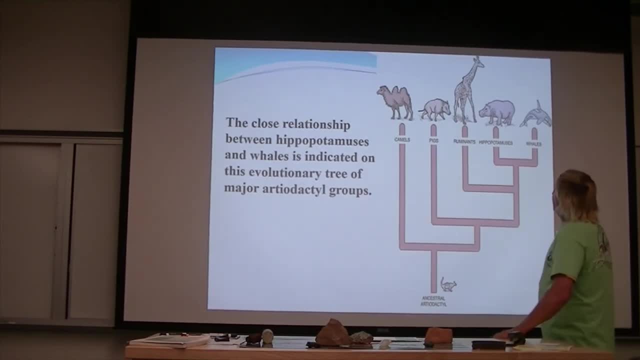 and then we go into hippos and whales. so what we think happened is that dogs go back to form whales, whales then come back out of the ocean to form hippos, and what's neat about this area is that within the last 20 years there have been so many discoveries. 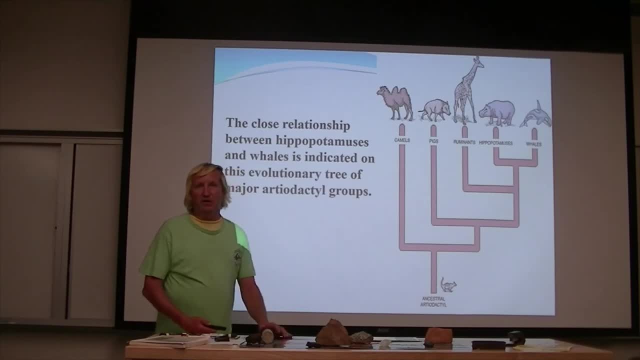 so the valley of the whales, that was a discovery in Morocco. so at that time what is today northern Africa, a desert, was actually a part of the Mediterranean Sea that had flooded that and whales would go in there and spawn, and so we have all these whales from a very long period of time. 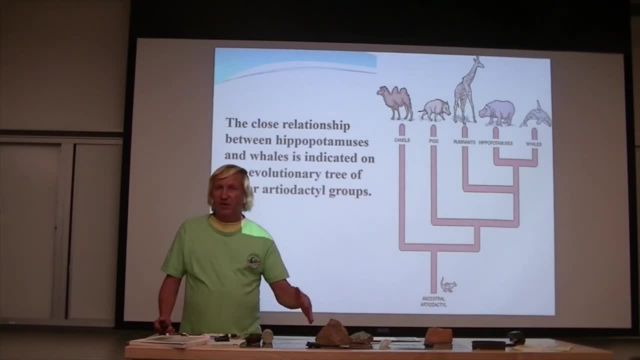 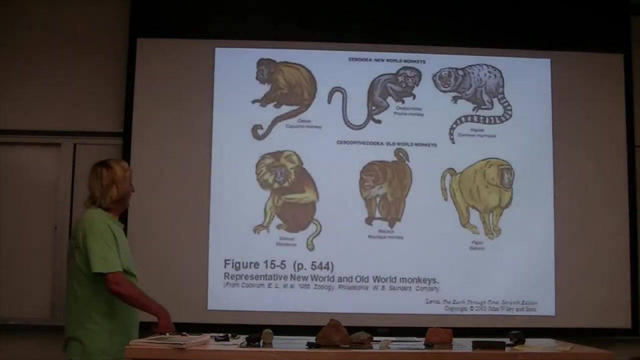 and we've been able to put together- paleontologists have been able to put together- a whole sequence of whales that show a transgression from a dog to a whale, and that's pretty powerful. then there's these guys here and then it starts to get into the little human evolution thing. 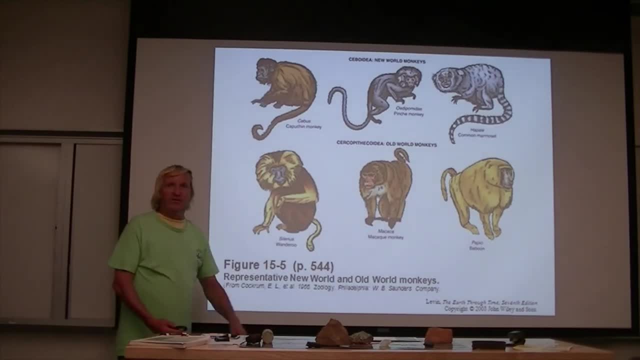 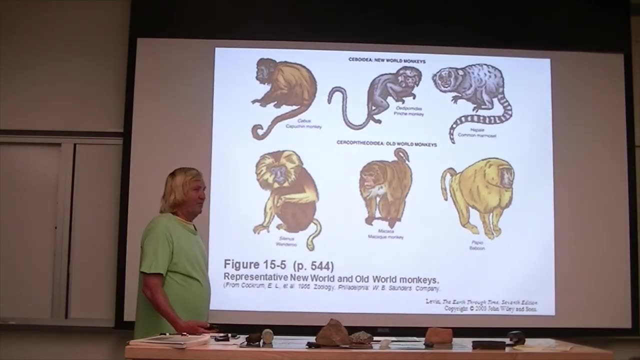 which I'm not going to go into. if you want to go deep into human evolution, you can take an anthropology class with that boy. that gets very people get very emotional about that when you talk about human evolution, when you talk about animals and plants, ah, okay, yeah. 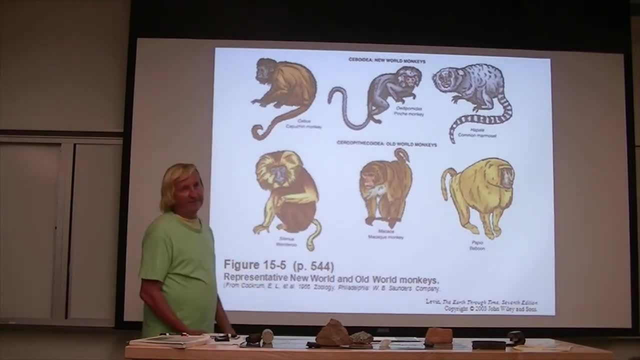 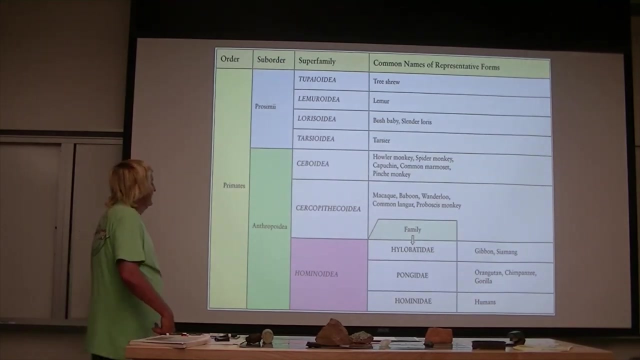 so where do humans come from? well, most anthropologists will tell you that humans, as we call humans, appeared on earth about 3 million years ago. we do have very close genetics to a chimpanzee- we're not too far off. so primates- and this gets to the anthropology. 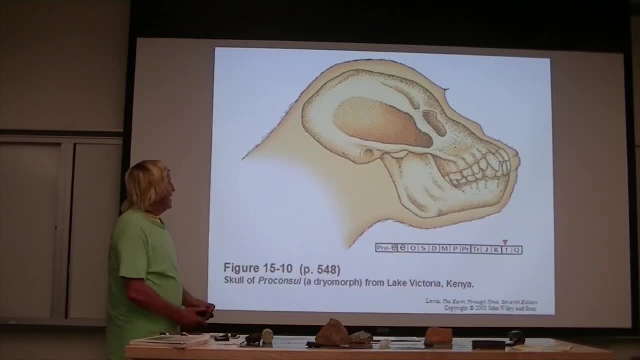 which I'm going to avoid. you know the evolution of the head, the brain, cranial capacity. that's the big thing as it turns out with humans. there are two species of humans. there are actually two lineages, one died off, and the whole thing in anthropology right now. 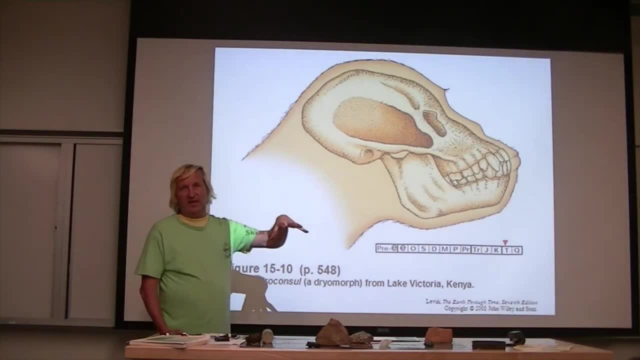 is cranial capacity. so the size of the head, size of brain, more brain cubic centimeters or not really a cubic centimeter to be able to be brain. but the larger the brain, the larger cranial capacity, the more advanced the species is thought to be. that's kind of the growing trend in anthropology right now. 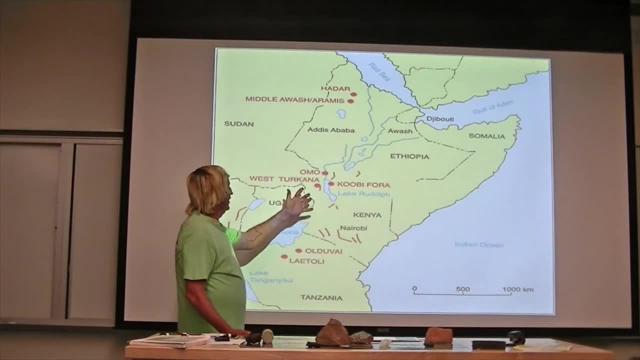 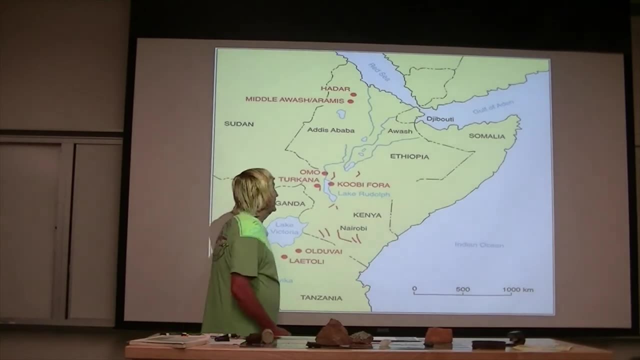 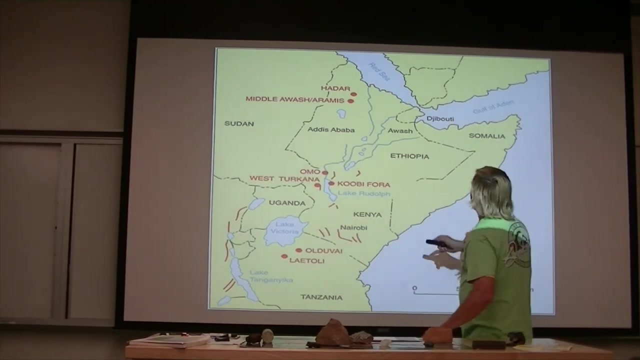 so what do the human whole thing start in Africa? ironically, right along a rift. so, basically, what's occurring here in this part of the world is that Saudi Arabia, the Arabian plate, is moving to the north and to the west, away from Africa. as it moves away, it opens up the Gulf of Aden. 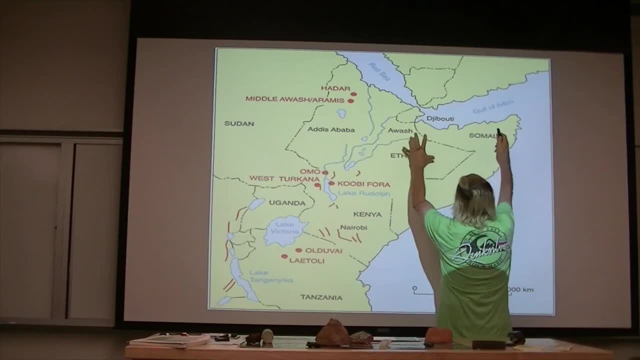 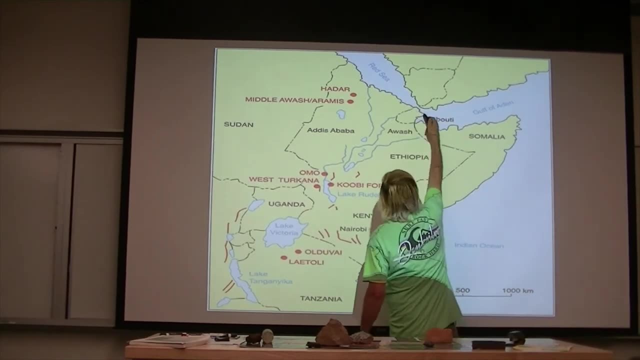 and the Red Sea. so at one time the Gulf of Aden and the Red Sea were closed in and these two continents were together, and so this is like a triple junction: one goes this way and this way and then one goes right through here and this is called the Olagai Gorge. 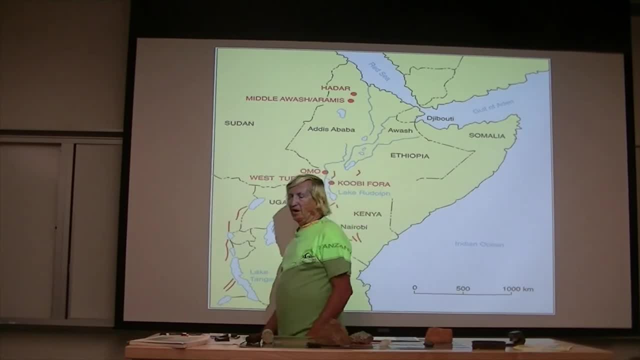 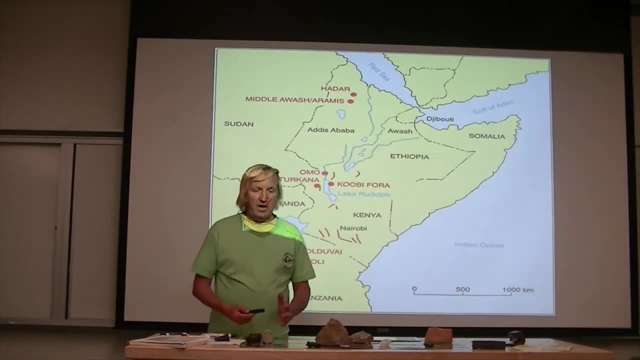 in Africa and this is where the earliest human remains have been found. is there a complete fossil record of humans? no, there's not. we don't have that transition. I know in popular talk we call it the missing link, right? it's really transition fossils. you're looking for a clear transition. 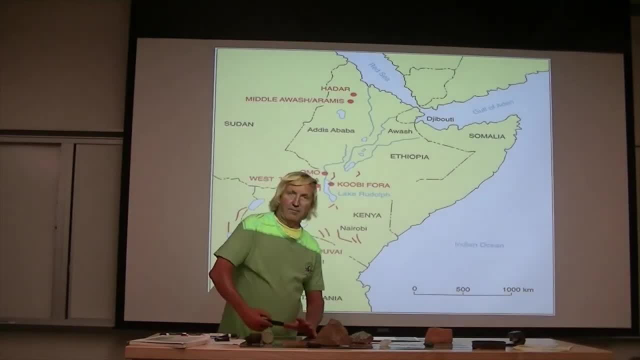 this brain, this head, this jaw, arm, whatever, and you like to see a sequence of events? we have that with tetrapods today, so we have devonian age fish that show a great transition from fish to land animals. we don't really have that in humans right now. 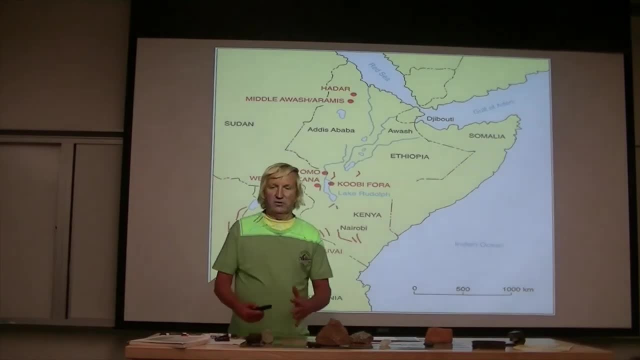 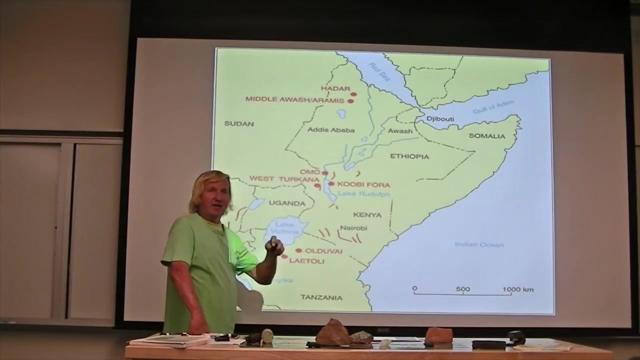 we don't have apes to humans. there's a lot of missing transition fossils in there. are they out there to be found? who knows? as time goes on they might make new discoveries and, like I said, that's for the anthropologists to go with. so the big thing in anthropology. 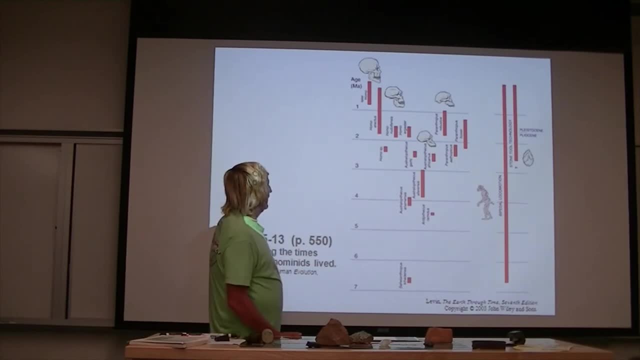 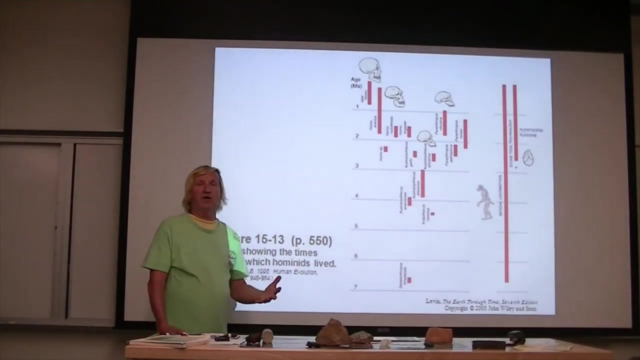 is: what do you call a chimp? what do you call an ape? what do you call a human? is there a transition? and right now, there isn't. there definitely is an evolution of human species. humans have evolved. our brains have evolved: our jaws, our heads, our eyebrows, our skulls. 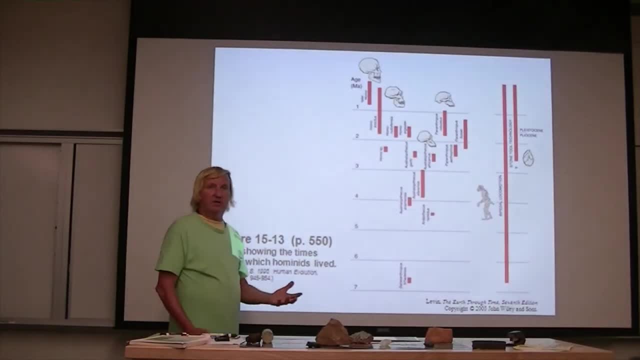 we have a larger cranial capacity today, larger brain size than previous men or man like and women did have. but the transition from ape to what we call today a human, those transition fossils aren't there or they haven't been discovered yet. so certainly these are a comparison of skulls. 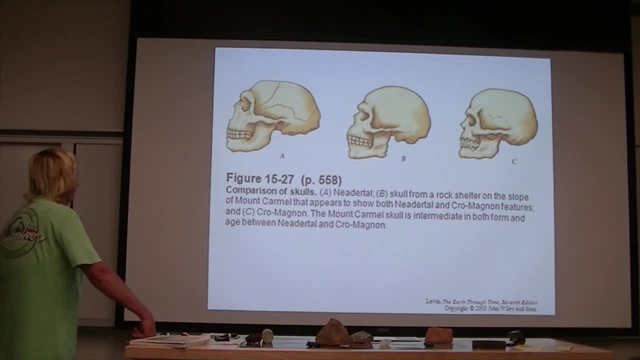 so here's a Neanderthal, the skull from a rock shelter on the slope of Mount Carmel. both shows Neanderthal and co-magnon features, and then see co-magnon. Mount Carmel skull is intermediate, in both form and age, between Neanderthal and co-magnon. 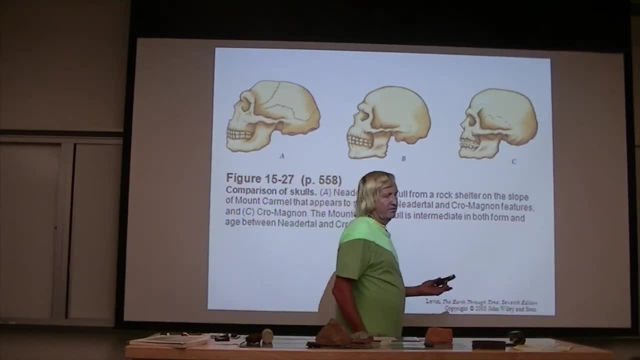 so this basically shows a transition. so humans have had evolution. now, when you talk to religious scholars, they'll completely dispute this. and then there's some anthropologists that believe that there were two different human lines, that this one went extinct and this one is the one that's living today. 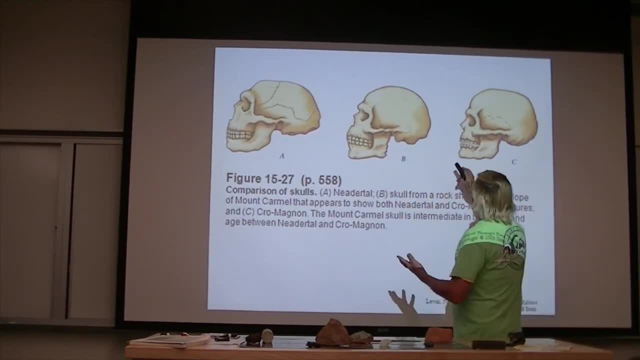 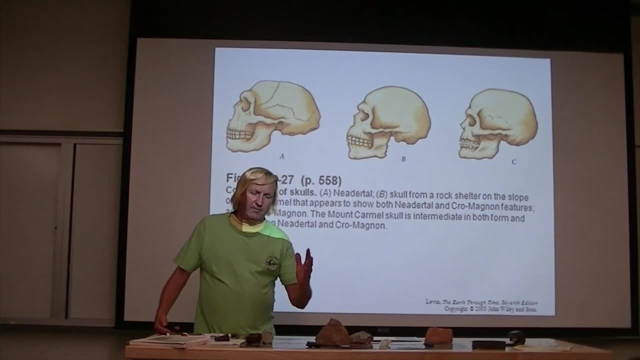 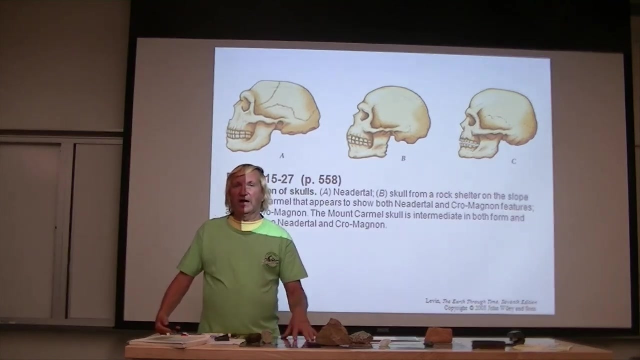 but even though if you look at B and C, you can see that there is some evolution that's occurred. I mean, we have evolved as humans think about it. blonde people are from the northern latitudes. they are better adapted with blue eyes to see in white conditions. 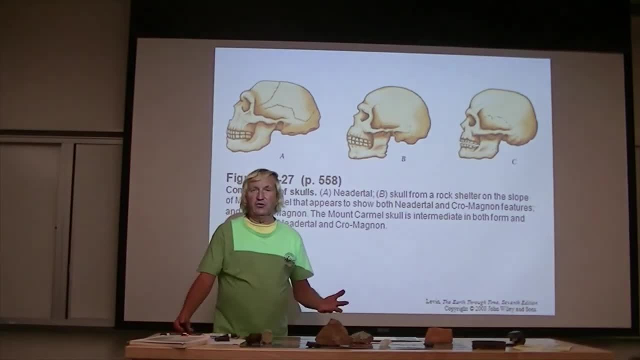 dark skinned people have an adaptation in their skin pigment where they develop more melon, making their skin darker. that's an adaptation for more sunlight. so humans have evolved and the difference between a dark skinned person and a light skinned person is simply this evolution. 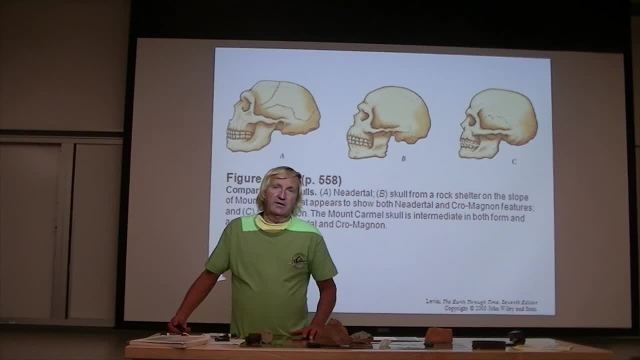 a little bit of pigment melon to make skin darker or lighter. skin is just a lack of so. humans have evolved adaptation, natural selection, through environmental pressures. so people who live in northern hemispheres tend to have light colored eyes and it shows that blue eyed people 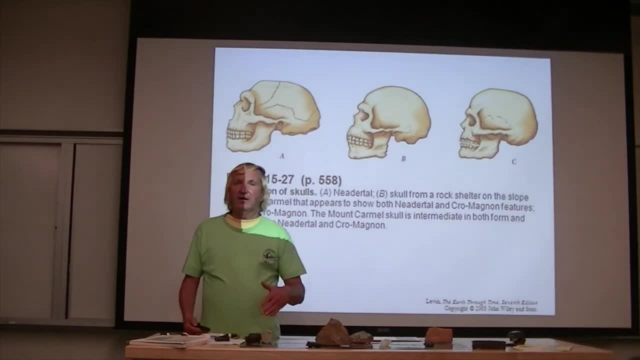 blue eyed to green are better adapted and seen in white conditions where there's lots of snow. people who have darker eyes are better adapted for. they have a better adaptation for warmer environments and deserts. so humans have evolved. is there a transition all the way back to apes? 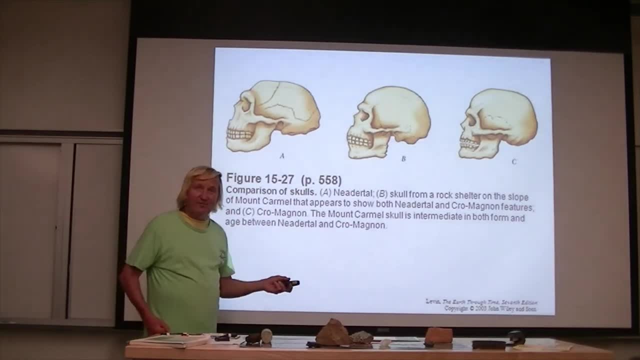 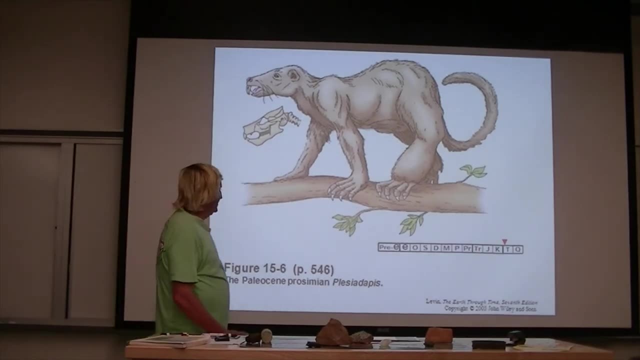 no doesn't mean it's not there. that's for the endopolis. so, as it turns out, what makes us uniquely different from all the primates is, right here, our thumb. this is probably the most important advancement that humans have is the thumb. thumbs allow us to grasp. 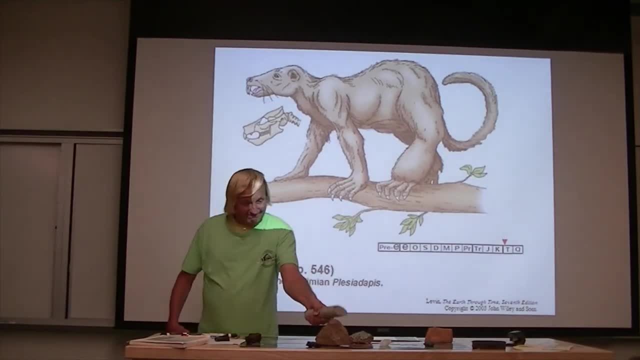 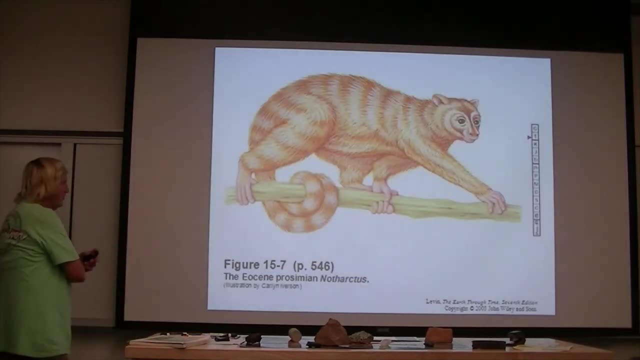 when I try to pick something up without a thumb it's a little harder with a thumb. I can really grasp, really grasp on the thing with the thumb. so thumbs have been important. you know tails, we have a tailbone. it's completely useless, we don't need it for anything. 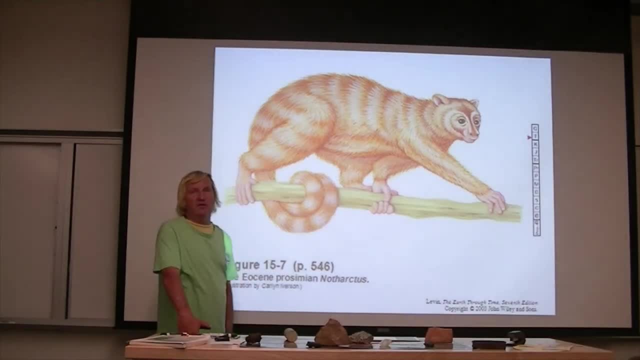 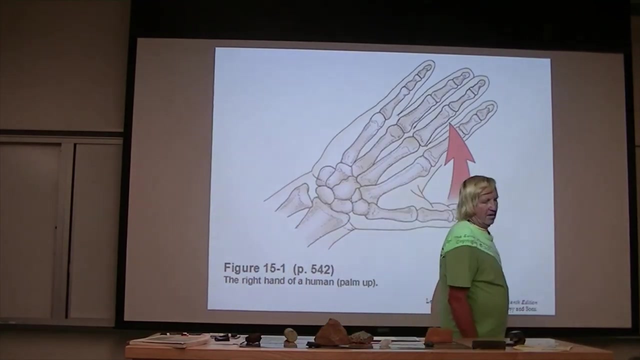 I've heard they say it's the most painful thing you can go through and there's no way they can heal it. what are they going to do? wrap your whole bottom half in a cask? that'd be difficult. so the thumb- really important aspect of the hand. 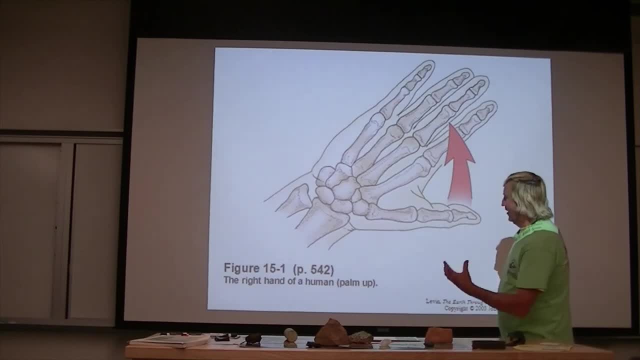 it allows us to grip, and when humans developed that thumb, that made us the most adaptive species on earth, because we then can make tools and change the earth. and that's exactly what we were doing, and you can blame it all on the thumb. so I never really thought about that until 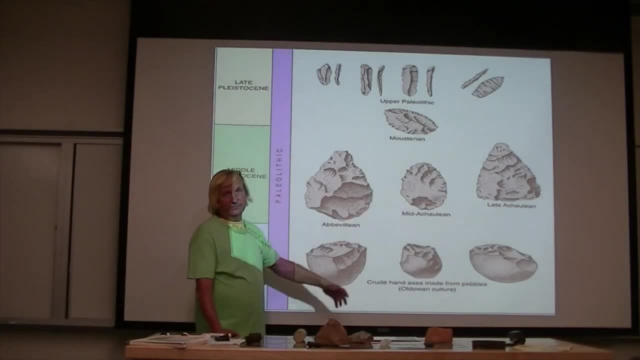 now on the thumb. so because of that, we make tools. our first tools were crude, out of stone- obsidian. but when you have the thumb you can make tools. it's hard to make a tool without a thumb, I mean if you're sitting there trying to. 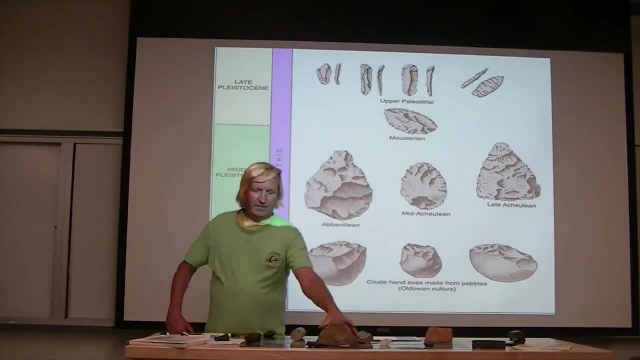 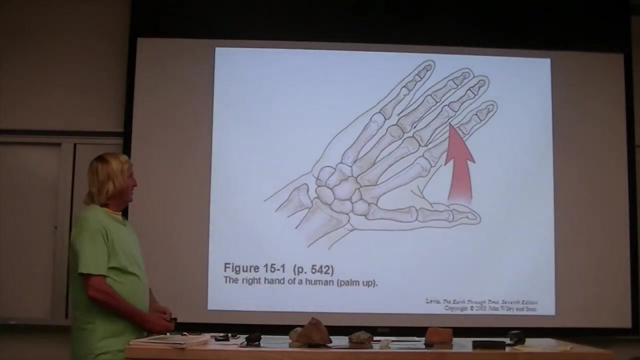 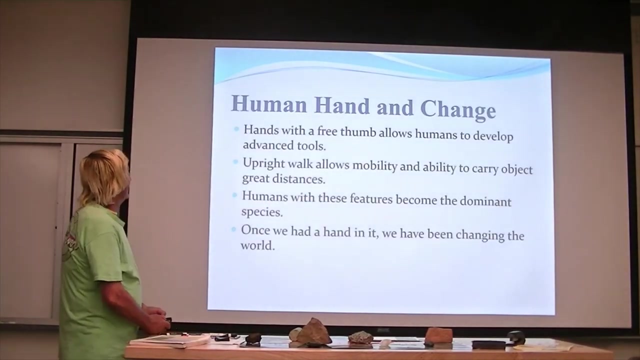 you know, you just grasp. you know, if you have a knife for a rock, you can, you know, grab with your thumb. and so the thumb, very important adaptation. it allows us to change the world and we've been changing the world. so the human hand in change hands with a free thumb, allows humans to. 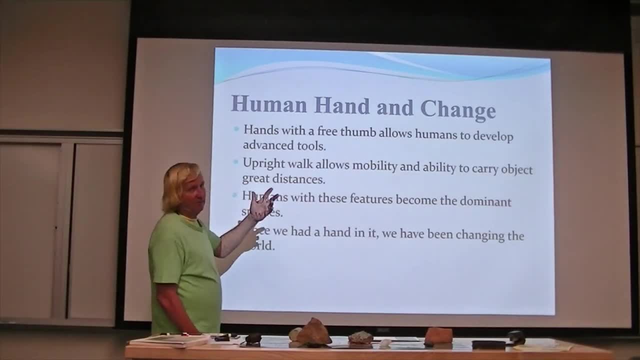 develop advanced tools. upright walk- this is really important- allows mobility to carry objects for great distances. so if you're hunched over it's hard to carry things, but if you're standing up straight you can carry a lot here with your load. humans, with this feature, became the most dominant species. 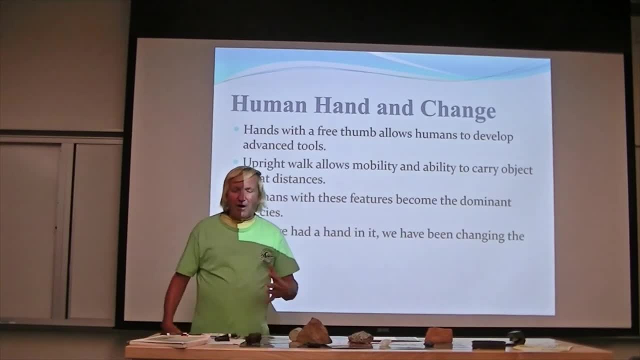 and we really became the most dominant species right around the end of the Wisconsin glaciation about 12,000 years ago. this is when humans radiated out. so humans appeared on earth 3 million years ago and they really don't do a whole lot until. 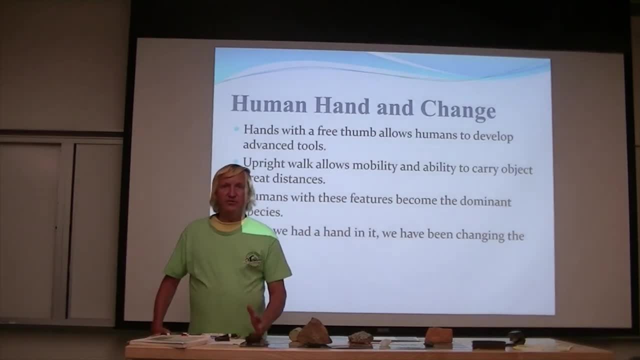 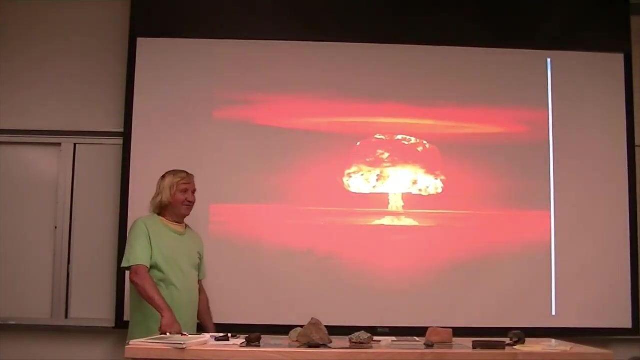 they transform. and then this is when, 12,000 years ago, during the Holocene, when humans really become the most dominant species on earth, and with our thumb we've had a hand in changing the world ever since, and we're continuing to change the world, for good or bad. 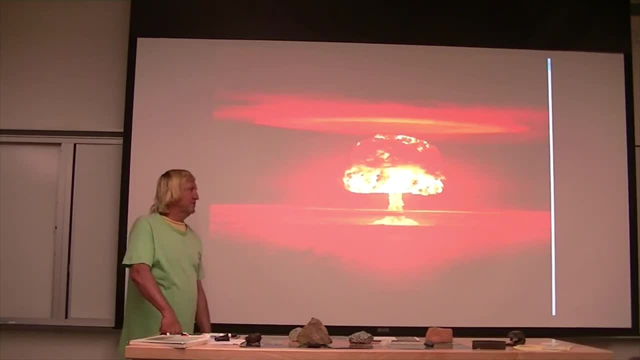 you know that's debatable and that kind of concludes the PowerPoints presentations for this semester. so after this, your focus is just to focus on the and then take a photograph. when you take a photograph, if the paper's down like this, put it on a table.